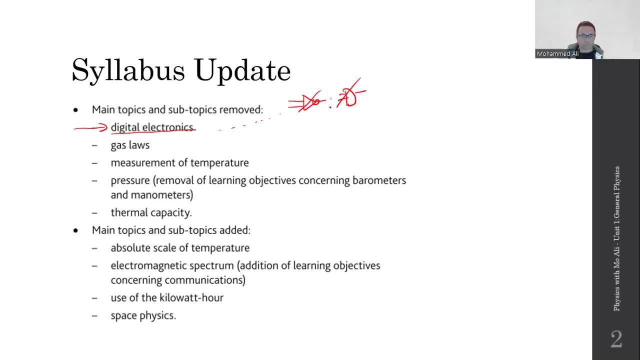 have probably seen these. These have been removed from the syllabus right. However, the mention of digital and analog as information systems has not been completely removed. It's actually been shifted to waves when it comes to communication and such. So we're going to study. 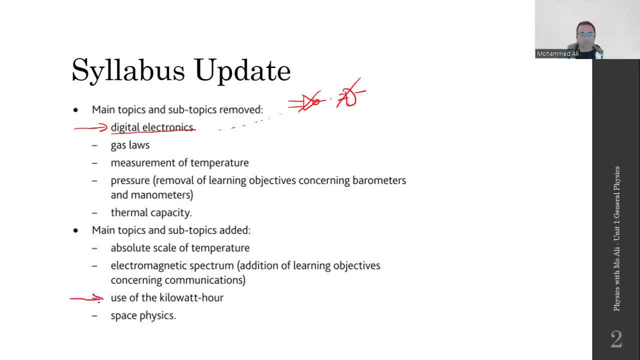 them later. Additionally, a new unit of energy was added called the kilowatt hour, And we're going to study that. So it's a very simple thing. It's what we use to measure electrical energy consumed at home, But that's another story. So, when it comes to electricity, these are the topics that have been. 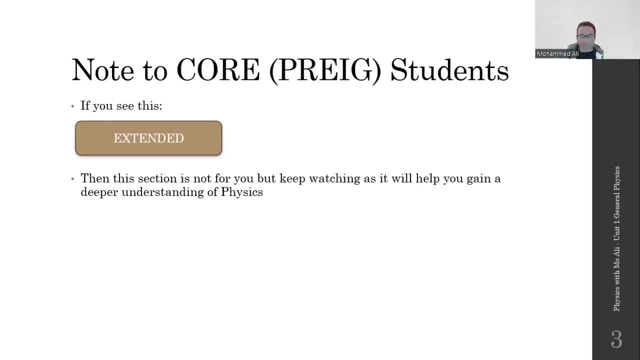 changed. A note to core students of course, or pre-IGCSE or year nine students: if you see the term extended on a page, know that this is not for you. However, it's very useful if you watch that section and try to understand it, because it'll help round out your understanding of the topic. 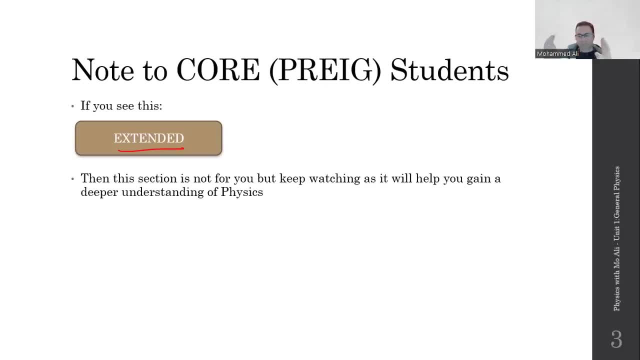 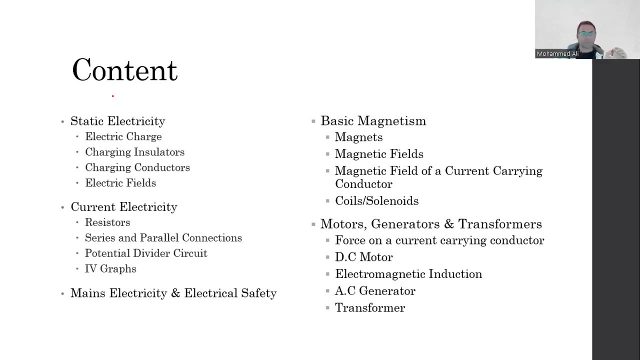 And unlike unit one, for example, where there was an entire chapter that you didn't need to study, Here there are just minor rules that have been skipped for your sake, But listen to them Nonetheless. they will definitely help. So what are we studying today? We're studying electricity and magnetism. So we're 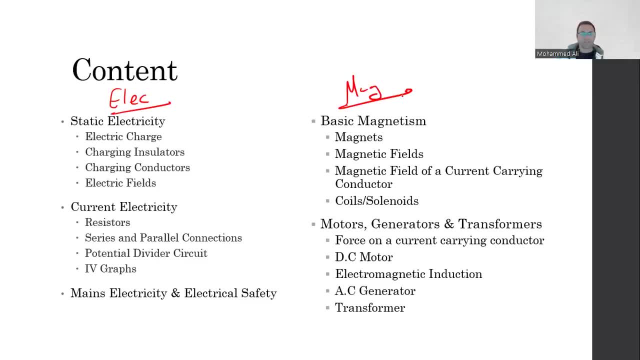 splitting them up into electricity and magnetism. From the electricity point of view, we have static electricity. So what's a charge? positive, negative, attraction, repulsion, charging, electric fields, basic stuff won't take long. The important part of electricity would be current electricity, So circuits. So what is a circuit? 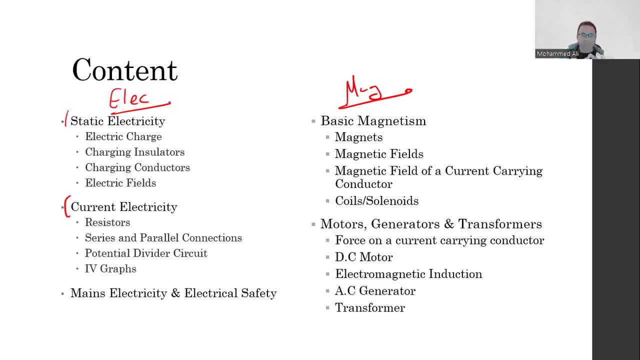 What's voltage? What's current? What's resistance? What are resistors? How do you connect them in series and parallel? What are potential dividers? Like different types of stuff, And we finalize electricity by talking about electrical safety features that we have at home, like the fuse. 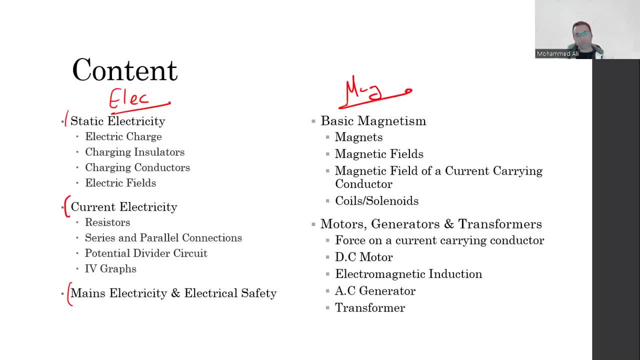 the circuit breaker and earth wires, And why do we need these features? Next, let's talk about magnetism. Magnetism: We're going to split them into two major parts, although the second major part is split into three. The basics of magnetism, as in: what's a magnet, what's a magnetic field and how. 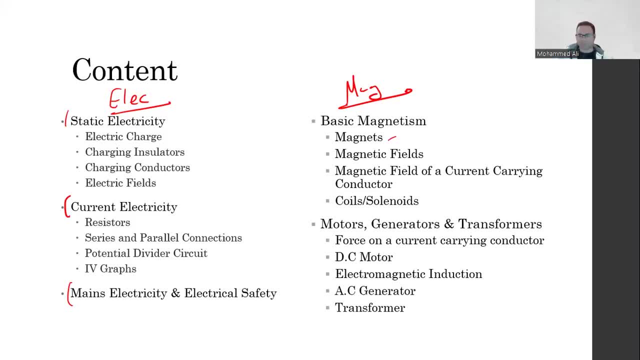 an electric current can produce a magnetic field. So you have electromagnets and coils and their applications, And then we have different electromagnetic applications, specifically three things: the motor, the generator and the transformer. So we're going to find three distinct sections when it comes to magnetism And then we're going to split them into two major parts. 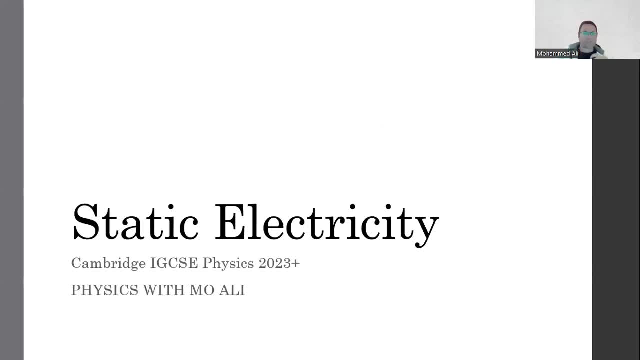 magnetism and electricity together. Let's get started with static electricity. The word static, if anybody doesn't know, means not moving. So when we're talking about static electricity we mean this electricity is not moving. So it's not a circuit per se. There's no flowing charges. 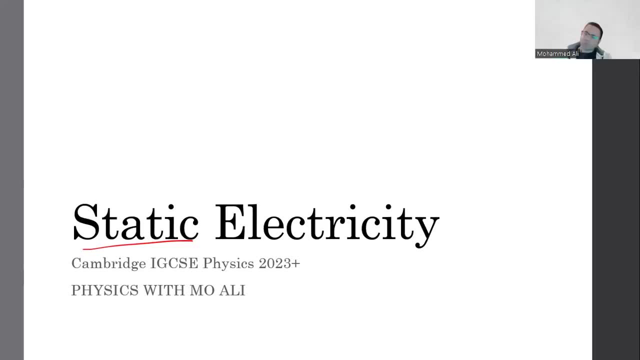 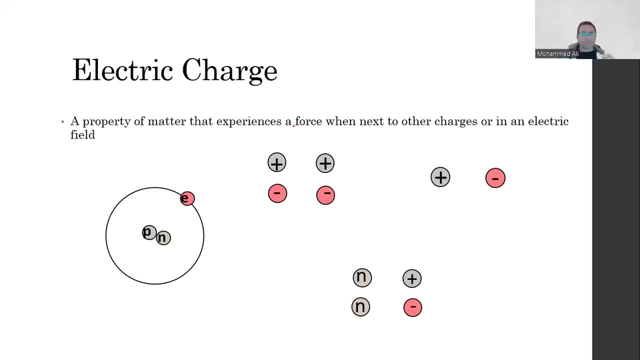 and so on, Although charges will move, but they will mostly move in order to stick from one object to the next and make something either positively or negatively charged. So, speaking of charge, what is charge? A charge is defined as a property of matter that experiences a force when next to 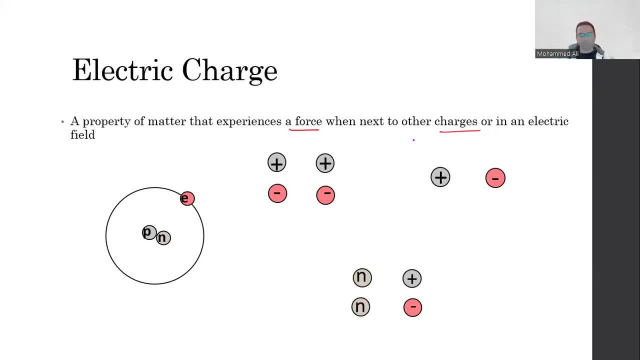 other charges or in an electric field. What do I even mean by that? If you take a look at an atom, inside an atom there are protons and neutrons and electrons. These are the three subatomic particles in an atom. A proton is positively charged, An electron is negatively charged. 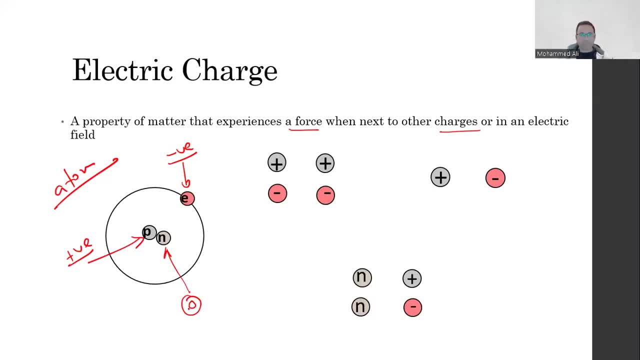 whereas a neutron is neutral. Charge is something that all matter has. Everything has charge Everything. Everything is either positive or negative, And that's because everything is made up of protons and electrons. Neutrons are charged or neutral. I'm sorry, even though they should be charged because they have both positive and 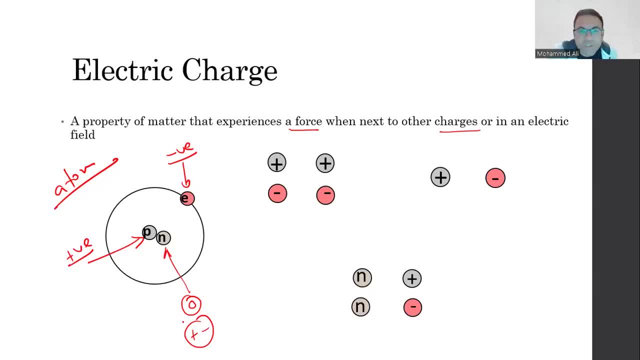 negative charges inside them. So if something is neutral, it doesn't mean it literally has no charges. It simply means it has both positive and negative charges in equal amounts. They're equal. Their resultant is zero. Basic concepts: positive and positive, repel negative and negative. 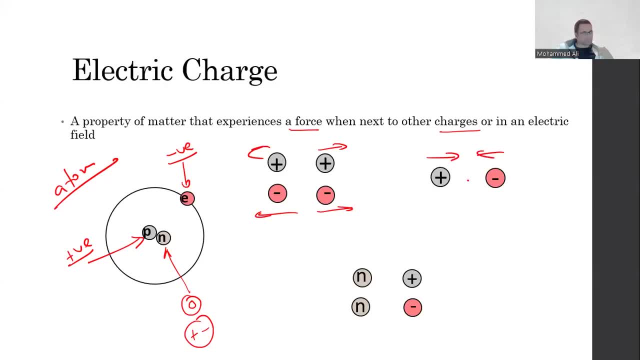 repel positive and negative attract, Like poles or charges. repel opposites attract. But neutral objects are also attracted to charged objects. So if something is positive or negative, it's also attracted to things that are neutral, Like we agreed, because they have both positive. 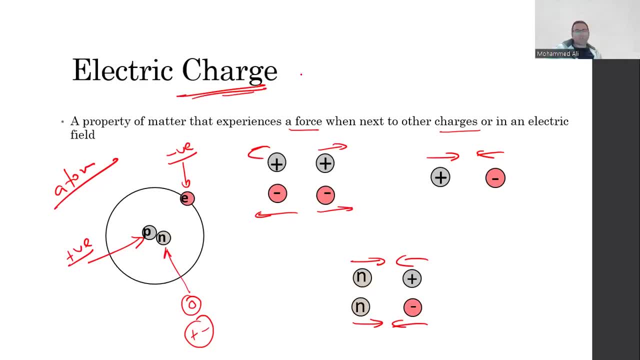 and negative charges. Now, charge as a quantity has a unit of measurement. This unit of measurement is called coulomb. So a proton has a certain amount of charge in coulomb, certain amount of charge in coulombs for the negative, and so on. Good, Now when it comes to charging objects or like a charge, 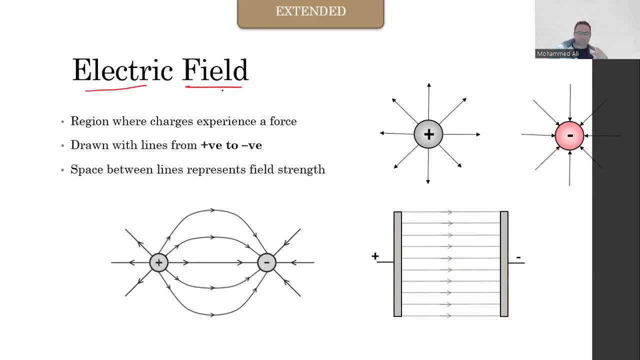 itself. it has a region around it called an electric field. We'll talk about charging objects after this. What's a field? It's a region where charges experience a force. So, for example, here I have a positively charged ball If I put a positive charge here. 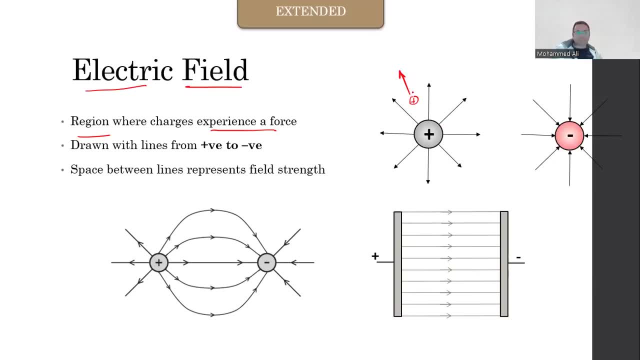 it'll get repelled, which means it'll experience a force. So we show this force by drawing lines. These lines are always drawn coming out of a positively charged object or into a negatively charged object. Why? Because the direction of this arrow, of this, 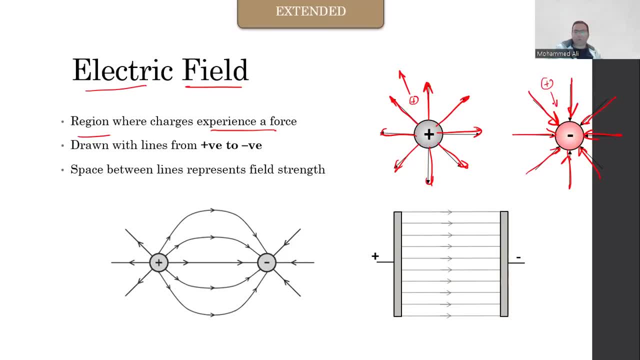 line of these lines shows me the direction on a positive particle. It shows me the direction of the force on a positive particle. Now you might be thinking: what about the negative? What will that do If you have a negative charge? it'll just move opposite to the direction. 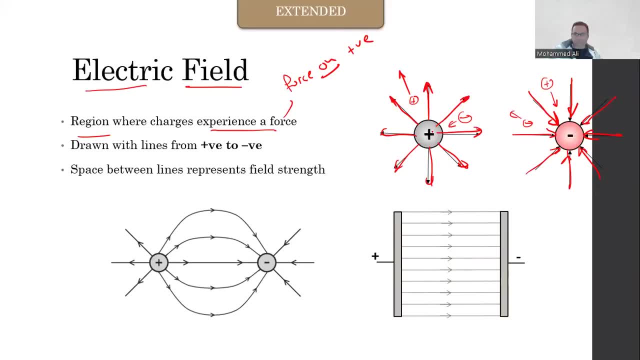 of the electric field lines, Because negative and positive attract, so it'll move towards the positive. Negative and negative repel, it'll move away from the negative. Now one more feature. The space between the lines represents how strong the field is. The closer 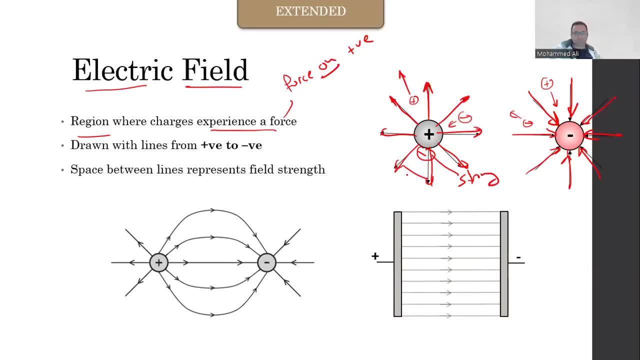 the lines are to each other, the stronger the field is, And the farther away the lines are from each other, the weaker the field is. Okay, good, If you put a positively charged object next to a negatively charged object, their fields will join together to form a 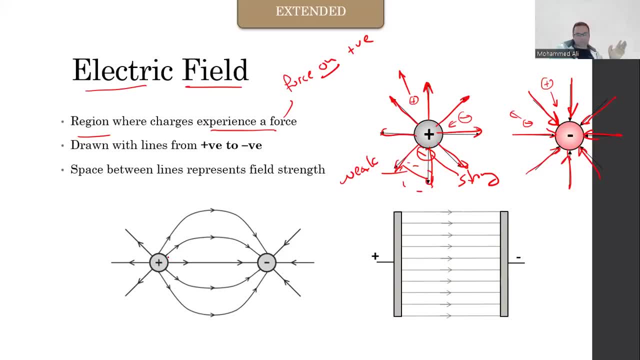 combined field. If you have two spheres, the field will look like this: Yes, from positive to negative, and the field strength changes, Being strong here, weak here and strong here. But if you have two flat plates, one is positive, one is negative- 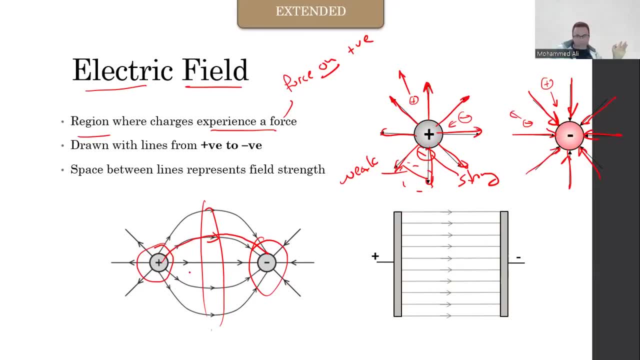 the field lines will move from positive to negative, just like usual, from positive to negative. But because the surfaces are flat, the spaces between the field lines are constant. They don't change, they're equal. And if the spaces between the field lines are different, you're in the wrong place. 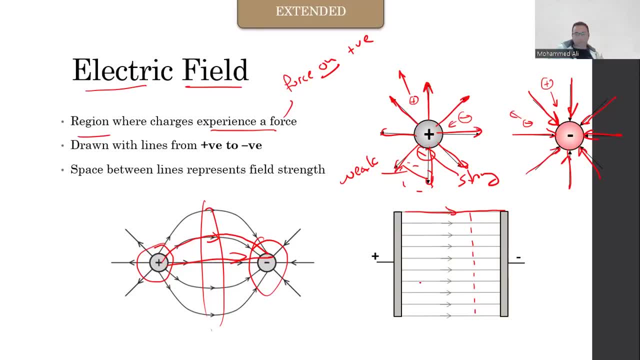 for already in the whole path. It's a menu, correct. It's the exact answer, correct. Let's lines are constant or equal, they don't change. we call this a uniform field, the word uniform meaning meaning constant. so the field strength is also constant, okay. 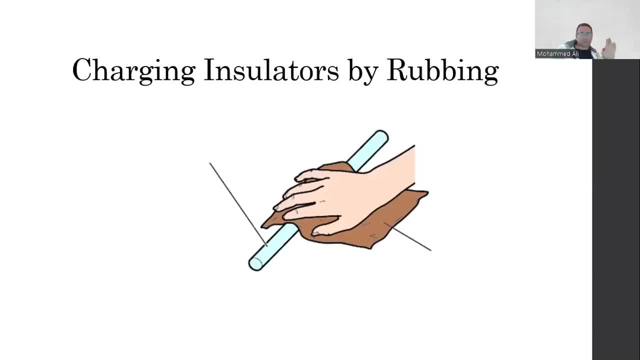 so, going back to core stuff for a bit, you can charge an insulator by rubbing it with another insulator. so if you have a cloth, a cotton cloth for example, and a glass rod or a plastic rod and you rub them together, the friction between them causes one of the objects to lose electrons. 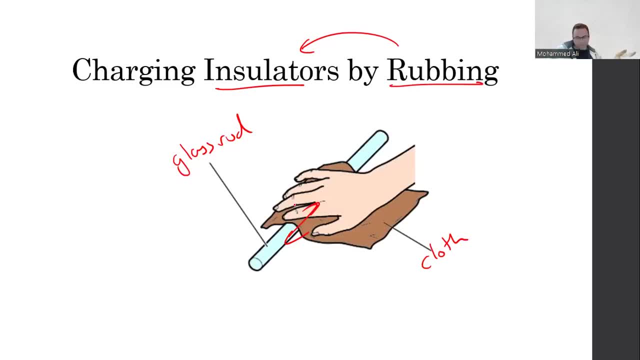 and the other gains electrons. so by rubbing them, the cloth loses electrons and it's gained by the rod, for example, which means that if you separate them, the rod becomes negatively charged because it has gained electrons, whereas the cloth becomes positively charged because it has lost electrons. so the only way of charging something is by either having that. 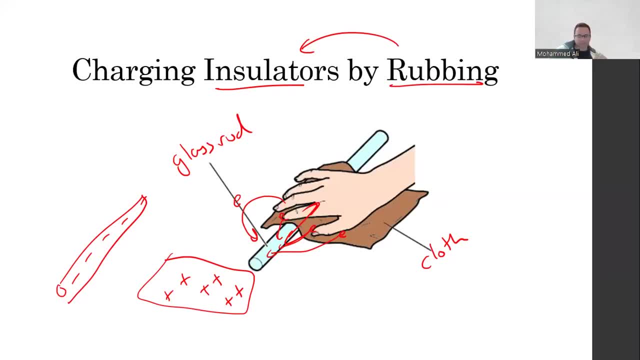 something. lose or gain electrons. lose or gain electrons. now, which one is losing, which one is gaining? i genuinely don't know. it depends on the materials. but if the question tells you that, hey, electrons have moved from one object to the other, then that's your clue, that's your key. 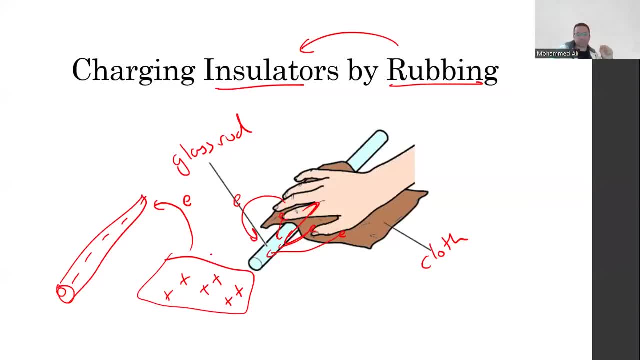 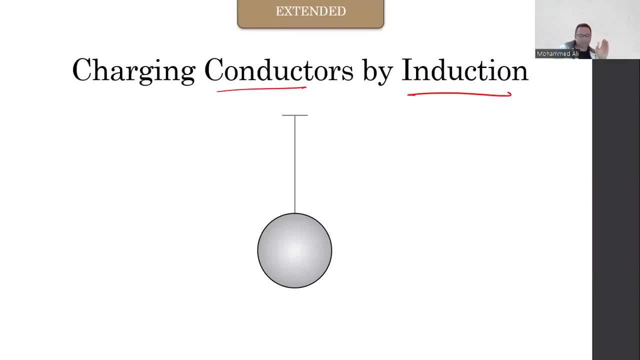 whatever gains electrons is negative. whatever loses electrons is positive. yeah, you can also charge a conductor by induction. but let me preface this by saying something in the curriculum, in the document, there's no mention of induction directly, but there is a mention of understanding how things are charged when the electrons move. so i'm keeping this in. 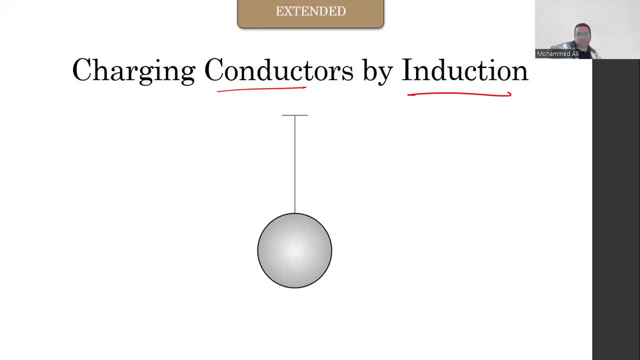 here. all right. so charging a metal by induction is not mentioned in the curriculum document directly, as is but a mention of charging a substance by adding or removal of electrons is mentioned, so i'll just keep it as is. if you have a metal, ball metals are good conductors of electricity. why? because they have free moving. 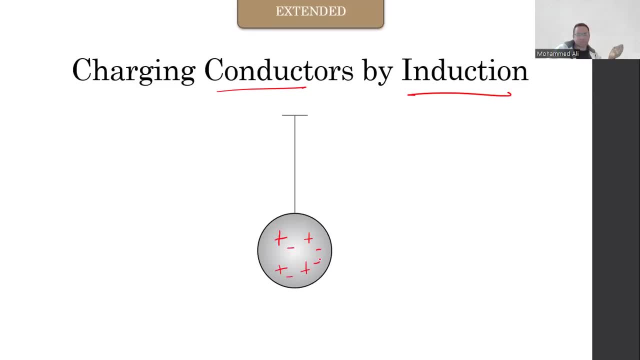 electrons. so not only do they have, you know, positive and negative charges in their atoms, they also have free moving electrons. so they have free moving electrons, so they have free moving ones, so they don't get charged, they also don't get demanded as a function of the ook guys. look at the. 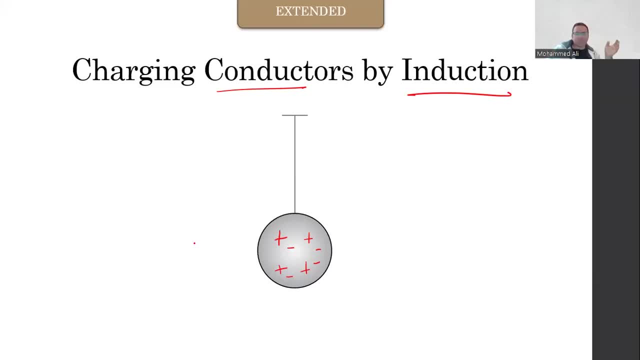 已经. plants are almost 味 nd term any or a or e t e in. on. Now that's cool and all no problem at all. but what's going to happen inside is this: This left side becomes positively charged and the right side becomes negatively charged. 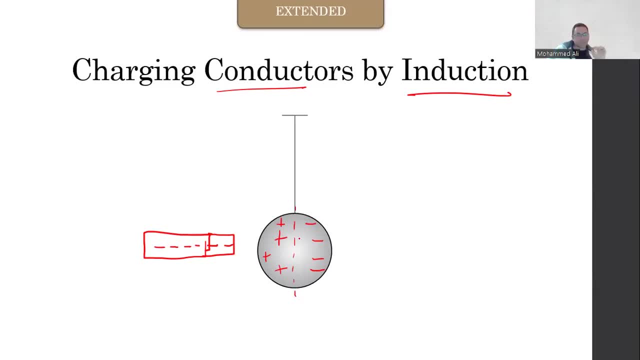 So the distribution of charges changes. Now the ball is still neutral. by the way, Right now it is still neutral. Number of positive charges equals number of negative charges. But if you connect this ball to what we call an earth wire or a ground wire or just any other conductor, 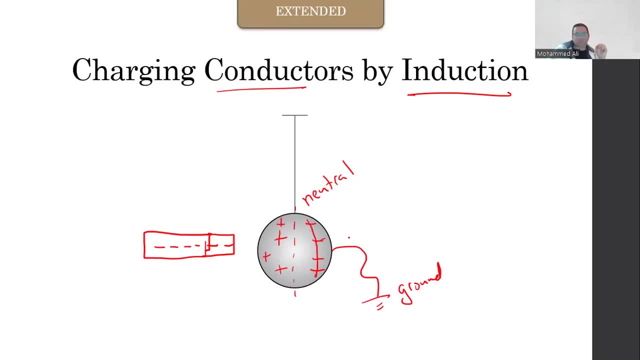 these electrons are going to get repelled out of the metal sphere. So the metal sphere now becomes positively charged. What we then do is we remove this ground wire. If you remove the ground wire, there is no way for these electrons to go back. 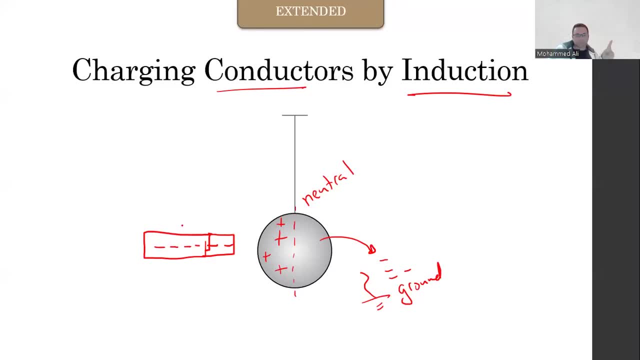 So now the sphere is positively charged. So here are the steps: You bring close a negatively charged rod- or positive, doesn't really matter much- And then you connect this metal sphere with an earth or a ground wire And then you remove the wire or the conductor before removing. 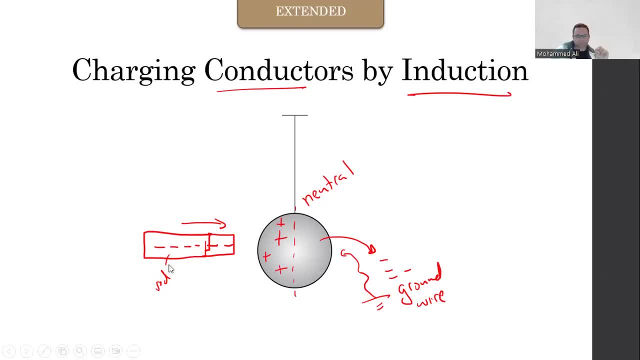 This will charge your metal conductor. If you want to give the metal ball a positive charge, you use a negative rod. If you want to give the metal ball a negative charge, you use a positive rod. It always charges the opposite charge And that's static electricity. 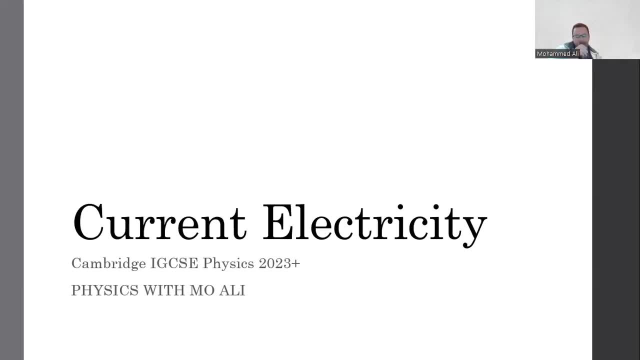 Very short, very succinct and honestly, not very- I don't want to say- important. It doesn't really show up in a lot of questions: Current electricity: Now take a deep breath, because I know I do need to take a deep breath. 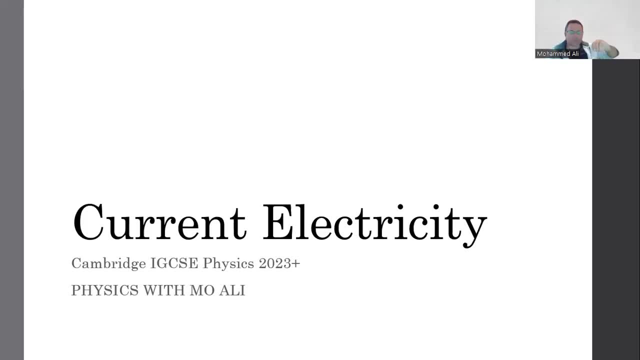 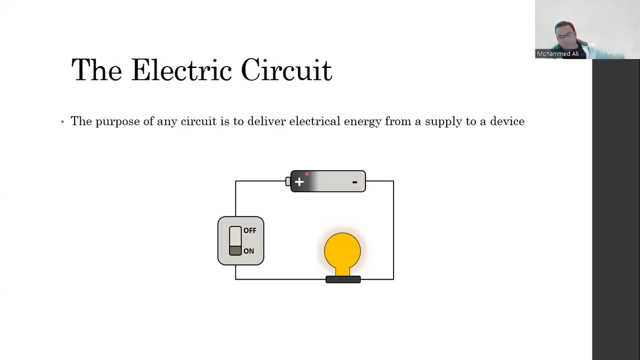 We're going to start current electricity. This is very important. Almost all of electricity relies on you understanding the difference between voltage and current and resistance Before we start. short story: If you have a circuit, it's the purpose of the circuit. 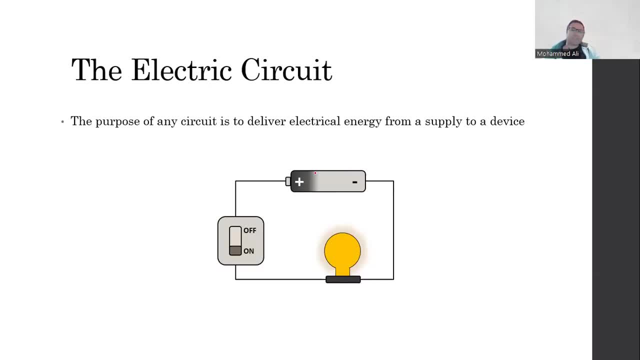 The purpose of this circuit that's in front of you right now is to deliver energy from a source of power like this battery to a device that needs the energy, like the bulb. The way we do this is by connecting this electrical source of energy. 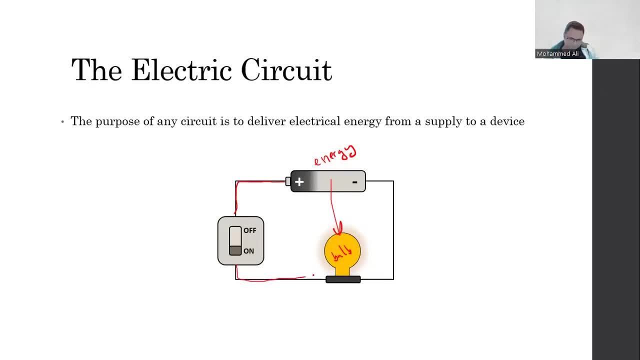 using metal wires- Copper wires are the best- So that you have a circuit, a loop, Once you close your switch. and when I say close the switch, I mean the circuit's going to be on. If I tell you we open the switch, the circuit's going to be off. 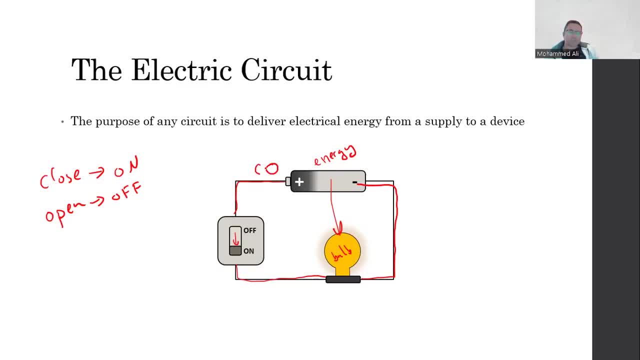 So once you close the switch, charges, positive charges leave the positive side of the battery and each one of these charges carries with it- Oops, I don't know why I did do that- Carries with it electrical energy. So every one of these charges carries with it some energy. 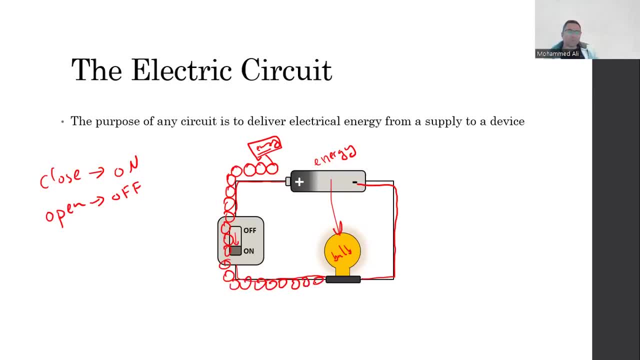 These charges move, move, move, move and move through the circuit. The reason they're moving is because the battery's giving them a push. So the battery's responsible for the pushing. It's applying a force on them to push the charges through. 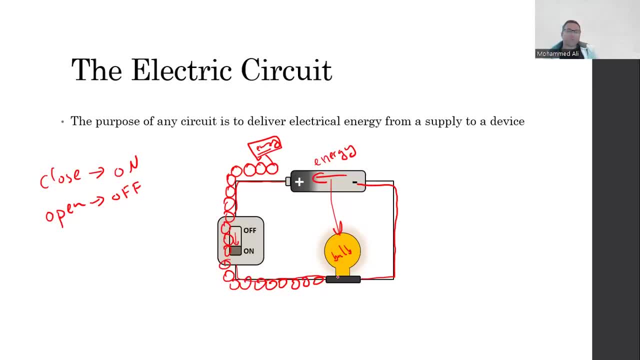 Once the charges reach the light bulb. the light bulb has a property that we call resistance. It tries to slow down the charges. So as the charges go through the light bulb, they lose their energy- Something similar to friction, And as friction produces heat. 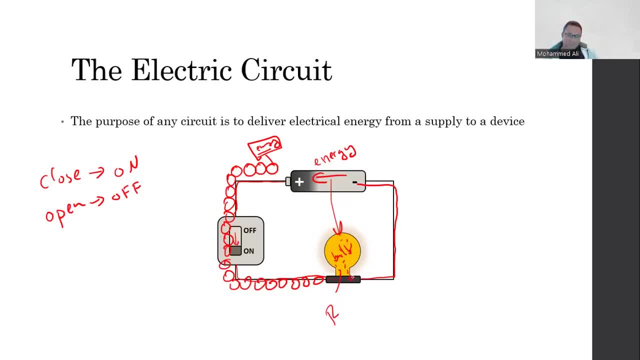 the friction- and forgive me, friction- between the charges and the light bulb itself releases electrical energy into the light bulb, So the light bulb lights up. These charges then get pushed back or pulled back to the battery. They gain some more energy, They're pushed out and you have a circuit. 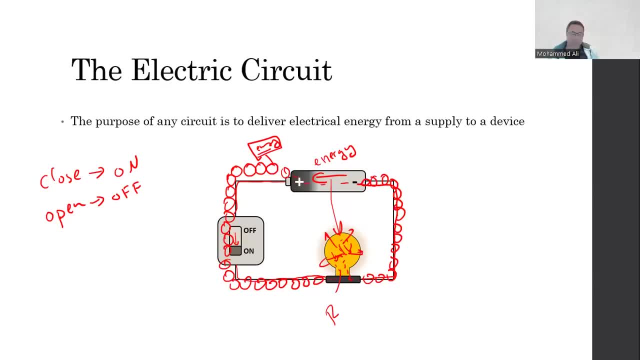 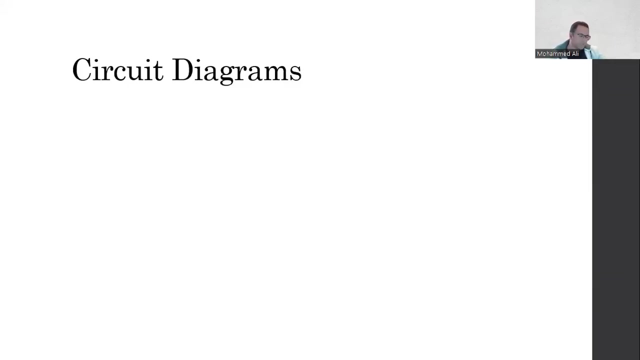 So the purpose of a circuit is to deliver energy from the battery, the source of energy, to a device that needs it, But we need a full loop, a closed loop, a circuit, All right. Next, We're not going to be drawing circuits like that though. 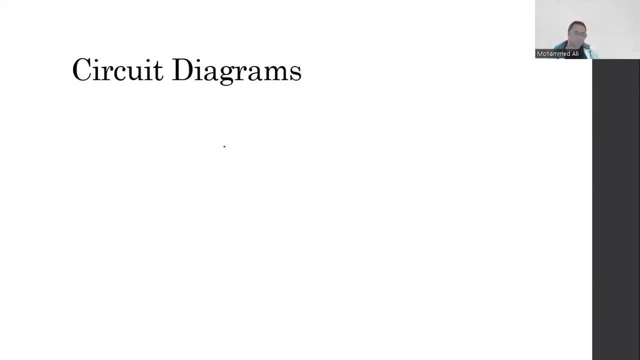 We're often going to use circuit symbols, So here are the symbols. This is the symbol for a battery. This is a symbol. This is a symbol for a switch. This is the symbol for a light bulb. That's all there is to it. 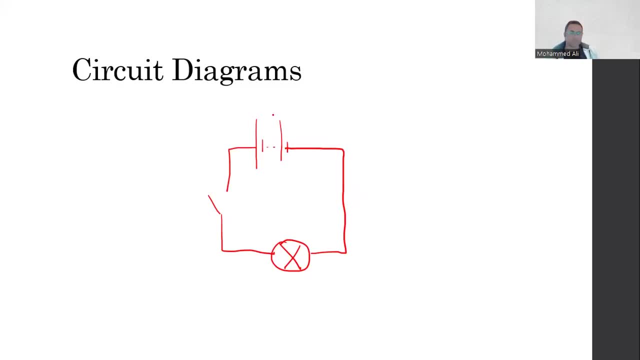 So battery switch, light bulb. The long line of the battery is the positive charge, The short line is the negative charge. Here's a light bulb. You want to call it a light bulb, a lamp. The switch is always drawn open. 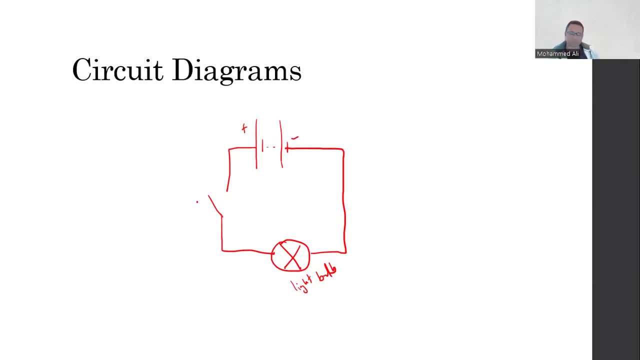 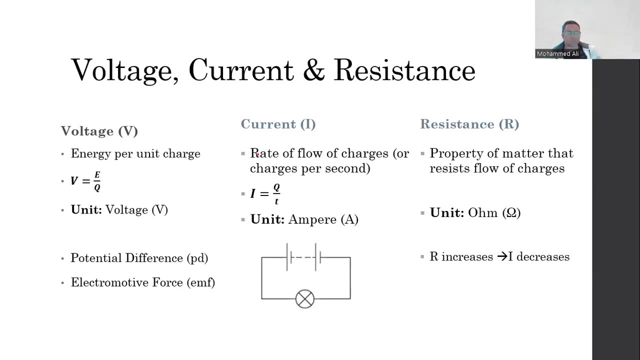 I don't care what the orientation of the switch is, It's just always drawn open. Next, Now let's define our three most important quantities when it comes to electricity: Voltage, which is V. Current, which is I. Now, the reason it's called I is because the full term 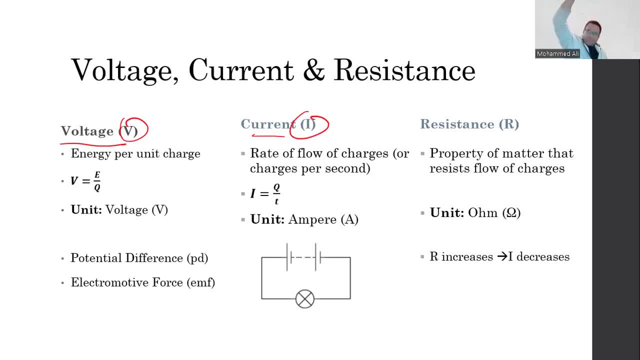 is electric current intensity. So they plopped the I from intensity and used it here, But we stopped calling it intensity a long time ago. We just called it current. but the letter I stuck And resistance, which is R, Very good. 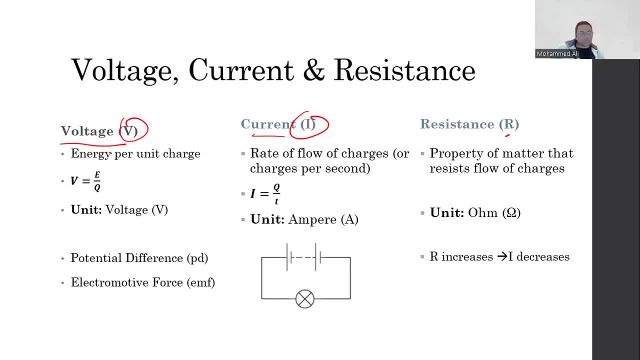 Now next up. what is voltage? Voltage is defined as how much energy there is per charge. How much energy there is per charge, And the unit is voltage. So, for example, a battery or a cell that has a voltage of 10 volts. 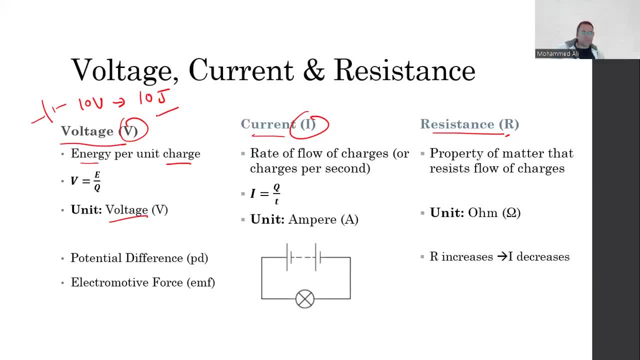 means it delivers 10 joules of energy per charge per coulomb. Like that, Every one of those circles carries 10 with it. It's calculated using: V equals E over Q, where V is voltage, E is energy and Q is charge. 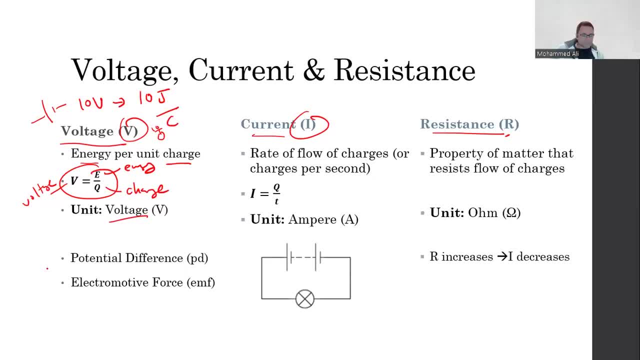 Now there are two different names for voltage, which we call potential difference or EMF- Electromotive force- potential difference. They both mean voltage, But potential difference is the voltage across something like the light bulb or a resistor, Whereas EMF is the voltage of a battery or a cell or a power supply. 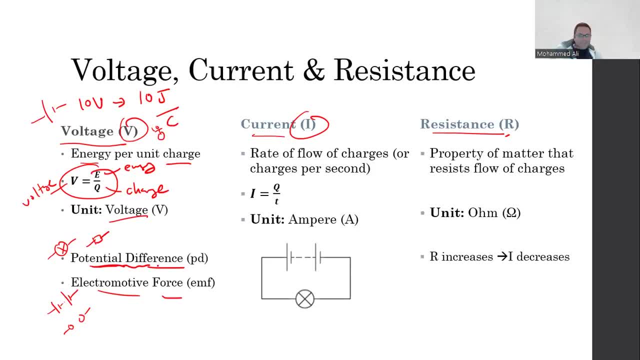 Why? Why is there a difference? Because this is technically energy lost by the charge, Whereas electromotive force is the energy gained by the charge from the battery. They're both defined as energy per charge, But potential difference is the energy lost by each charge. is the energy lost? 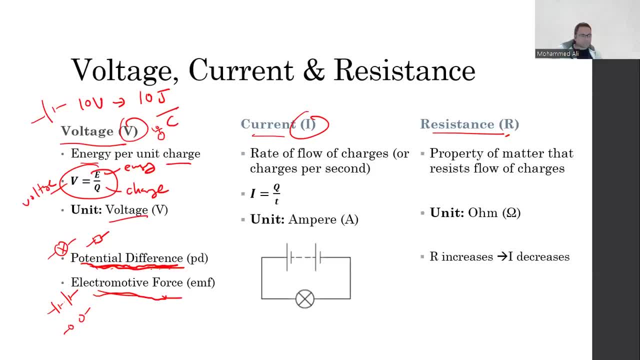 by each charge is the energy lost by each charge through a conductor, whereas electromotive force is the energy gained by each charge and it's used to drive the charge through the entire circuit. so we need that energy to push the charge through the entire circuit. very good. 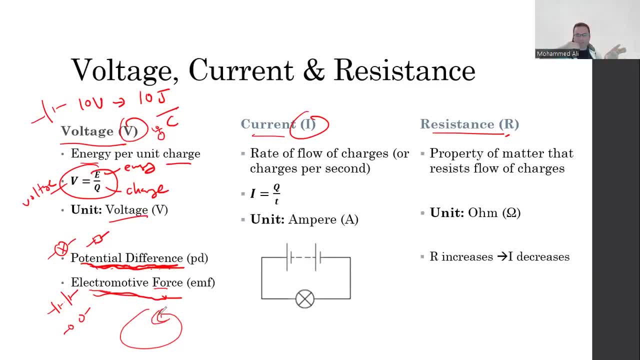 sorry for a second there. I froze for a bit because I realized I forgot to turn off annotations and somebody started writing on the screen. I know who you are, by the way. I know who you are. I'm going to go and find you. wait, I should do a Liam Neeson impression. 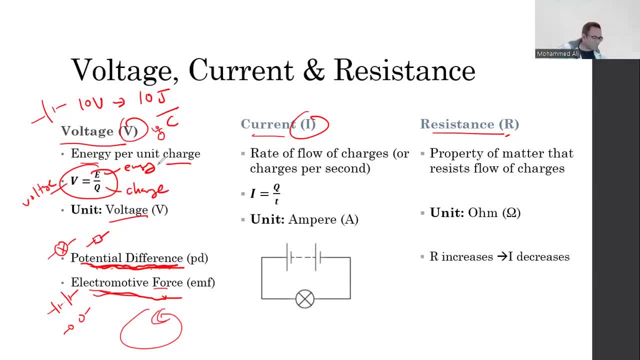 wait, wait, I'm going to find you. wait, no sorry, have you watched Taken? I love that movie. Taken is so cool. anyway, moving on, you should watch Taken if you have. anyway, what's current? current is defined as the rate of flow of charges, which is the number of charges. 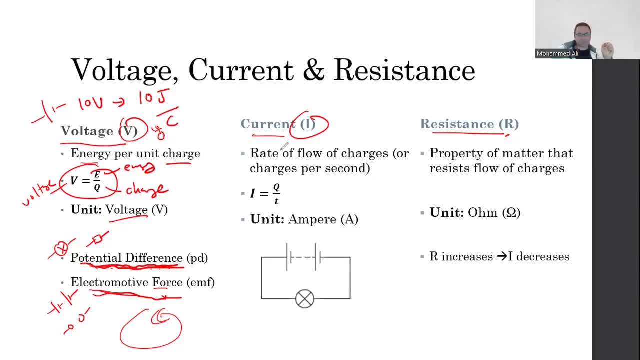 that go through the circuit per second. it's basically how fast the charges go around the circuit. the unit of measurement of current is ampere, so basically current is how many amperes or coulombs right charges go through the circuit per unit time per second. 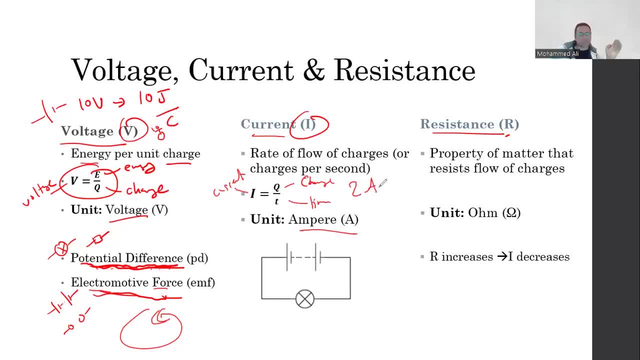 so if I tell you that a current in a circuit is 2 ampere, this means that you have two charges that go through the circuit every second. there are two charges that go through the circuit every second. speaking of the direction of the charge, the current often is from positive to negative. 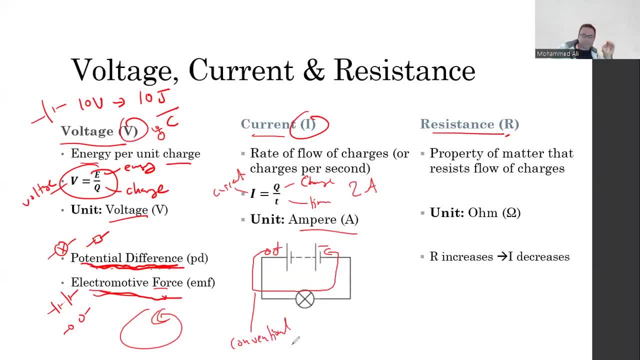 this is what we call the conventional current, but you will remember. you will remember that we said the charges that are free to move inside the circuit are the electrons. hmm, electrons are free to move. what's going on? the electrons actually move from negative to positive, so shouldn't the current be from negative to positive? 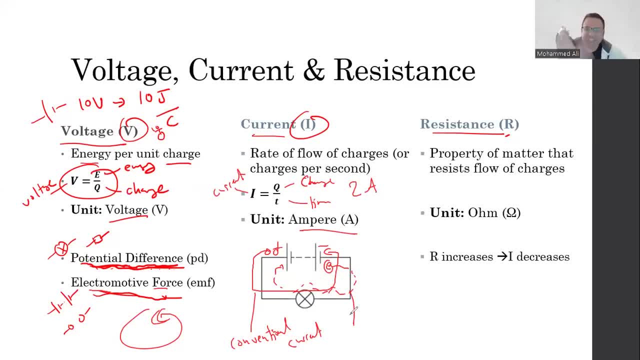 we say no, we know we made a mistake a very long time ago, but we're sticking to the mistake. the current will always be from positive to negative, but but to recognize the mistake, we also say that, hey, the charges that actually flow in the circuit are the. 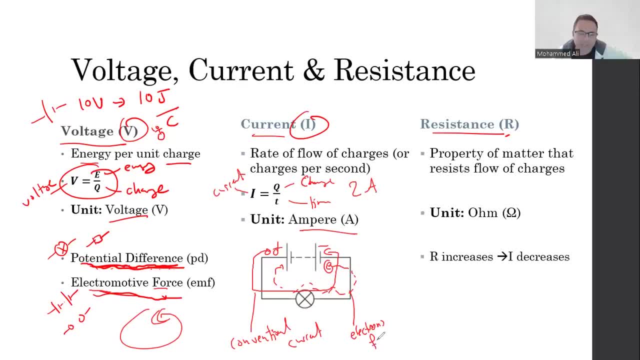 electrons, and the electrons flow from negative to positive. so if a question ever asks you to state what type of particle actually moves in the circuit, you say electrons. alright, but if i ask you what's the direction of the current, it's from positive to negative. electrons are from negative to positive. 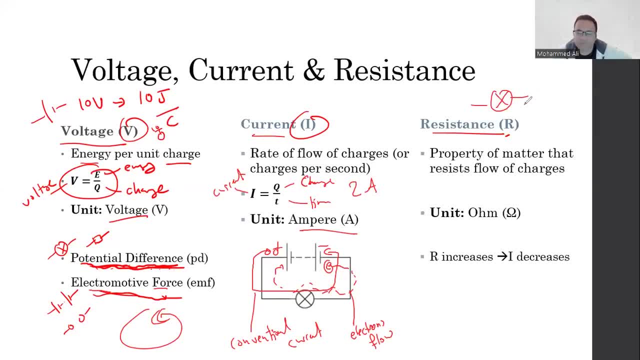 now, finally, resistance. that's the thing in the light bulb is a property that resists the flow of charges. but why? because inside any conducting wire there are atoms and these atoms are vibrating. so when a poor electron is trying to go through, because the battery is giving it a push. 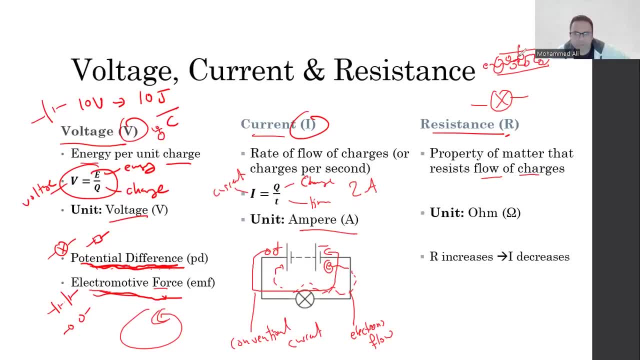 it keeps colliding with the atoms in the way, causing it to lose energy as it collides with the atoms. some materials are very good conductors, which means they have a lot of free moving electrons and very low resistance. the atoms are designed or arranged in such a way to allow charges to move freely through them. 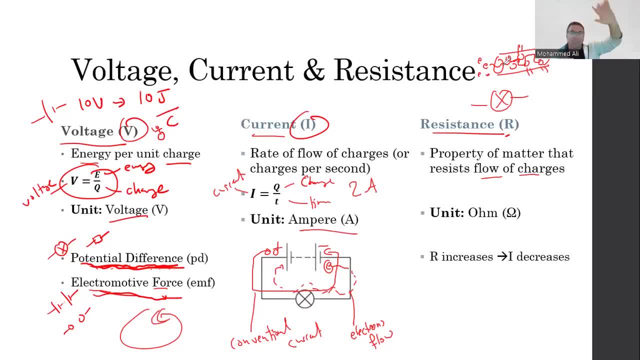 whereas some materials have high resistance, they have very few free moving electrons and the atoms are not really helping. so the basic concept is this: the higher the resistance of a material, the lower the current. so the current decreases and if you decrease the resistance going through of a material, 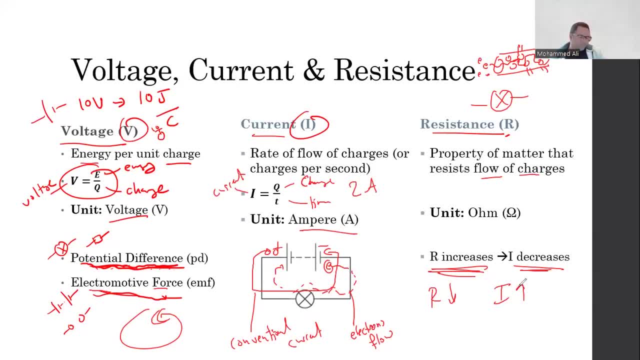 the current will increase. very good. the unit of measurement of resistance is called ohm, so the basic concept is this: the higher the resistance going through of a material, the lower the resistance going through of a material. the lower the resistance going through of a material- very good. 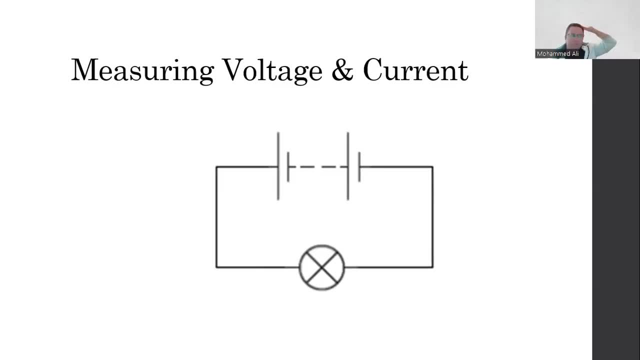 next, how do we measure voltage and current? like there are measuring instruments that we use to measure voltage, we use what we call a volt meter and it's always connected in parallel to the component that you want to measure. so if i ask you to draw a voltmeter connected to measure the potential difference across the 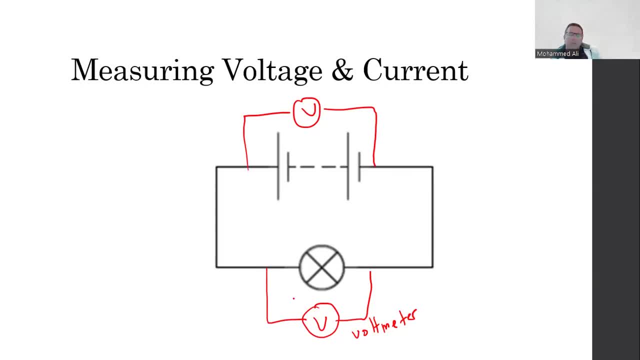 light bulb. this is where you connect it parallel to the light bulb. can i draw a voltmeter to measure the emf across a battery? then you connect it across the battery in order to measure current. we use an, a meter, which is used to measure current now, and a meter is always placed in. 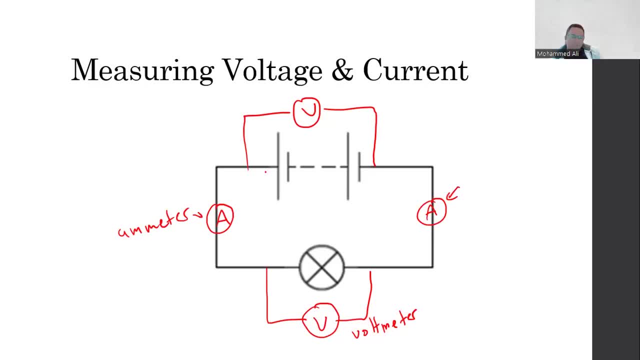 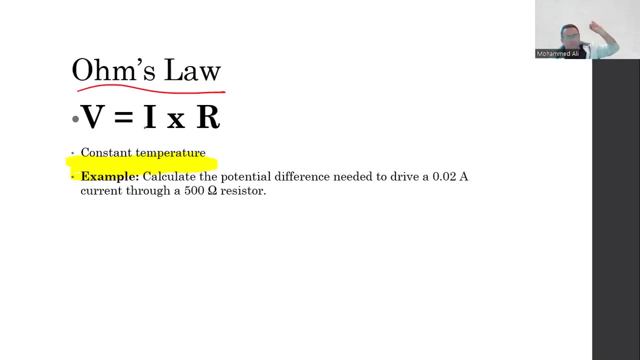 series in a circuit, and it doesn't matter if we put it here or here. as long as it's part of the same wire in the same circuit, the current will be the same, so it doesn't matter, good. next, the most important equation we have is ohm's law, which is literally an equation. 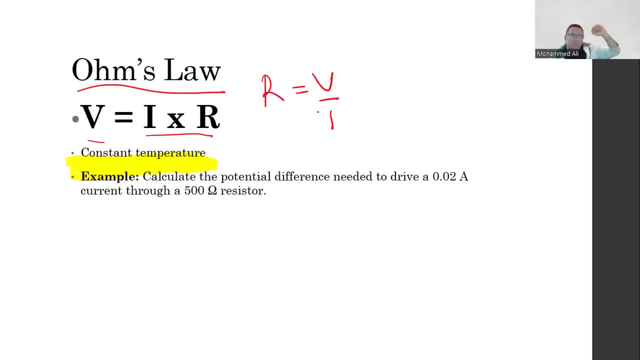 v equals ir. or you could just rearrange it and say r equals v over i, or you could rearrange it and say i equals v over r. rearranging this formula is extremely important. we're basically going to use this forever and ever and ever every time we solve electricity, so please keep that in. 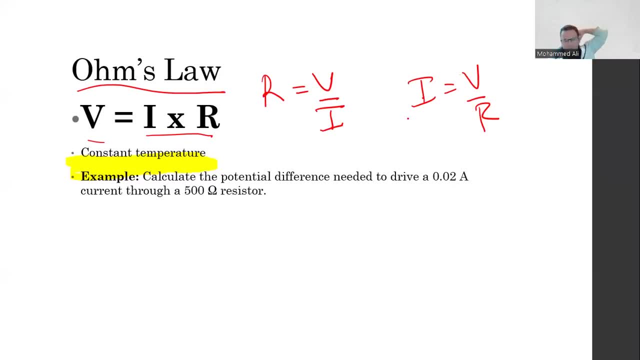 mind. all right. so here's one thing. though there's one more thing: the resistance of a resistor. the resistance of a resistor has to what be constant for this equation to work, because if the resistor keeps changing the values of the current, now the circuit will change. the resistance has to be constant. sure, a certain value of resistance will. 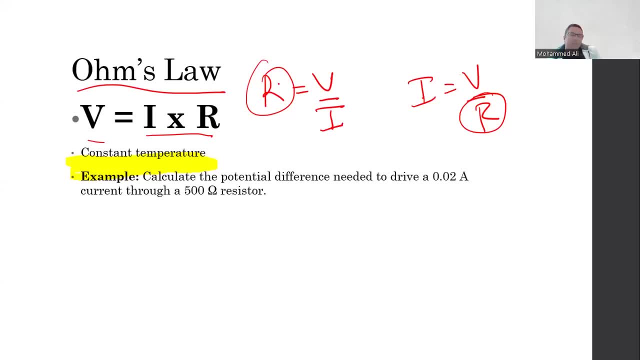 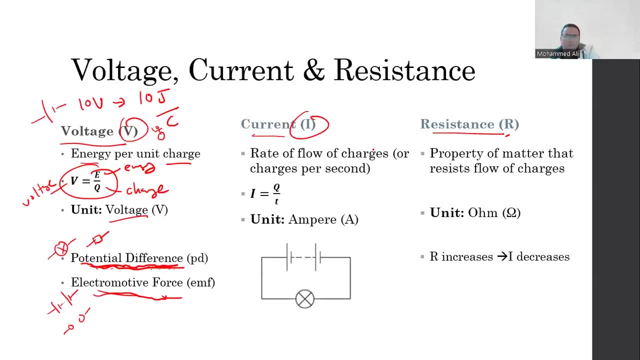 give you a certain value of current, but the resistance still has to be the same and for it to be the same, the temperature has to be constant. now you may be. you might be wondering why, because if you go back, remember i said resistance exists because atoms and a material cause the electrons. 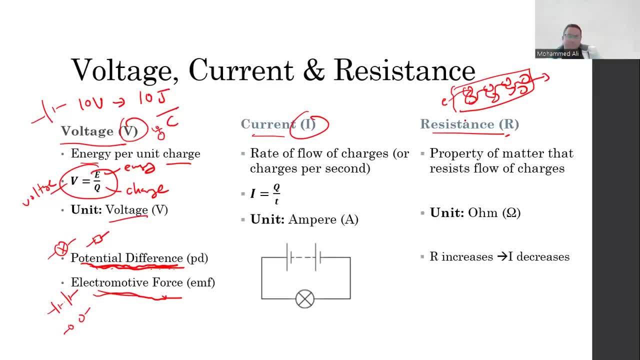 to bump into them. so they resist, right? if you heat up a metal object, these atoms vibrate faster and as they vibrate faster they collide harder with these electrons, making it even harder for them to go through. yeah, they keep colliding, a lot and a lot and a lot. 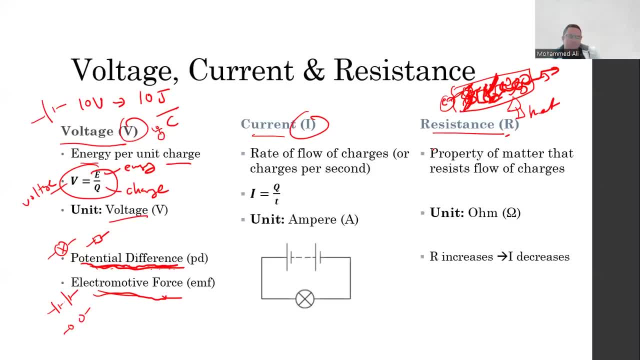 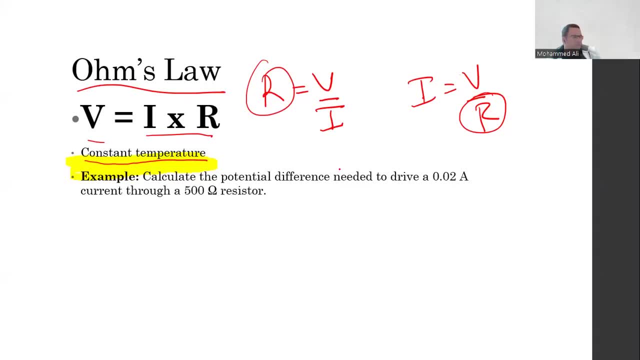 until they finally were through all right. so temperature has to be constant. now let's use this equation before i answer a question that was set. calculate the potential difference, that's voltage needed to drive an 0.02 ampere current. so that's current through a 500 ohm resistor. That's R. That's easy, I want. 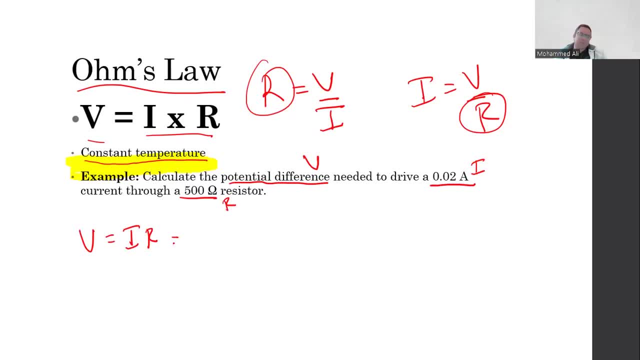 V. So V equals IR, I is 0.02.. R is 500.. So 0.02 times 500.. This gives me 10 volts. There's nothing special. If anybody has any questions, send them now, But I'll be answering a question here as. 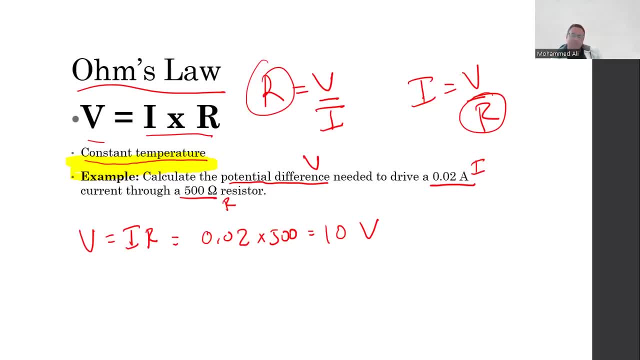 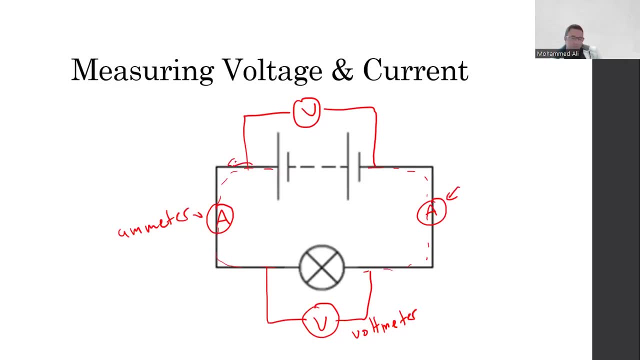 well. So how will the current be the same if a device has resistance? Well, I'm saying the current will be the same throughout the entire circuit. So, for example, if I tell you, hey, the current is 0.02, the speed of the charges will be a constant 0.02 from the very beginning. 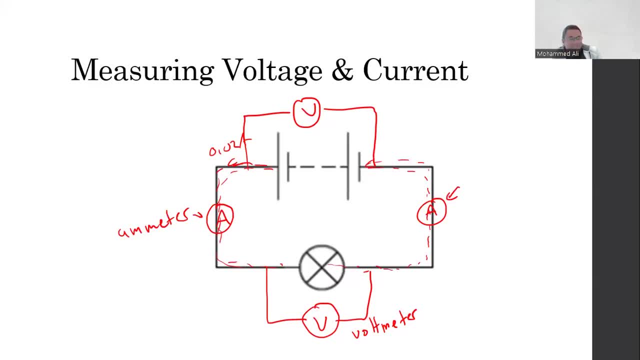 to the end. It won't change. It has that value from the beginning because the battery already knows what the resistance is. So when it releases a current, I equals V over R. it already knows what its voltage and resistance are. So it gives out the current at that fixed speed from the beginning. It doesn't change. 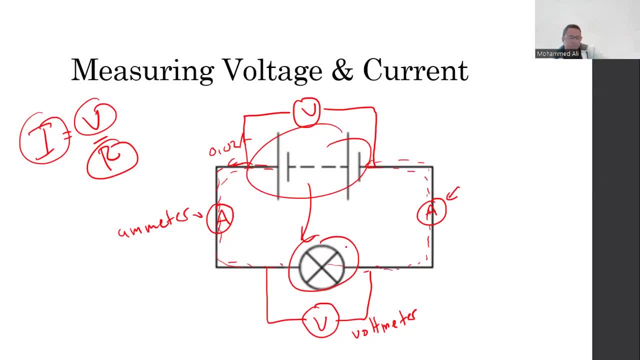 Gives out the current at a fixed speed from the beginning, with no change whatsoever. If you increase the resistance, as in you add another resistor or you change this lamp to one with a higher resistance, the current will decrease, but it will still be constant throughout the same wire. 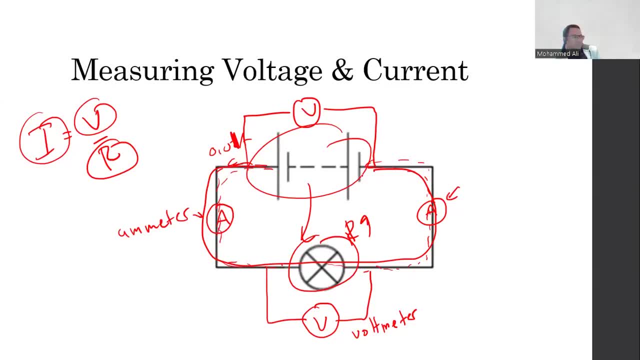 All right, The resistance has decreased the current, but it does not decrease inside the lamp only No, no, no, no, no, no, no. It decreases from the very moment it leaves. So, Ash, here's the thing. 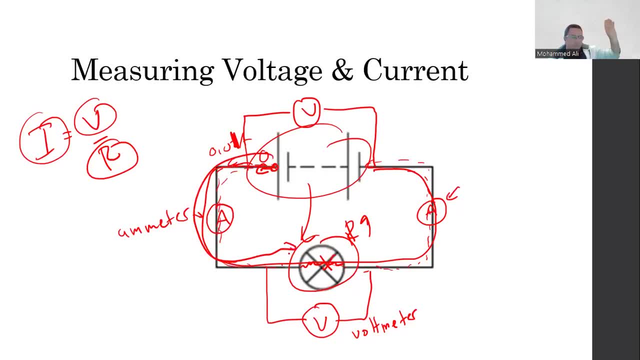 Lots of people have this image: Charge leaves super fast. Oh my God, there's resistance, I have to slow down. And then, once it leaves super fast, No, it doesn't do that. What happens? God, that's silly. 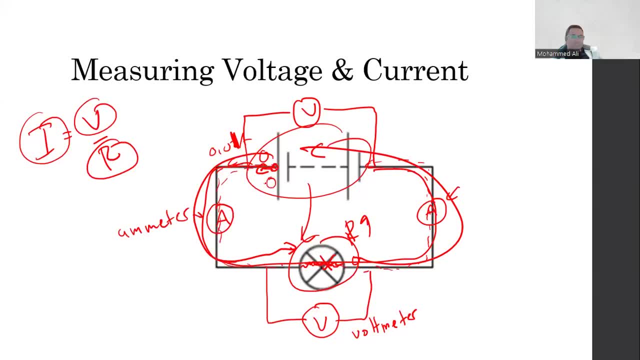 What happens is this: The charge leaves and moves at the very low current that it will be moving with through the lamp. Now you might be wondering why, Why? Why would it do that? Because, if you remember the very first story, all of these charges move together. 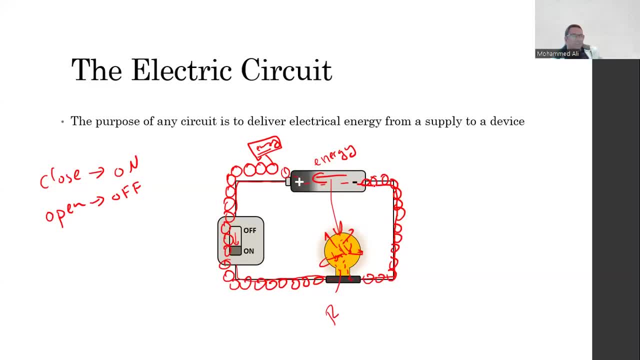 They're like a big chain, like a train In Arabic it's like a train. If one of them slows down, all of them have to slow down and move at the same speed, So it doesn't move fast and then slow and then fast. 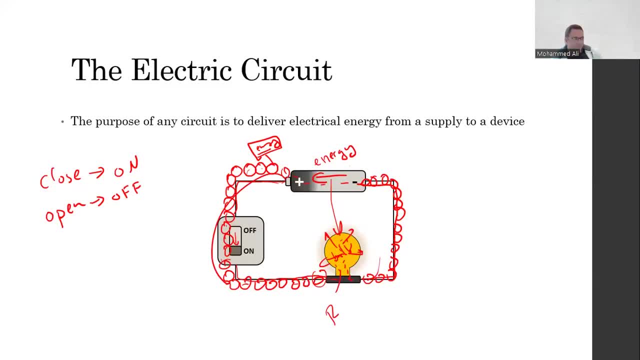 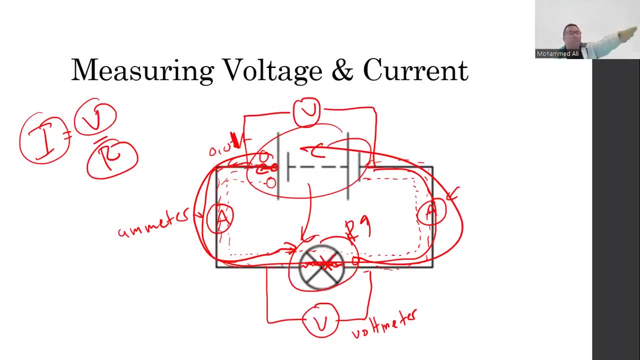 No, it just moves at the same speed from the beginning. Okay, How does resistance? How does resistance affect voltage? That's the second question. For now, it does not affect voltage. For now, resistance does not affect voltage. You want to know why? 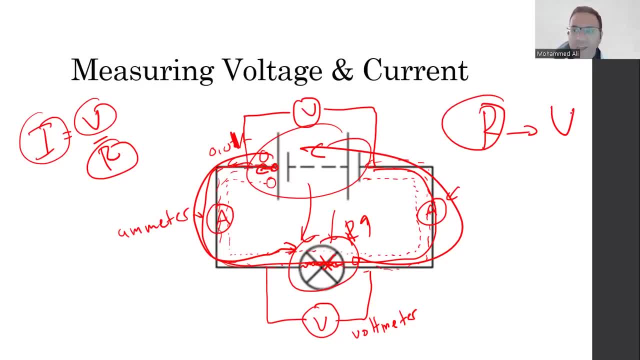 Because I choose which resistance to put in using the lamp, I choose which voltage to put in using the battery. They don't affect each other. They both, however, affect the current. The poor current gets slapped around by resistance and voltage. However, this will change in a little bit. 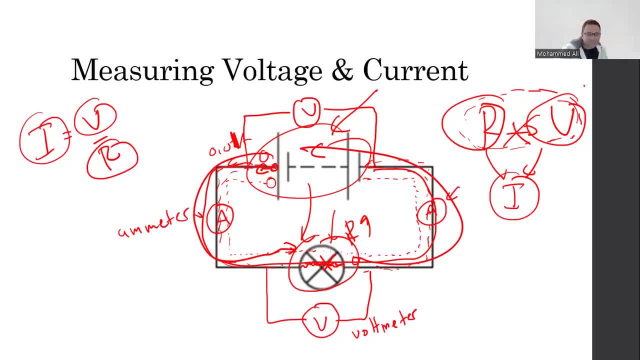 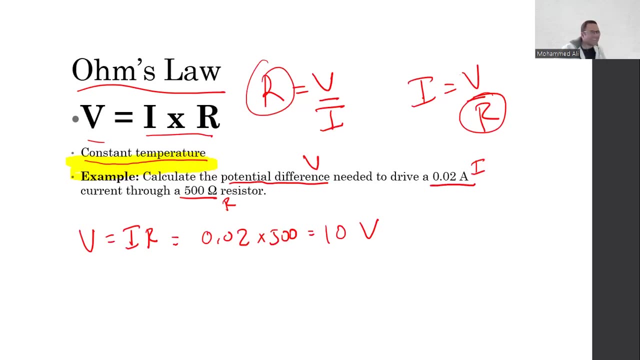 This will change in a little bit. I have a third question which is extremely important. Where is Mr Yu? I don't know. He retired. He saw the 2023 syllabus and retired. Anyway, Thank God some people remember the OG videos. 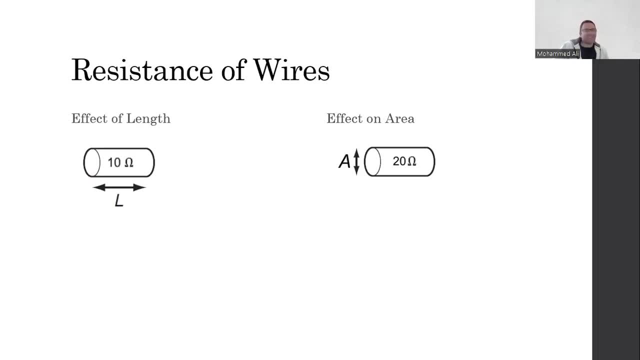 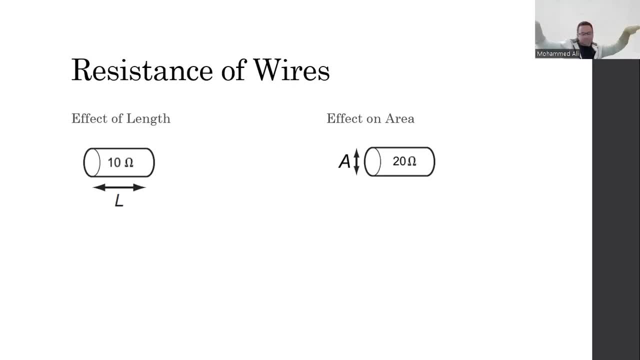 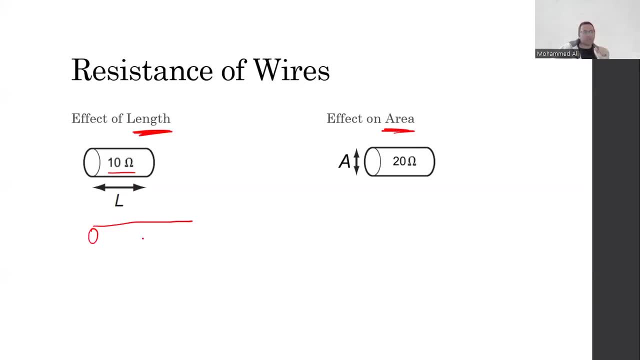 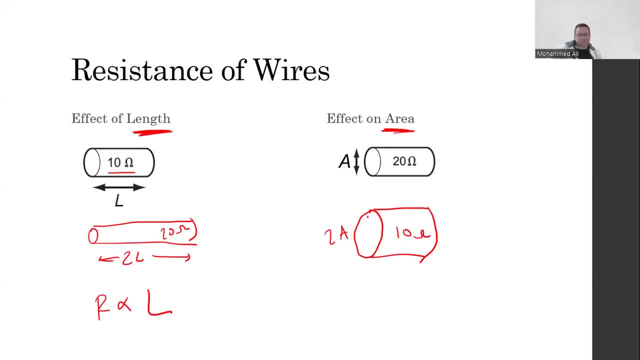 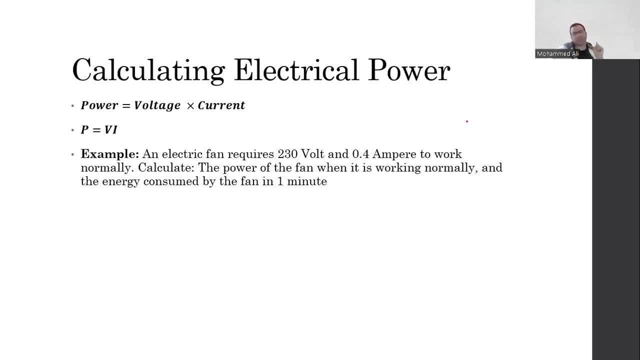 If you remember, in unit one we defined a very important quantity called power. Power was defined as energy over time. Power is defined as energy over time, But in electricity we don't measure energy and time. we measure voltage and current using a voltmeter and an emitter. 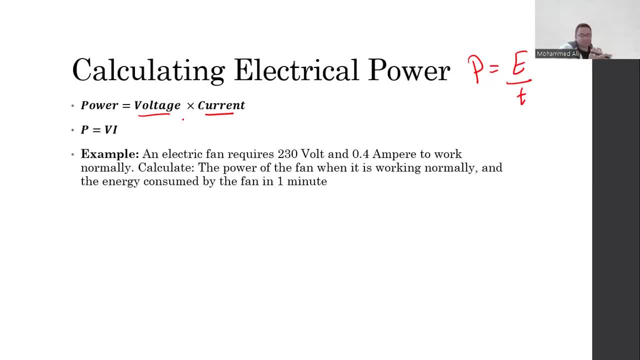 So we calculate power using V times I. No fanfare, it's just V times I. If I want to calculate energy, you go back to unit one. energy is power times time. If you can get energy using V times I, then it'll be V? I times time. 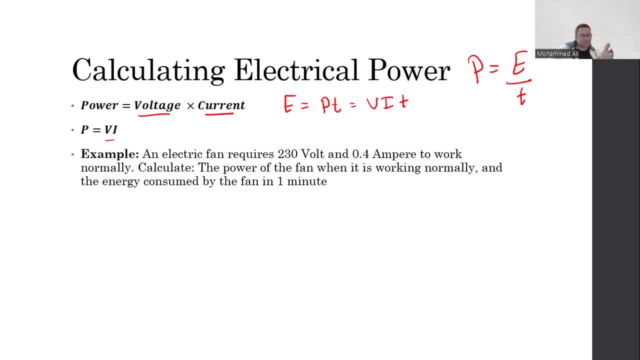 I'll replace power Power with V I. Let's see how we can use this. Here's an example. An electric fan requires 230 volts and 0.5 ampere to it, So voltage and current Calculate the power of the fan. 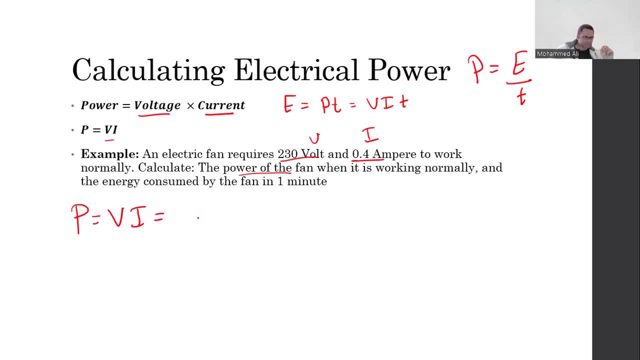 Okay, cool Power equals V times I. So what's V? 230.. What's I? 0.4.. This gives me 92.. Fantastic Watts. But then calculate the energy consumed in one minute. So now he wants energy. 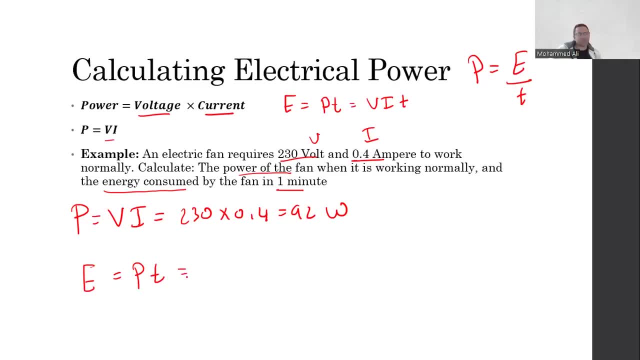 Now I know from unit one that energy is power, times time. So power is 92 watts. We just got that. Times time, which is one minute Time, has to be in seconds, So you multiply it by 60.. So 92 times 60,, which is 5,520 joules. 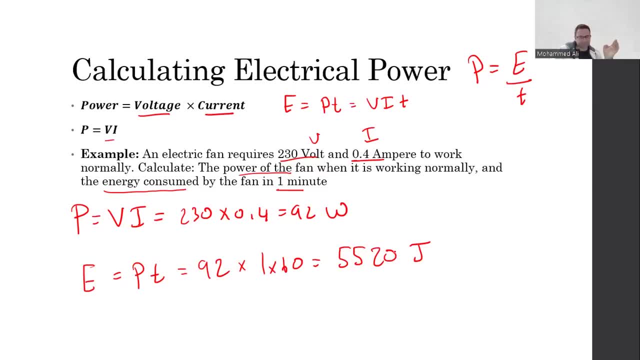 These have not changed Very good. As a final point, here there are two other versions of this formula. So if you take P equals V I and you join it together with V equals I. R using some, you know, clever math and substitution. 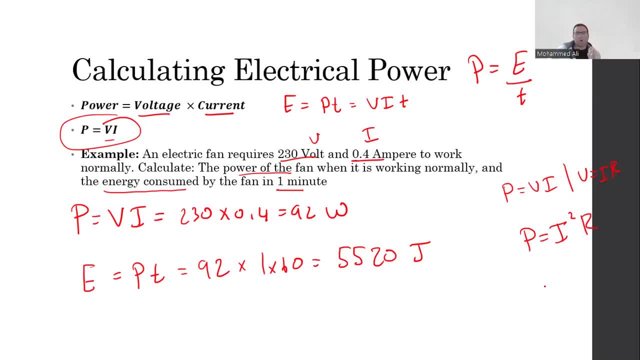 you end up with P equals I squared times R, or P equals. that's not a P. Give me a second: P equals V squared over R. These are simply P equals V- I, and we've replaced the V with I R once. 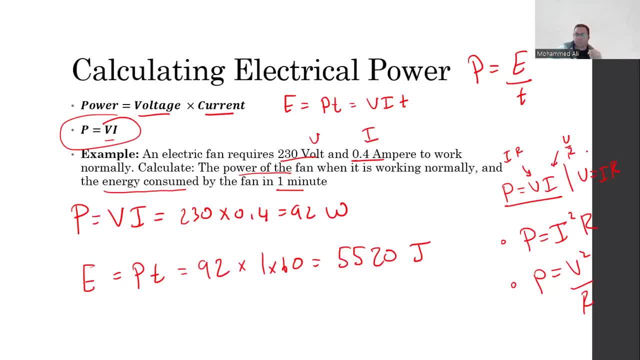 Or we've replaced the I with V over R once. You don't need to know the proof of them, Just know that these are two other versions of the same formula. What I recommend is, you don't really have to memorize these. If you do, that's fantastic. 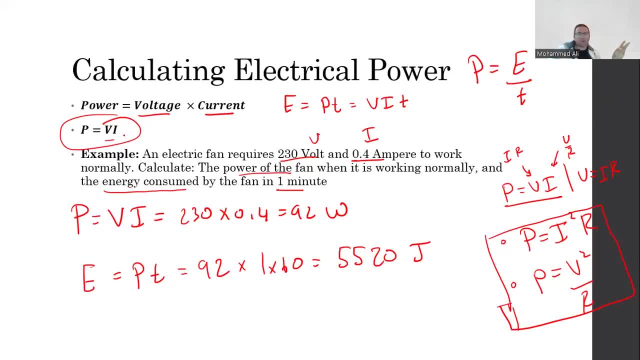 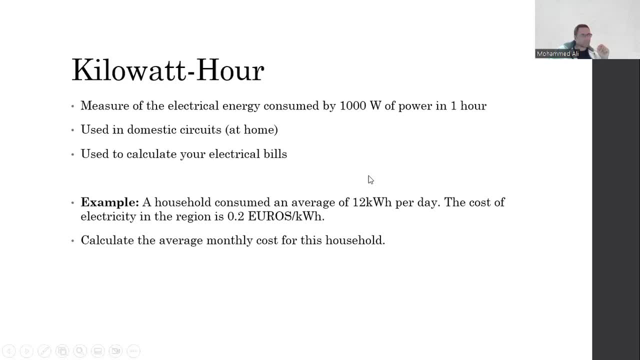 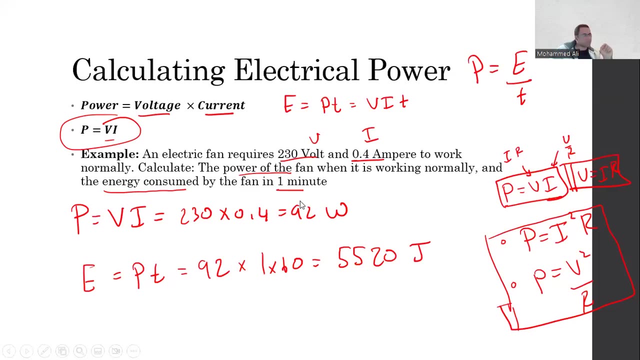 It'll make some questions easier for you, But if you already know and you've memorized, P equals V times I and V equals I R, you're set, You're fine, All right, Let me answer a question regarding this example we solved. 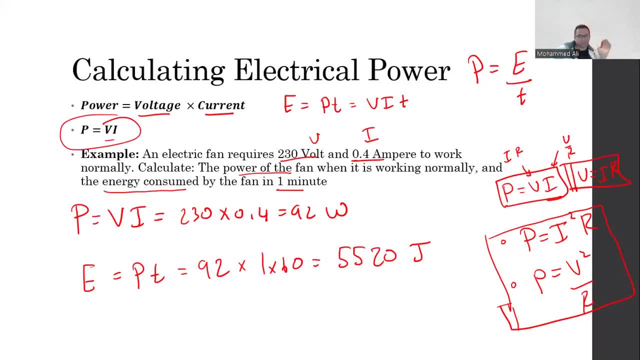 When do we turn the minutes to seconds when calculating energy? Always The unit of energies in joules. that's based on the SI units that we discussed earlier, And SI units are kilograms for mass, meters for distance and seconds for time. 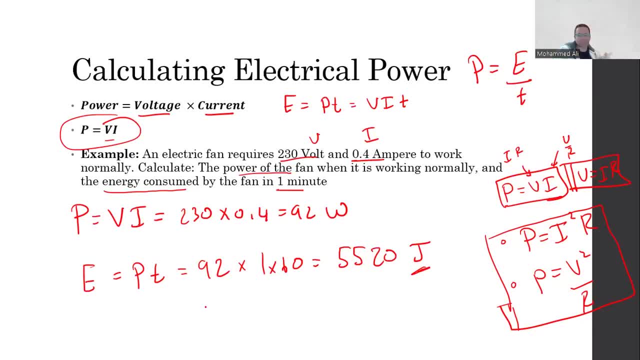 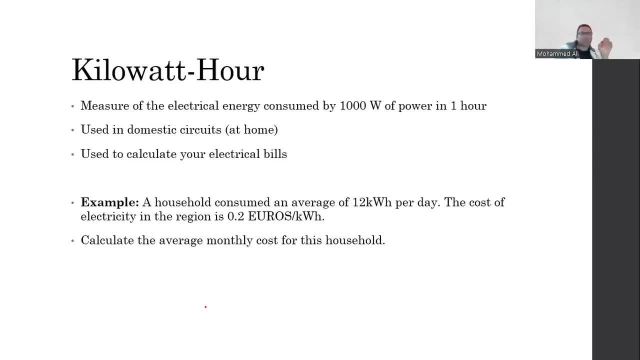 So it has to be in seconds. It must be in seconds. Next, There's an extra unit of energy that we use at home called the kilowatt hour. You probably don't see it at all unless you pay the electricity bill or you look at the electricity meter and you see how much you have to pay. 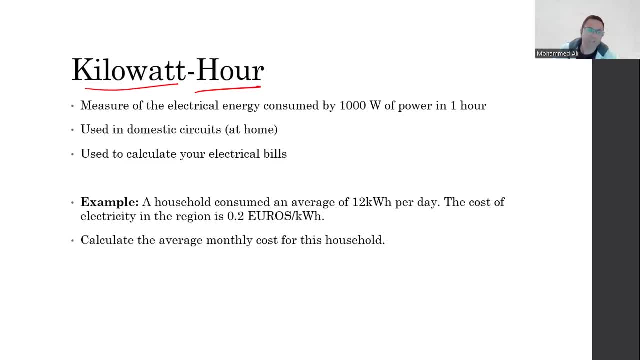 They don't tell you how many joules you consumed. They always tell you how many kilowatt hours you've consumed. But what is a kilowatt hour? It's defined as a measure of the energy consumed by 1,000 watts of power in one hour. 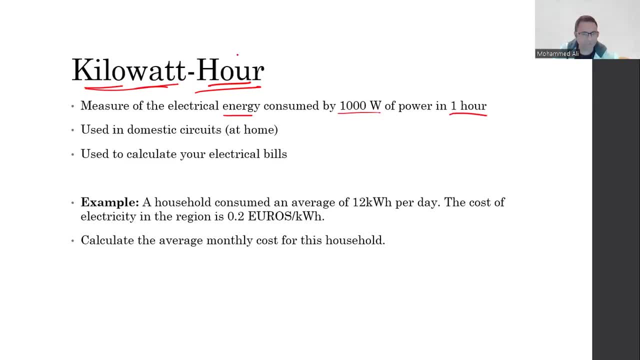 Literally: 1,000 watts, kilowatt in one hour. Try the math. Energy is power, times, time. What's the power? 1,000 watts. What's the time? One hour. How do I convert one hour to seconds? 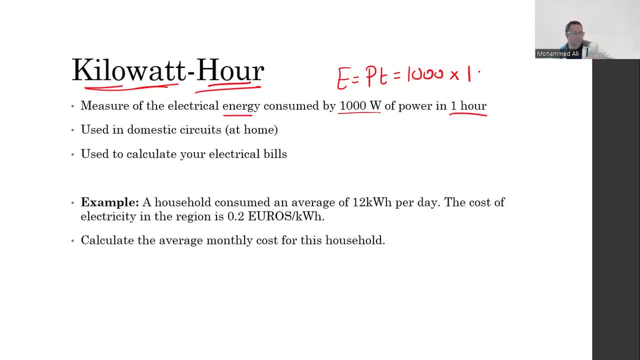 Because we need to remember that. So one hour to minutes is times 60. And then one minute to seconds is another times a 60. So what does that give us? 1,000 times 60 times 60. This gives me 3,600,000 joules. 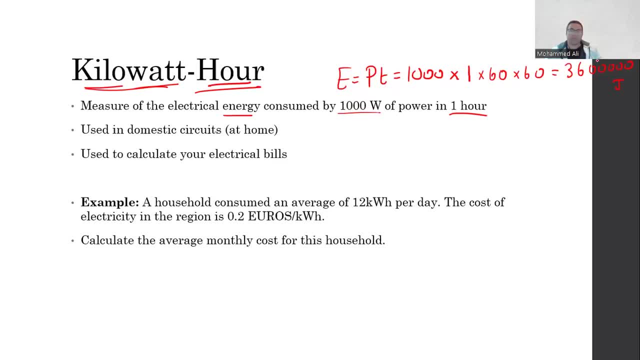 All right, Very good, Now you don't have to memorize this. but this is the value of energy, the amount of energy in a single kilowatt hour. So it's designed to help us limit the numbers we use at home. 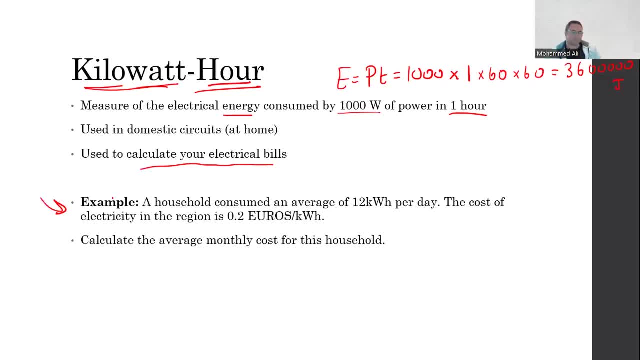 So how do we use it to calculate your electrical bill? Here's an example. I tell you that the household consumes an average of 12 kilowatt hours per day. So every day, this is the amount of energy they use up: 12 kilowatt hours. 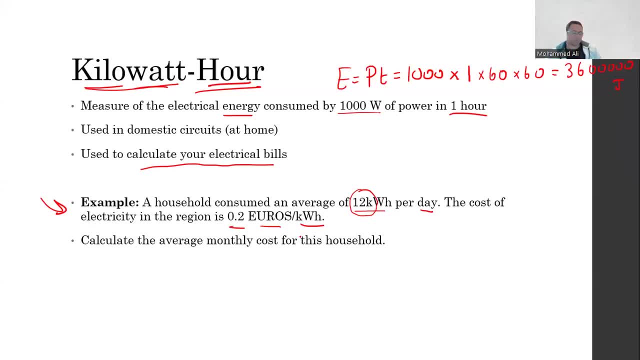 The cost of electricity is 0.2 euros per kilowatt hours. How many euros is this? You could replace euros with dollars, with pounds, with whatever pesos, whatever currency you want, It doesn't matter. So what's the monthly cost for this house? 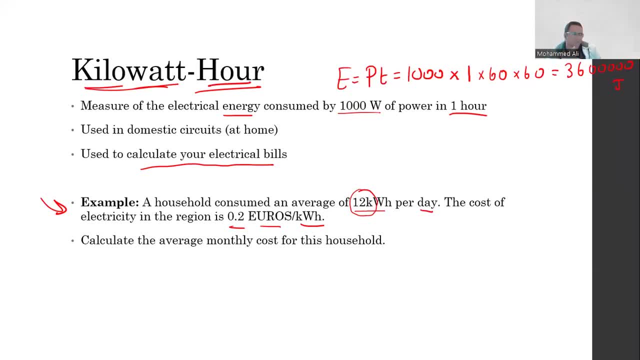 So wait a second. If I consume 12 kilowatts in a day and I want the amount of energy they use up in a month, how many days are in a month? One month has 30 days, So the first step is we're going to multiply 12 by 30.. 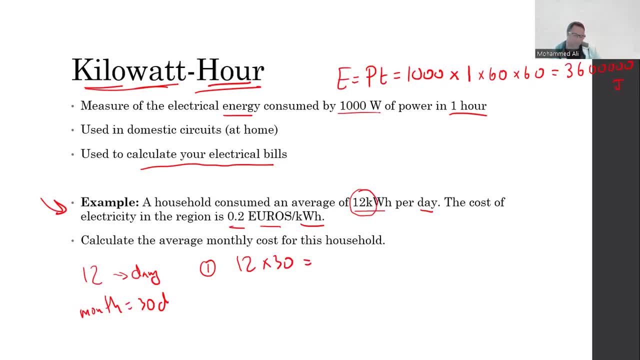 So we get the total amount of energy 12 times 30.. This gives us 360 kilowatts hours. That's the total amount of energy. So what's the cost of this? How much money do I have to pay? So the cost is going to be 360 times 0.2.. 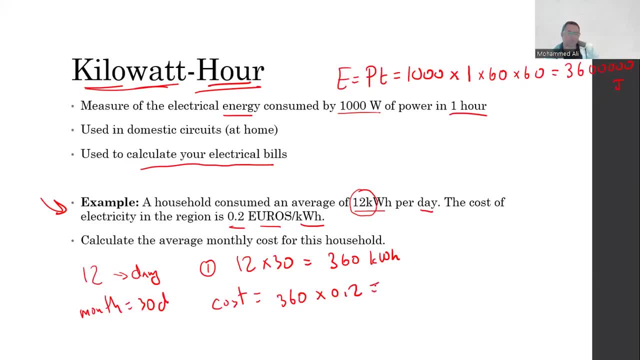 If one kilowatt hour costs me 0.2 euros, then how many euros am I going to pay? 360 times 0.2 gives me 72 euros, And that's the amount of money I have to pay for this energy. 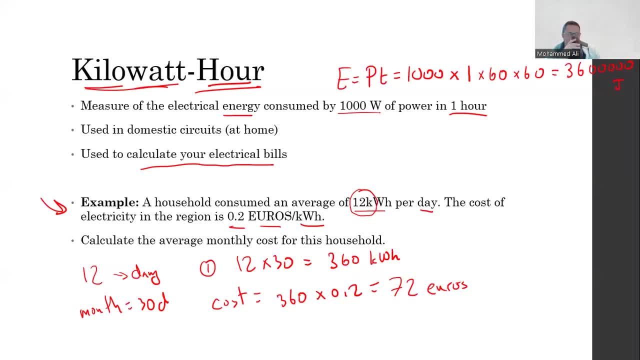 Very nice. So all we're saying is this: You take the total amount of energy per day. This is a math question. This isn't really physics anymore. If it takes, if it's a cost of 12, if they use up, 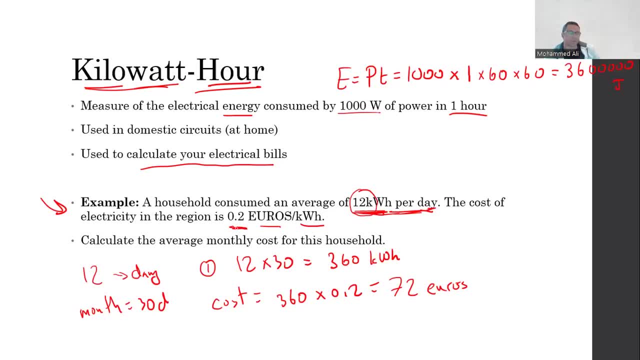 sorry, 12 kilowatt hours per day, and each kilowatt hour costs me 0.2 pounds, for example. then how many pounds have you used up, Or how many pounds do you need to pay in a month? What's the total cost? 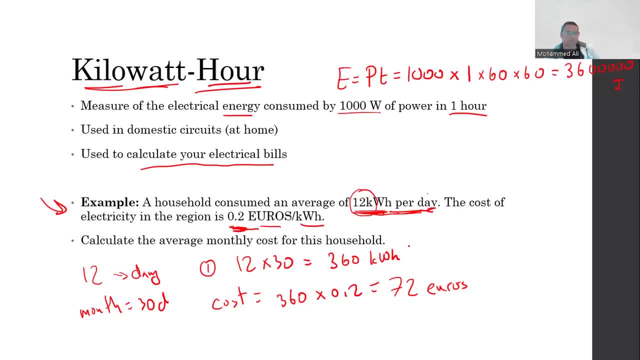 So it's 12 kilowatt hours in a day. 12 times 30 gives me the total energy expenditure, How much energy I used up. Then you multiply it by the price of a single kilowatt hour, So 0.2 times 360.. 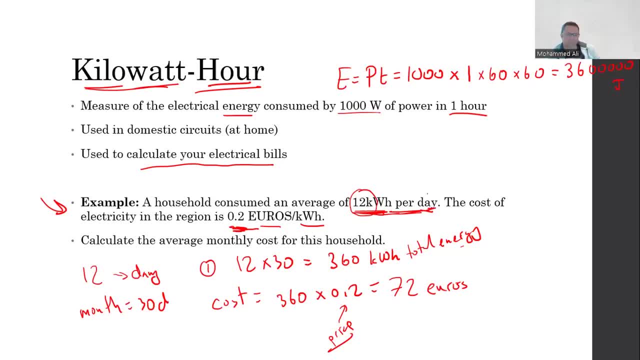 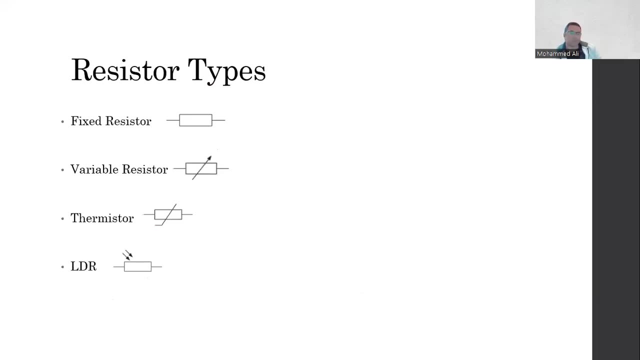 This gives you 72 euros. It's a math question more than anything else. Honestly, it's not a physics question, But still it's important to understand just the concept of the kilowatt hour Next up. Obviously, circuits or current electricity will not be complete unless we talk about resistors. 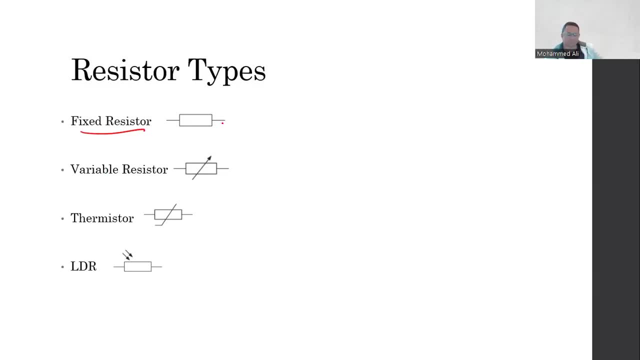 We have several types of resistors: A fixed resistor which has a fixed resistance: It just has resistance. A variable resistor whose resistance changes. A variable resistor whose resistance changes- How does it change? Based on length? Sorry, based on length. 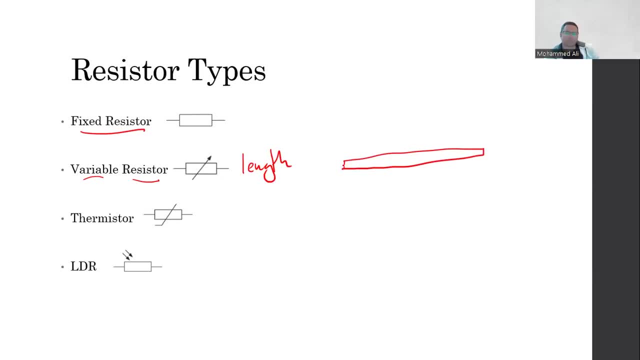 So if you have a long resistor wire, you connect to a circuit and you have a sliding contact. If you move the sliding contact right and left, you change how much of this wire is in the circuit. So this entire wire is 100 ohms. 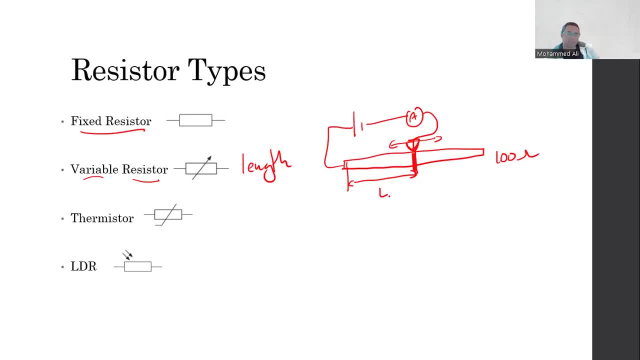 And you put the sliding contact in the middle. This gives you a resistance of about 50 ohms. This gives you a resistance of about 50 ohms. As you slide it to the right, the effective length in the circuit increases, So this takes up more space. 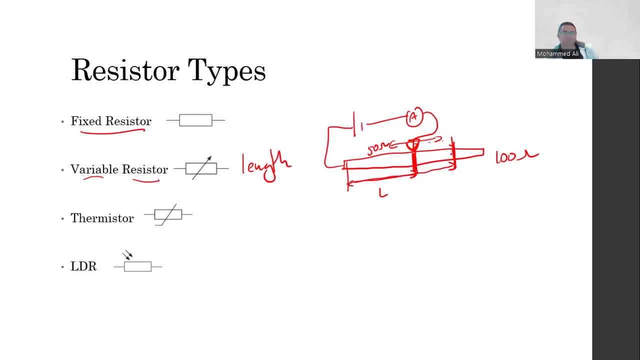 And as it takes up more space or the length increases, the resistance increases. So the resistance increases. It's like 75 ohms, for example. Maybe it's 80. As you move it to the left, the resistance decreases. 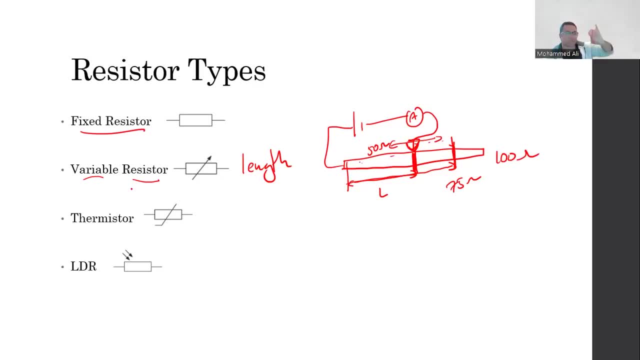 From its name. it's literally a variable resistor, A resistance that's variable. A thermistor is also technically a variable resistor, But it changes based on heat, on temperature, On A, on temperature. The hotter it is, the higher the temperature. 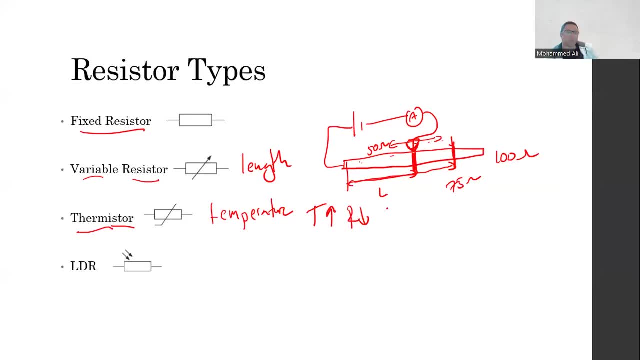 the lower the resistance of the thermistor And the lower the temperature of the thermistor, the higher the resistance. This is completely opposite to what we said a little while ago regarding fixed resistors, when we defined resistance, Because thermistors are made of non-metallic conductors. 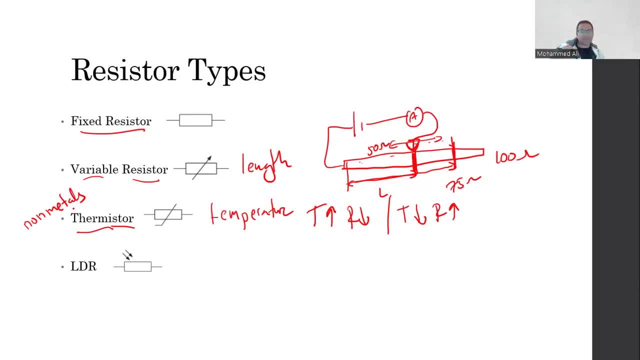 Non-metals, when heated, gain more free-moving electrons, So they become better conductors, So they conduct electricity better. Again, non-metals, when heated, conduct electricity better. This is why when the temperature increases, the resistance decreases. 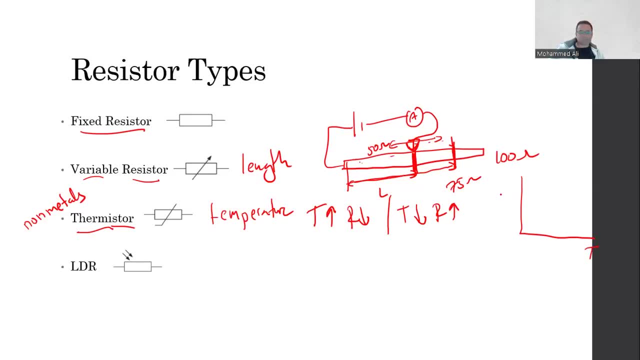 If you draw a graph of how the temperature changes or affects the resistance, it'll be inversely proportional. like this: The LDR is short for light dependent resistor- Light dependent resistor, So it depends on light. clearly, When the amount of light 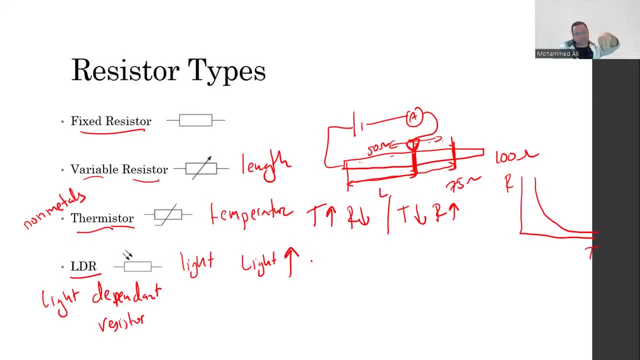 hitting the surface of the resistor increases, the resistance decreases. It's just like the thermistor, by the way, But it's not sensitive to temperature. It's sensitive to light, And if the light on it decreases, its resistance increases. It is very important to realize. 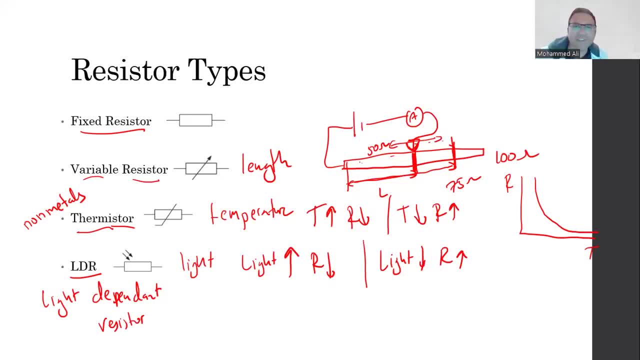 the LDR doesn't emit light. It receives light- okay, It's not emitting light. So when you put it in the dark or you cover it, the light on it decreases, So it gets a high resistance, And vice versa If you put it in the sun. 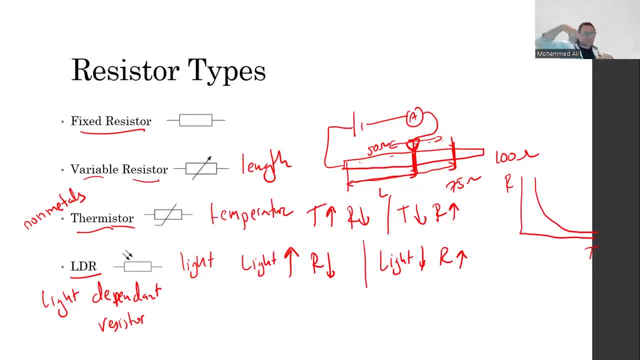 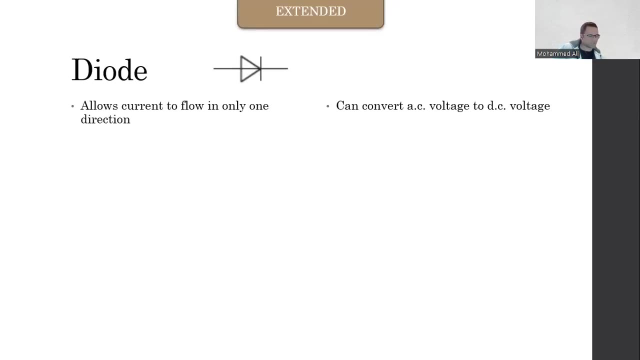 or in front of a light bulb. the light on it increases, so the resistance decreases. Very good. Now the last thing is not really a resistor per se, but you know what It kinda is. It kind of is: This is called a diode. 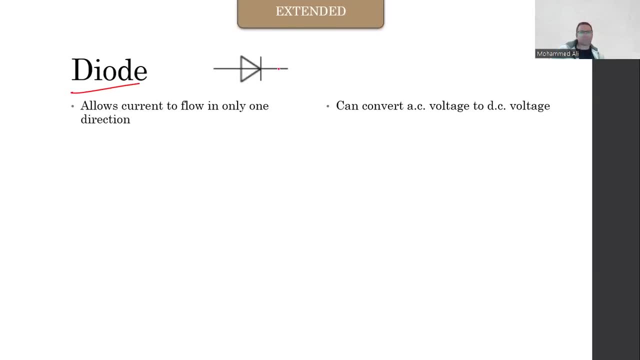 What's a diode? It's kind of like a resistor, but it only allows the current to flow in one direction. Remember, this is extended huh. If the current is flowing through the diode in the direction of the arrow, it goes through. 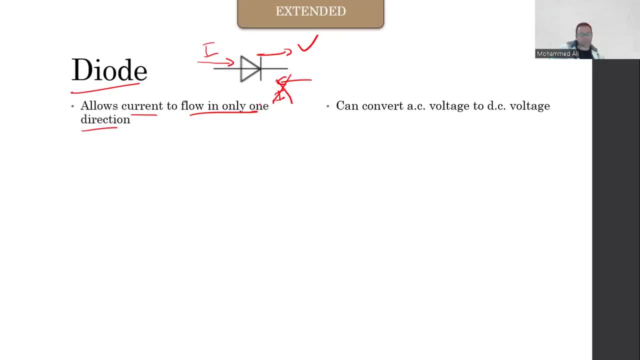 If the current tries to flow in the opposite direction, it does not go through. So it's basically a one-way gate. So here's a quick circuit. Here's the same circuit, but I'll connect the diode in reverse. This light bulb will light up. 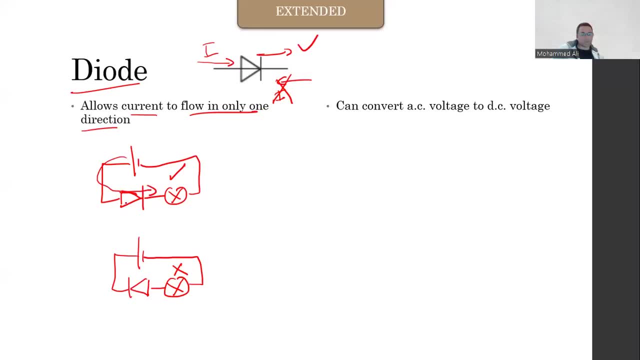 This will not Why. Because this light bulb, this diode- sorry- allows the current to go through. This does not allow the current to go through, because it's in the opposite direction. You don't really need to remember these terms. 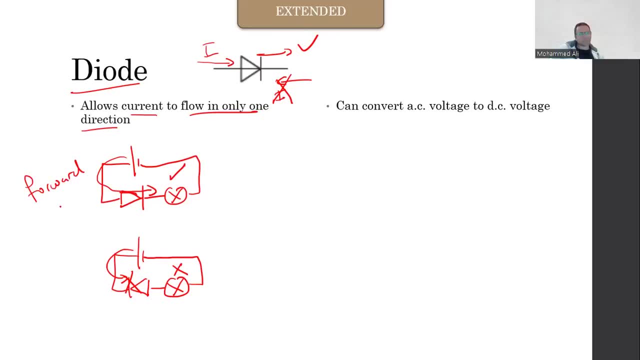 but when the diode is connected in such a way that it allows the current to go through, it's called forward bias. When it's in the opposite direction, we call it reverse bias. But again, that's not very important. Now the main function of a diode. 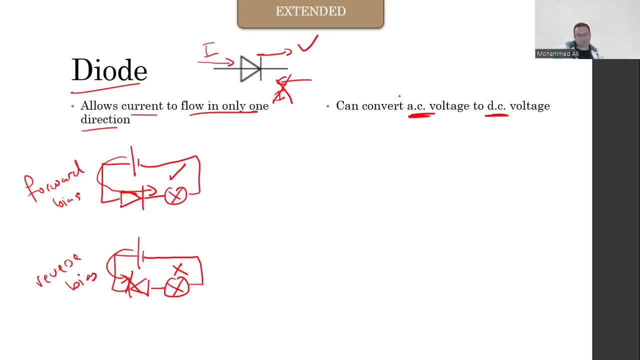 is to convert an AC voltage to a DC voltage, so alternating current to a direct current. If you don't know, a direct current is the current from a battery or a cell. It has a positive and negative charge. The current flows through in a single direction. 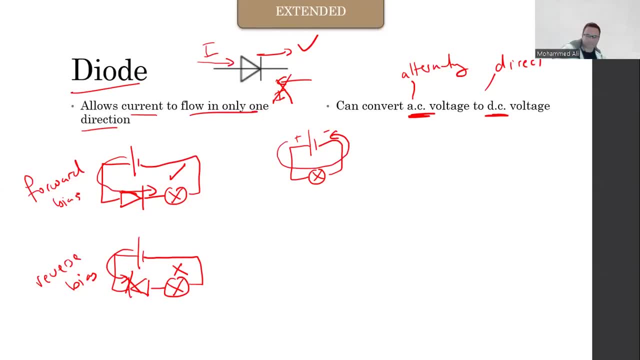 It doesn't change And it has a constant value. It's direct. This is called DC. However, an electrical socket or a generator produces what we call an alternating current, AC. What does that mean? This means that for like a portion of a second. 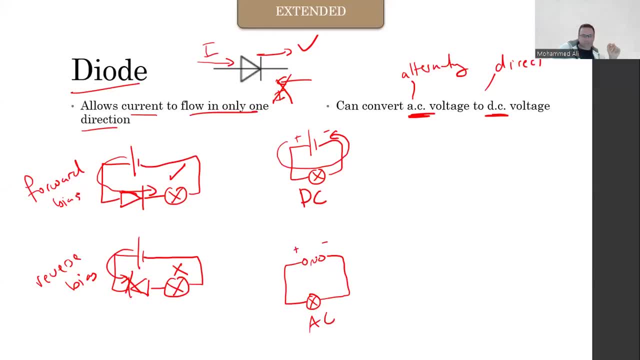 0.2 seconds, for example. this side is positive and this side is negative of these terminals. So the current flows from positive to negative, here And in the next 0.2 seconds, this is positive and this is negative. So the current flows. 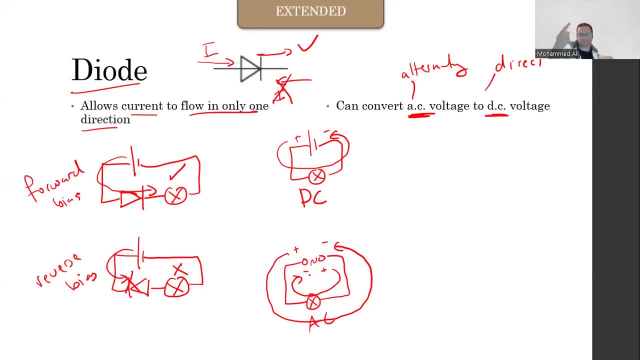 in the opposite direction And it keeps alternating. It keeps changing. All electrical sockets are AC. This is the graph for a DC voltage over time. This is the graph for an AC voltage. over time It changes. So how do you use a diode? 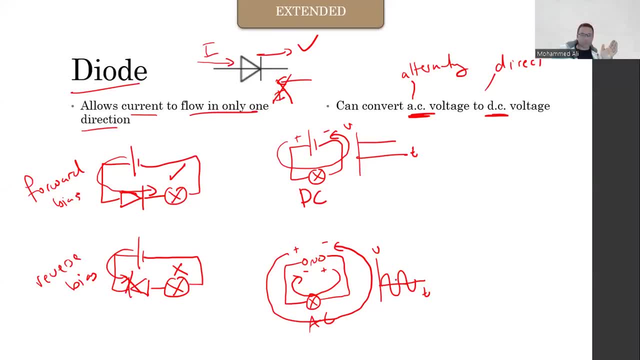 to change AC to DC. Well, it's quite simple. If you just put one diode, it'll only allow part of the current to go through and the other part will not. It will only allow part of the current to flow through and the other part will not go through. 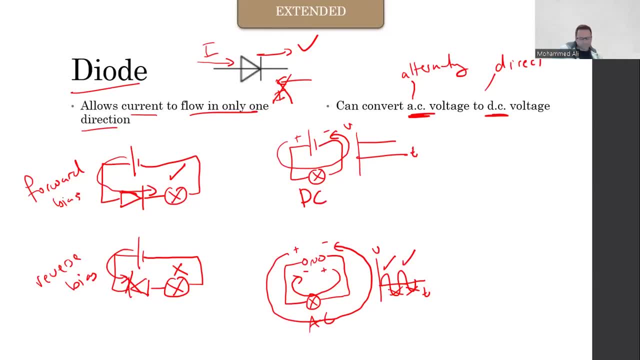 However, if you connect four diodes together, this will completely convert an AC voltage to a DC voltage. You do not have to memorize the order of the diodes. Just understand the flow of the current. Just understand the flow of the current. 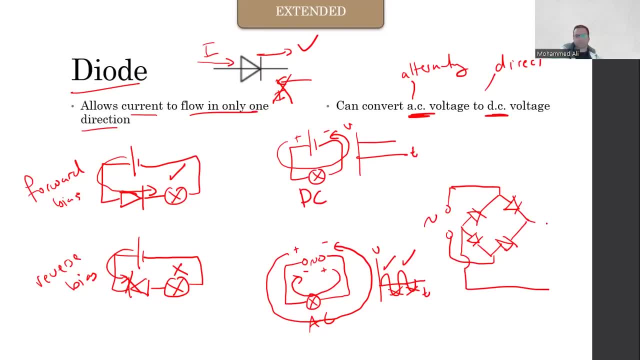 If this is the AC supply, then this is the resistor. that's the output. Maybe there's a light bulb, Maybe there's a voltmeter, It doesn't matter. Take a look at this If this is the positive side of the battery. 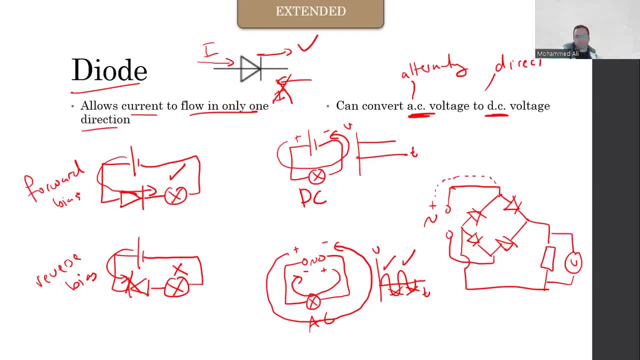 and the current goes this way. here it'll head to the right, Here it'll head to the right again, And there we go. It's gone through the resistor If the direction of the positive side of the battery or the supply has changed. 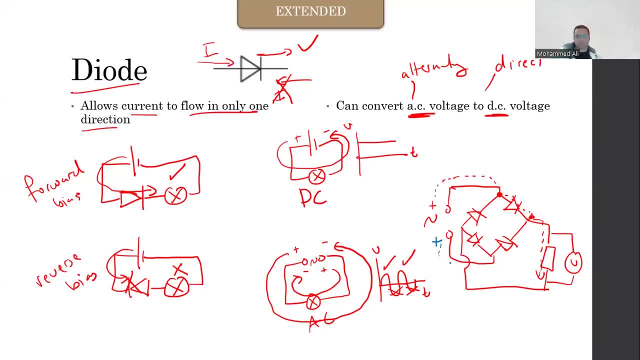 now. this is positive. I'll change the color now. The current will flow this way: Reach this junction Left or right, it'll go right, And then left or right, it'll go right, And bazinga, The current has gone. 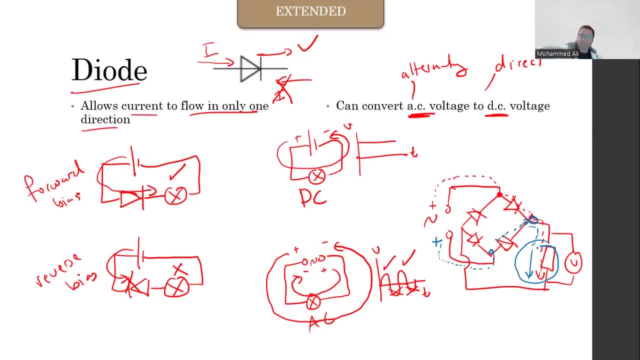 through the resistor in the same direction, even though the supply has changed the direction of the current, Even though the supply has changed the direction of the current. Don't memorize this, but understand that if you input an AC voltage here, the output will be DC. 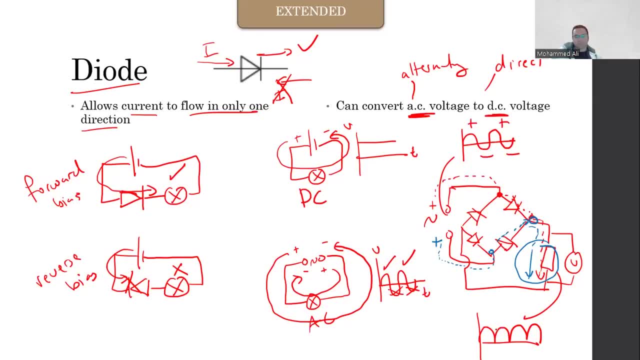 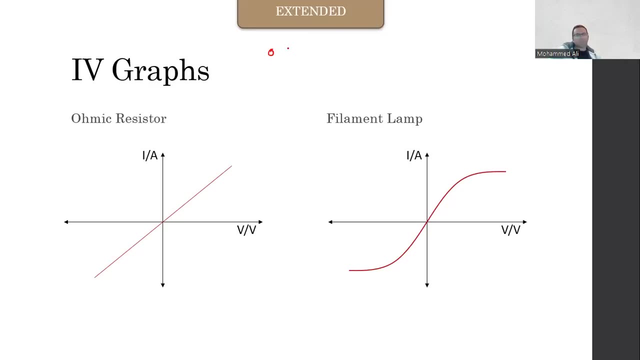 There will be no negative and positive sides of the voltage. It's all the same: Positive, positive, positive Doesn't change, All right. Finally, we have something called IV graphs. This is literally. hey, I'm curious What will happen. 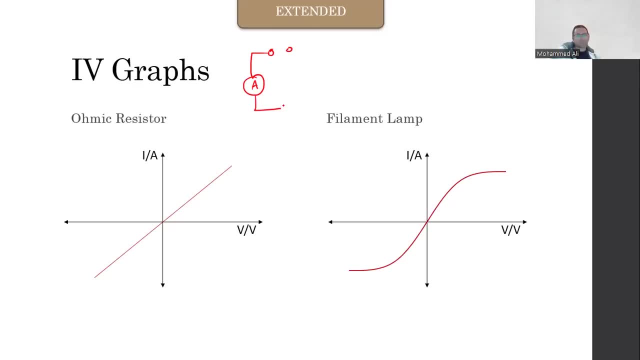 I'm curious What will happen if we put a resistor connected to a voltmeter and an ammeter and we keep changing the supply. When I draw an arrow on something, this means it's variable. So increasing the voltage For a fixed resistor. 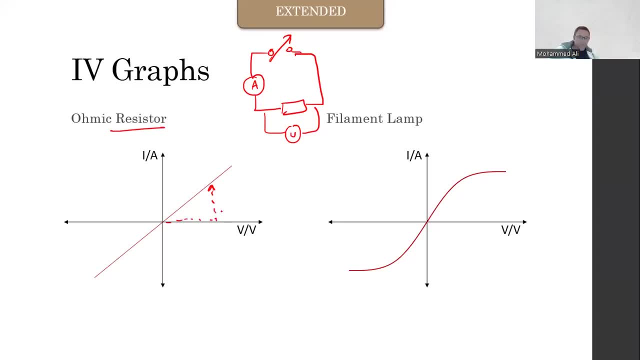 as the voltage increases, the current will also increase constantly. Doesn't change. But for a light bulb this is different. As you increase the voltage, the current also increases, But then it doesn't increase as much. Take a look at this. 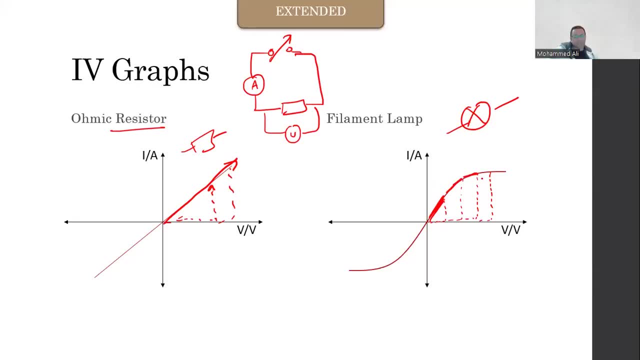 It's increasing a lot here. It's still increasing a lot. It's increased, but a little bit. It's increased a lot less. Why? Because as the voltage on the light bulb increases, the brightness of the light bulb increases, And if the light bulb 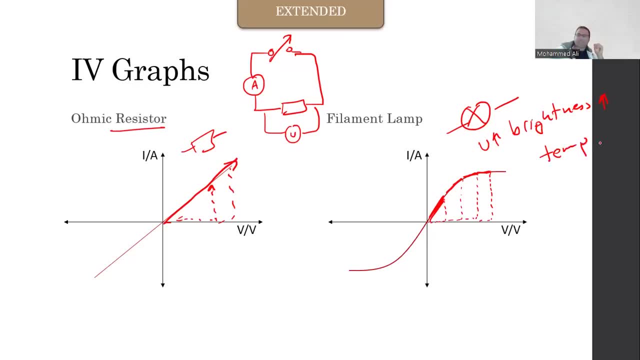 becomes brighter, its temperature increases, It becomes hotter And since filament lamps are made of metallic conductors, as it's getting hotter its resistance increases. So instead of the current increasing as expected, it decreases a bit. It doesn't increase as much as I want it to. 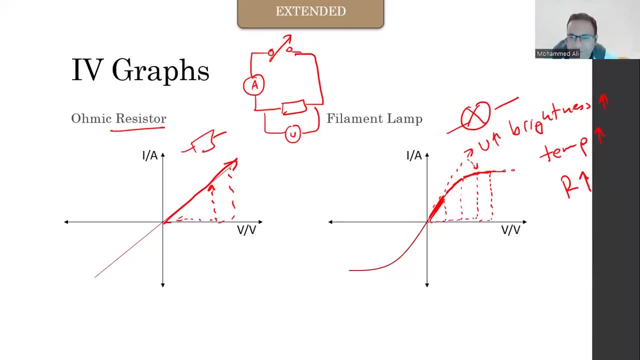 So the reason why the line slopes downward like this is because, as the current increases, as the voltage increases, the brightness of the light bulb increases, making it hotter, and therefore its resistance increases. Right Now, the most important part of circuits 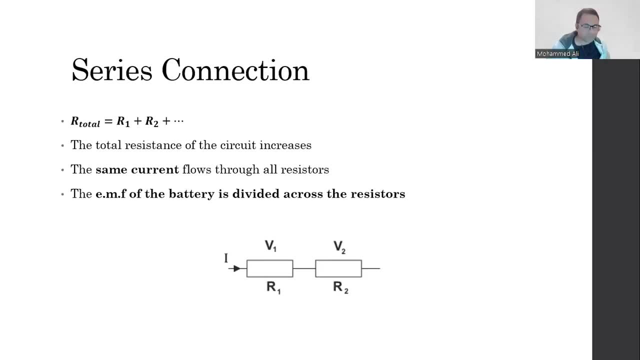 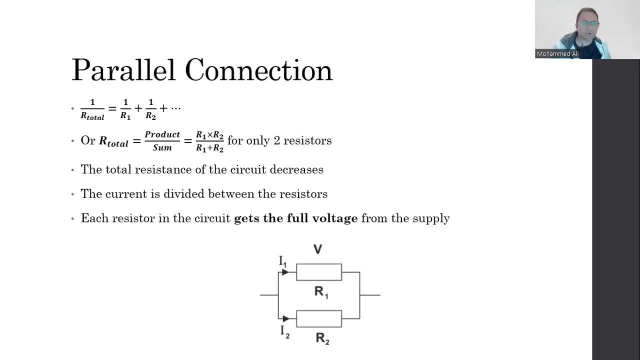 before we end the electricity part, the circuits part, at least, would be series and parallel connections. There are two ways of connecting circuits or multiple components, either in series or in parallel. If you connect resistors in series, the total resistance will increase. 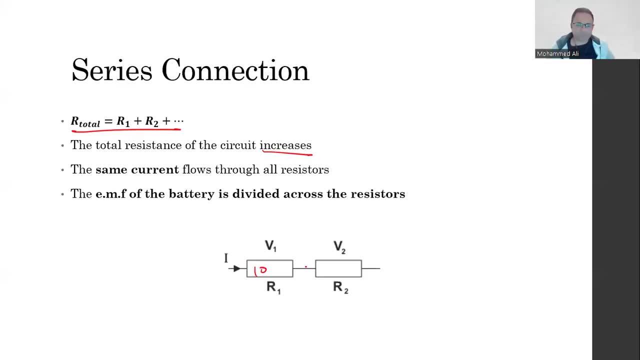 It's calculated using R1 plus R2 plus R3.. So if this is 10 ohms and this is 10 ohms, the total resistance is 20 ohms. for example, 10 plus 10 is 20.. However, 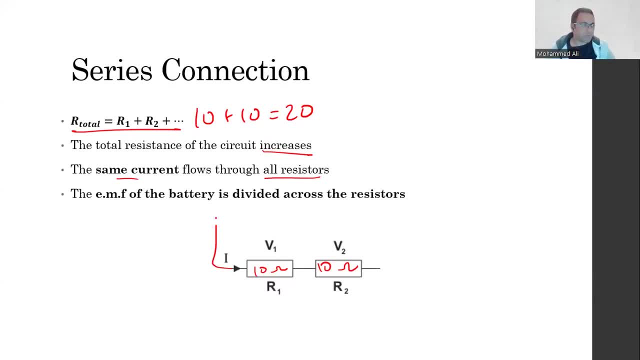 the current is the same because it's the same wire. So if I were to connect, if I were to connect a battery here, like a 5-volt supply here, and I tried to calculate the current, here we go. Let's calculate the current. 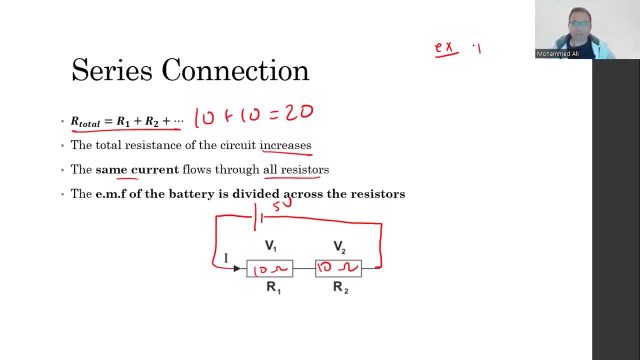 Here's an example right away. The example is: I equals V over R. I want the current. The voltage is 5 volts, The resistance is 20 ohms, So 5 over 20, this should be 0.25.. 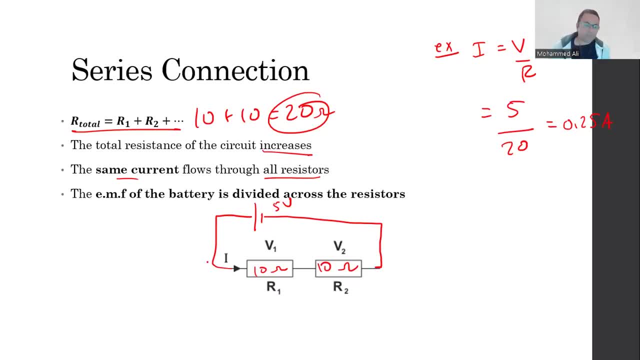 So a quarter of an ampere, Same 0.25 ampere here, here, here, because it's just one wire, However, the voltage of the supply is divided across the resistors, It's split across the resistors And it's always split. 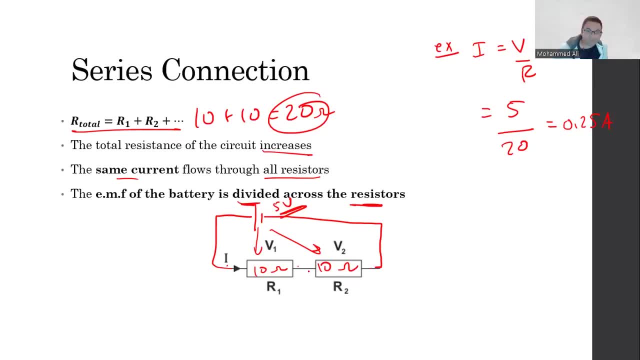 according to the ratio of the resistors. So if these two resistors are equal, the voltage is split across them equally. Try this out: We already got the current flowing through this resistance. Calculate the voltage across R1.. So you're going to say: 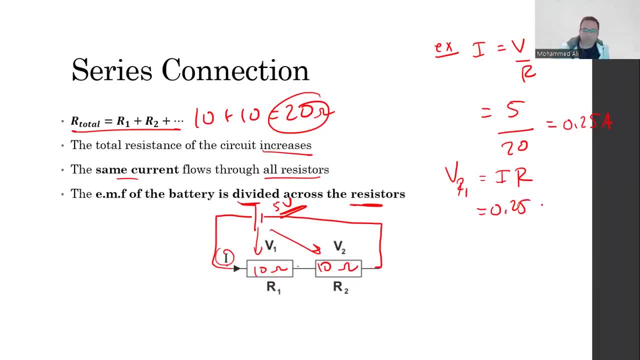 V equals IR Ohm's law. The current is 0.25.. And what resistance do I want you to measure? 10.. Like the voltage across 10.. 0.25 times 10 gives you 2.5 volts. 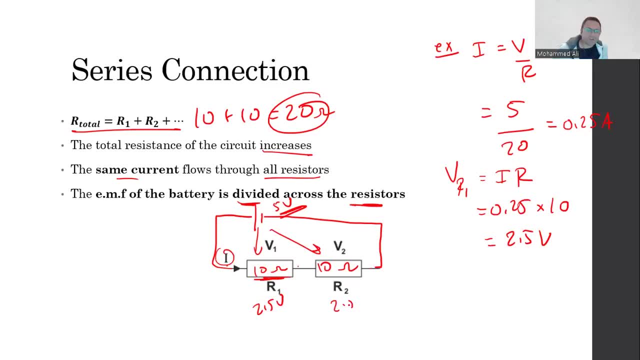 which makes sense, Because if this takes 2.5 volts, this will also take 2.5 volts. It's been split equally Fantastic. All right, Now your gears might be working, but what if the resistors are not equal? 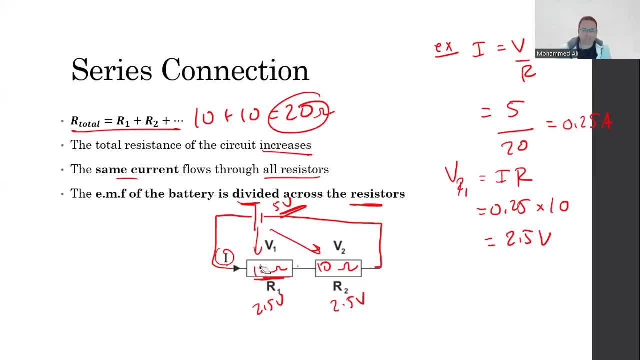 And I would respond by saying that's a really good question. What if they weren't equal? What if, for example, I'll keep the total resistance the same, But what if, for example, this was a 5 ohm resistor and this was a 15 ohm resistor? 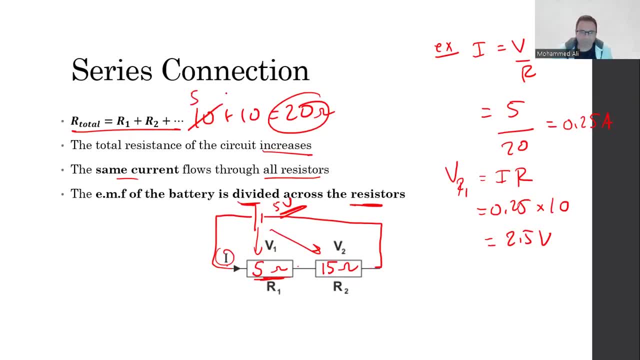 The total resistance is still 20 because you know, 5 plus 15 is still 20.. But will the voltage be split equally? I would say not. This would change. The current is still 0.25.. It hasn't changed. 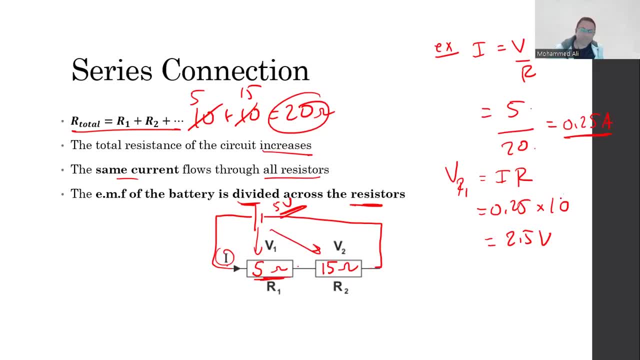 because the voltage is the same, total resistance is the same, But instead of calculating the voltage across the 10 ohm resistor, no, no, no, no, no, I want you to calculate the voltage across this 5 ohm resistor. 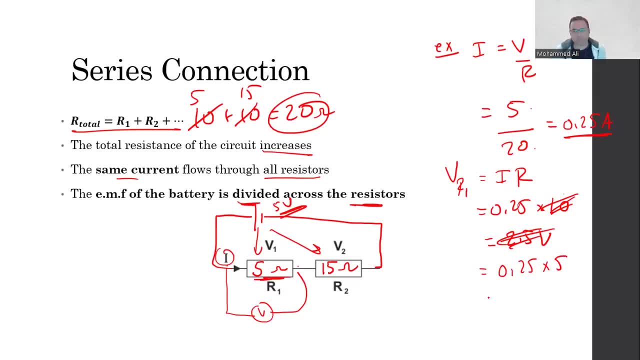 So that's 0.25 times 5, which gives you- come on, I'm sure you know- 1.25.. 0.25 volts: If the first resistor gets 1.25 volts, what will the second resistor get? 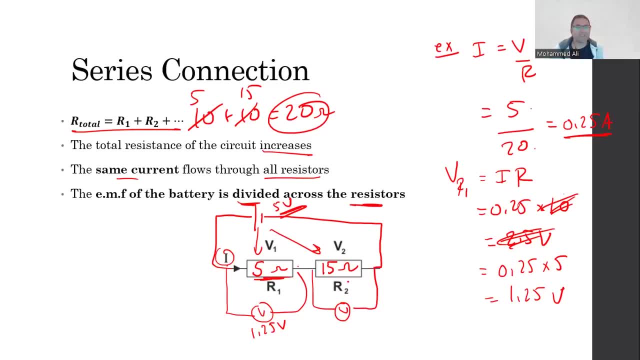 If I have a voltmeter here to measure its voltage, what will it get? The rest? The rest of it 1.25, or sorry, 5 minus 1.25.. This will give you 3.75 volts. 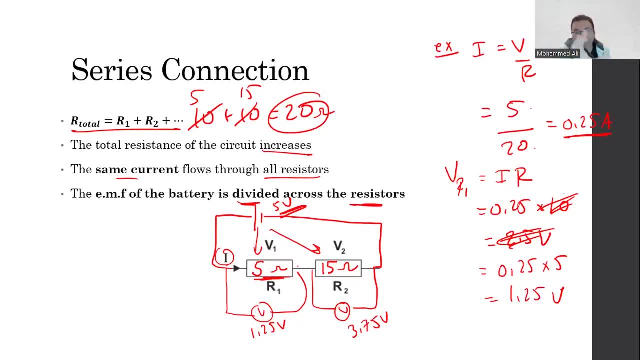 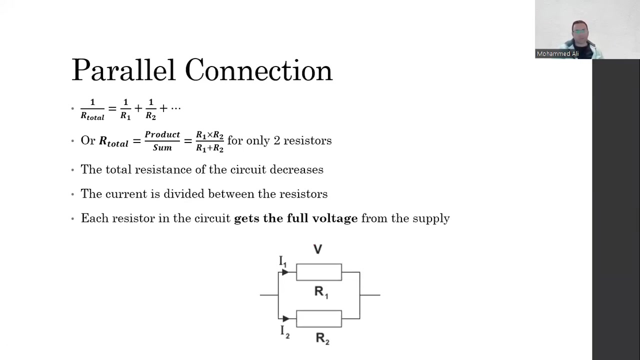 Voltage is not split equally. The bigger resistor gets a bigger portion of the voltage, The smaller resistor gets a smaller portion of the voltage. Very good, That's the series connection. What about parallel? The exact opposite. The total resistance in parallel decreases. 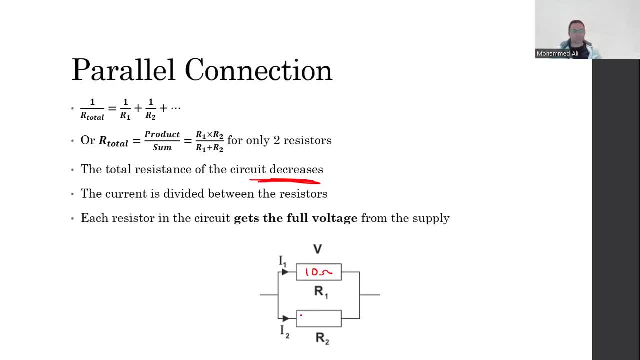 Total resistance decreases when you connect them in parallel. So if you have a 10 ohm resistor and a 10 ohm resistor, the total resistance is not 20.. Instead, we use this formula: 1 over R total equals 1 over R1. 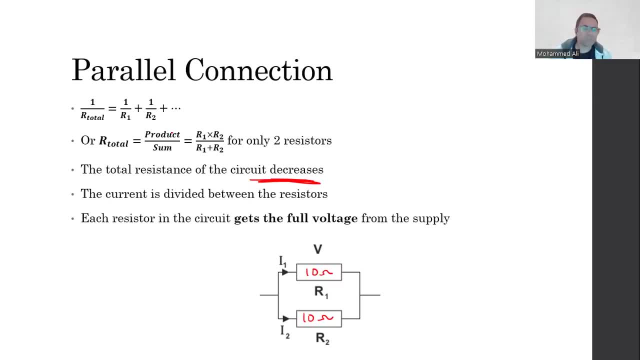 plus 1 over R2 to calculate it. Or we simply say product over sum, So R1 times R2 over R1 plus R2.. And give this a shot. Here's the example: 10 times 10, because I want the total resistance. 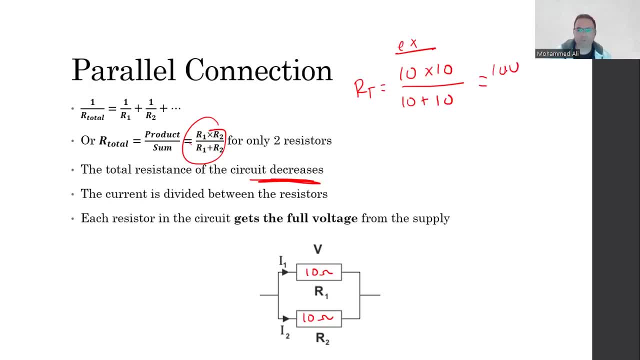 over 10 plus 10.. This gives you 100 over 20, which is 5 ohms. So the combined resistance of the resistors in parallel decreases. It doesn't increase, It decreases. All right, You might say, yeah, that's cool. 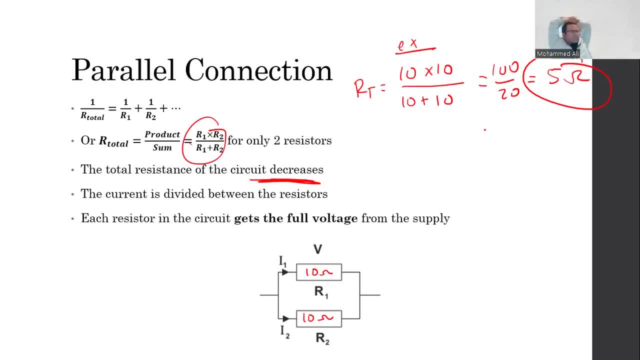 That's great. I need to stretch it. Anyway. That's fine. It's 5 ohms, No biggie. But what happens to the current? If you were to connect them in parallel, you would get this to again a 5 volt supply. 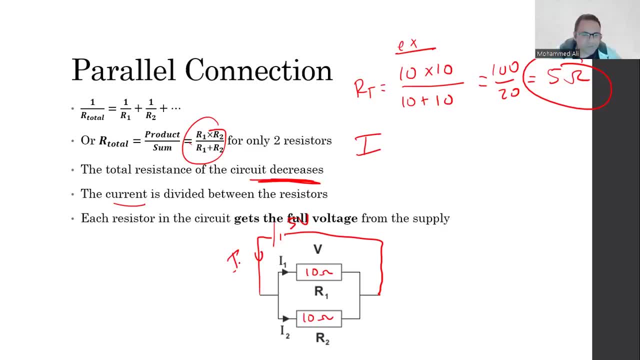 How about calculating the total current? Let's go. What is the total current? I equals V over R. The total voltage is 5 volts. The total resistance is 5 ohms, which gives you a 1 ampere current. But here's the thing. 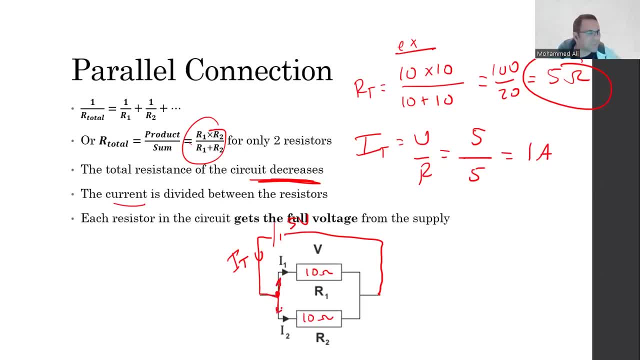 When the current is moving, it reaches a junction And this causes the current to split. some of it goes up, some of it goes down, And when some of it goes up and down, it splits. Does it split equally? Well, if the resistors are equal. 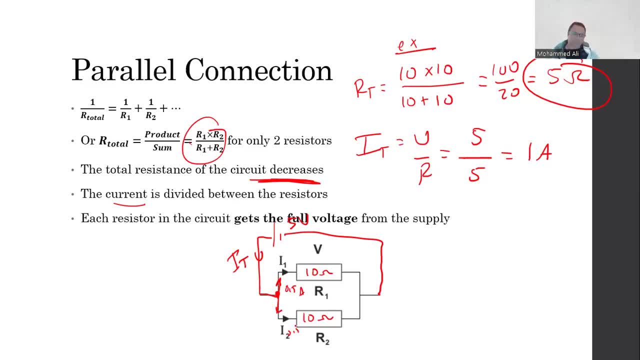 well, yeah, this will get 0.5 ampere. This is going to get 0.5 ampere. You want to check? Let's do this. I1 is going to be V over R1.. This is 5 volts. 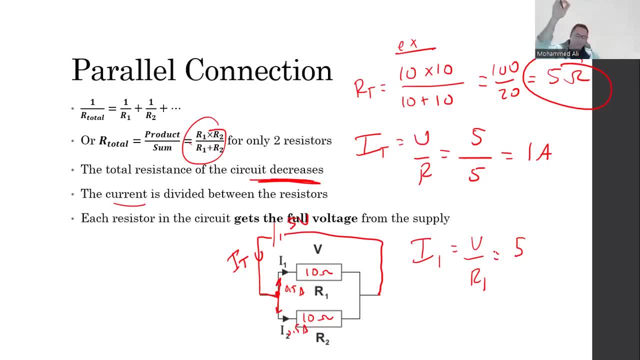 Now, why is it 5 volts? Because the most important thing when it comes to resistors, when it comes to resistors in parallel, is that every single component gets 100% of the voltage from the supply. 100% of the voltage from the supply. 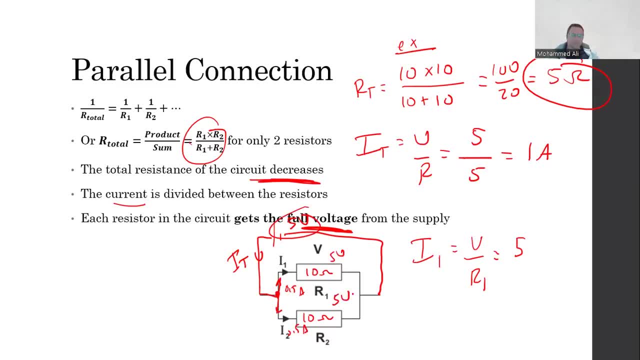 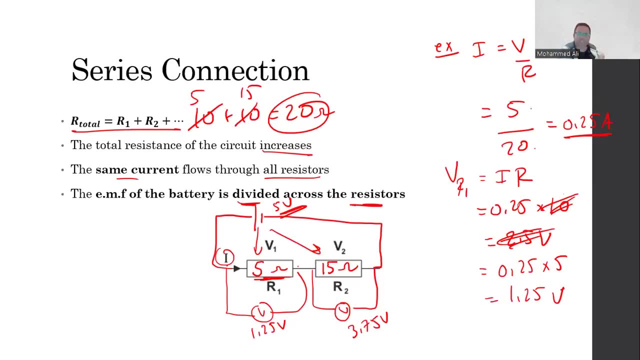 So if the supply is 5 volts, this gets 5 volts. this gets 5 volts because they're not sharing a current. In series they used to share the current. The same power charge has to feed two resistors. Charge is coming here. 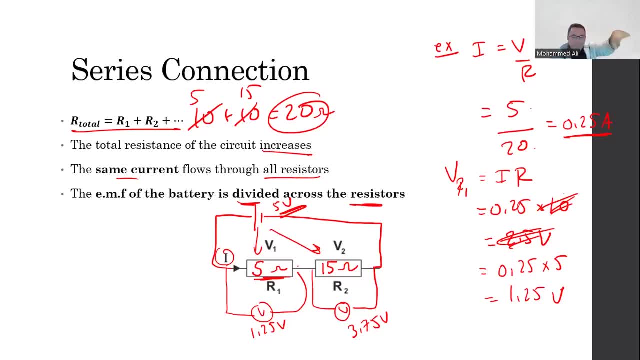 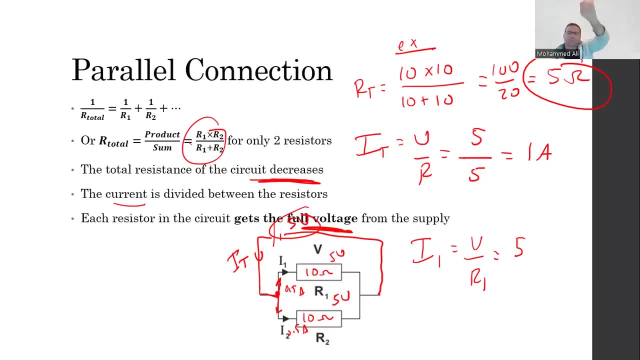 It gives this a few volts and the other one the rest of the volts. but here it's got two charges going through and each one gets its own voltage. So full 5 volts over what's R1? 10.. 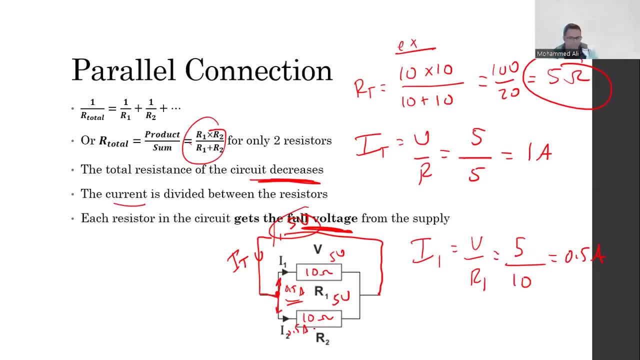 5 over 10 is 0.5 ampere, just like we predicted. You can repeat this with I2.. And obviously, obviously, if the resistors are not equal, the current is not split. equally, you can use I equals V over R. 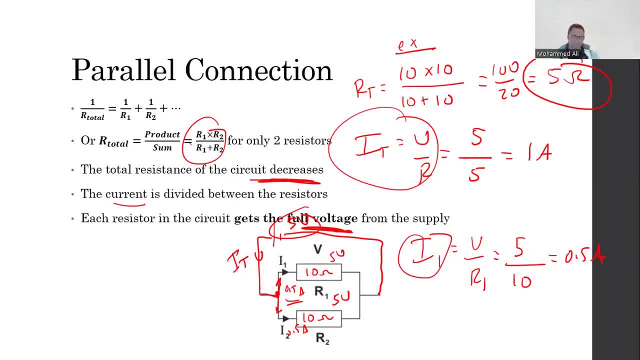 to calculate them? The exact same steps. I see a few questions, So just give me a second. So how is the R5?? I'm not saying in these resistors have become 5 ohms. No, this is still 10,. 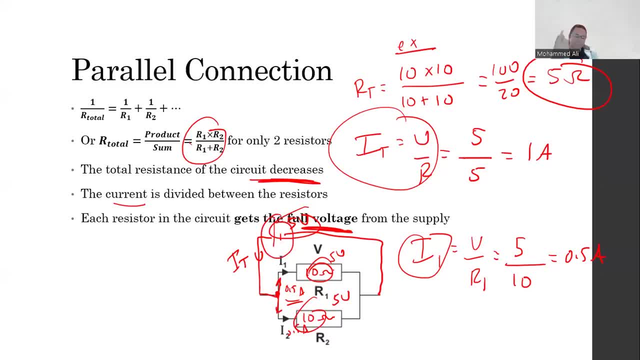 and this is still 10.. But the battery behaves as if there's a 5 ohm resistor in its way. Again, the battery behaves as if there's a 5 ohm resistor in its way, because now the battery has to double the current. 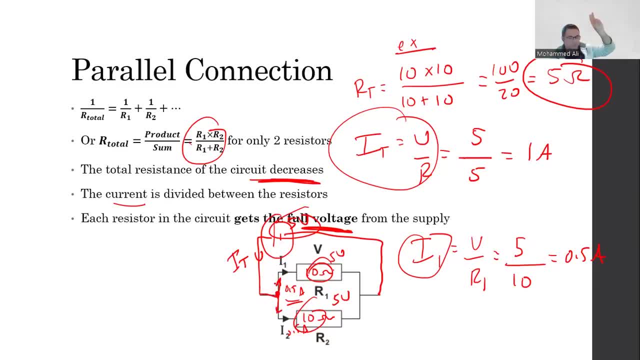 Keep that in mind. The battery has to double the current because you've got some current going here, some current going here, So it has to increase the current that it's feeding to the circuit to account for the split that's going to happen. 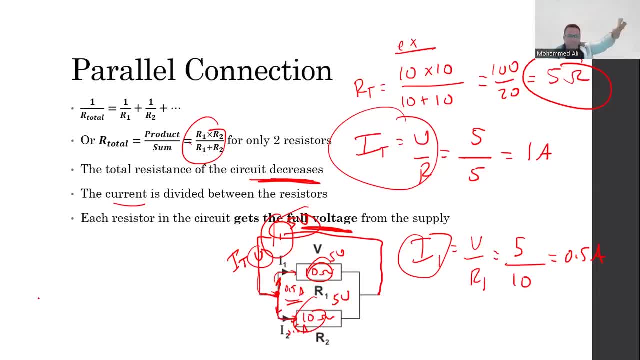 So the total current increases And, as we've studied earlier, if the current in a circuit has increased, this means that the resistance has decreased because the voltage hasn't changed. I hope this is clear. Okay, going back, Will the current eventually decrease? 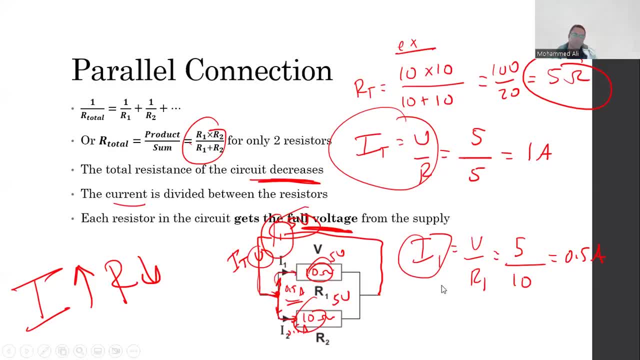 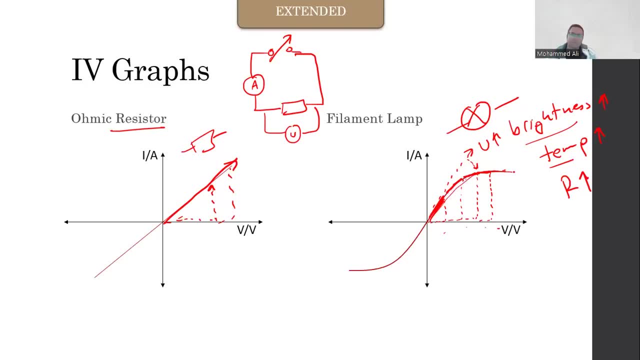 in an IV graph with the voltage increasing. No, it won't. If I were to go back to this IV graph, this will eventually plateau, but it will never decrease, because decreasing the current with an increasing voltage makes no sense. The current still has to increase gradually. 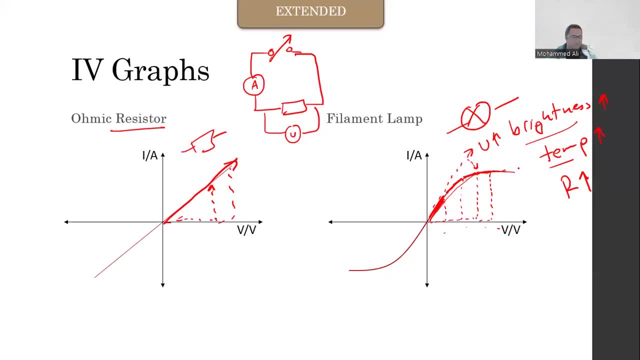 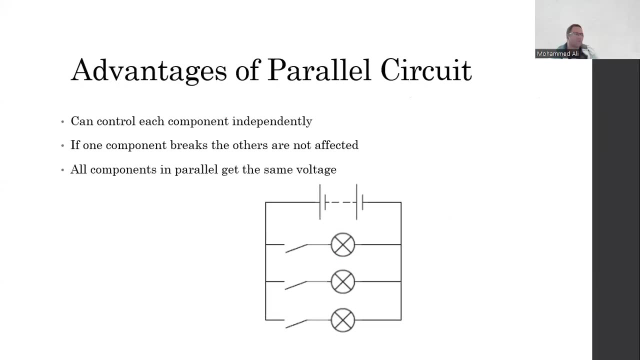 but it won't increase as much. That's the problem. Now, finally, are there any advantages to connecting components in parallel? Absolutely Yeah, of course there are. What are they? Well, you can switch them on and off separately. You can have separate switches. 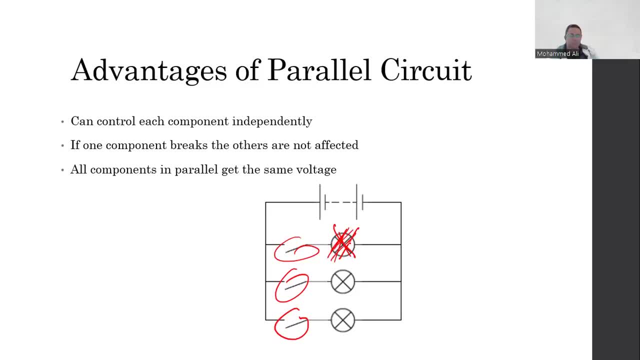 If one of them breaks- if, for example, you shoot a football at this in breaks- then the others won't be affected, It doesn't matter. And finally, most importantly, they all get the full voltage. For example, everything at home. 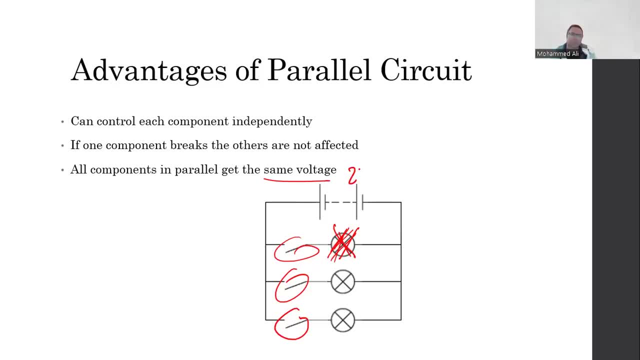 is connected in parallel Everything. Why? Because the voltage at home is about 240 volts, 220, 240.. Each light bulb gets the full voltage, which is amazing and brilliant. Why? Because imagine if you wanted to increase the number of light bulbs at home. 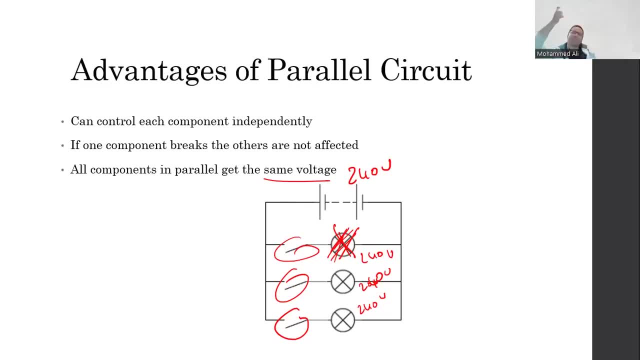 and they're connected in series. When you add one more, you don't get more light, you get less light, because each light bulb now gets less voltage. Eventually, as you add more and more light bulbs, the light bulbs won't light up. 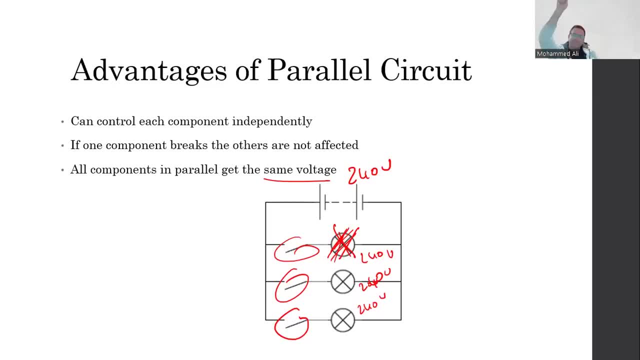 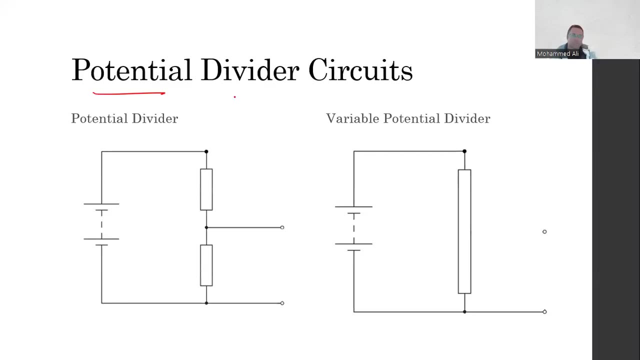 if they were in series, But if they're in parallel, everything gets the same voltage: full, 100% voltage from the supply. Very good, Okay. Finally, what about the potential divider? What is this? Take a deep breath, Look at the diagram. 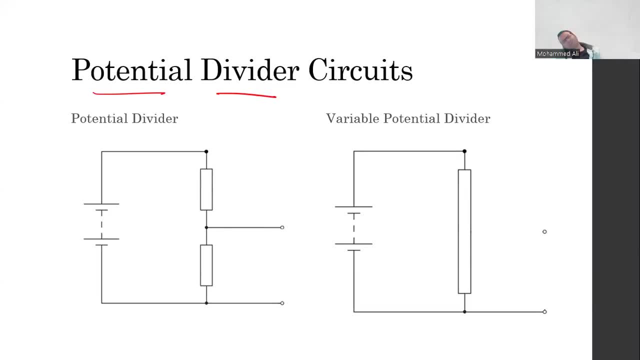 Look at the side this way, for example, and you go like: oh mister, why are you being like sneaky? Do you think you're clever? Do you think I'm? do I think I'm clever? This is just two resistors in series. 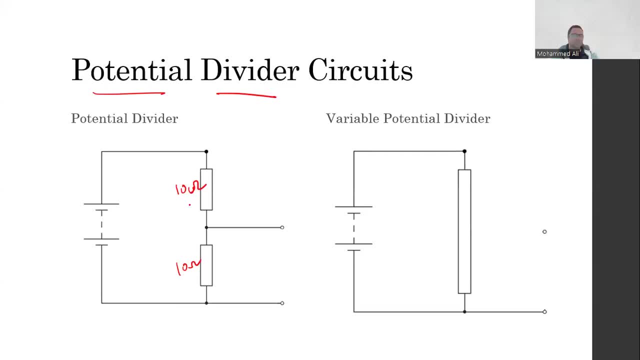 What game are you playing? Well, I'm clearly not playing League of Legends, but what game? what game are you playing? Well, here's the thing. Here's the thing. This is why we're gonna call it a potential divider. 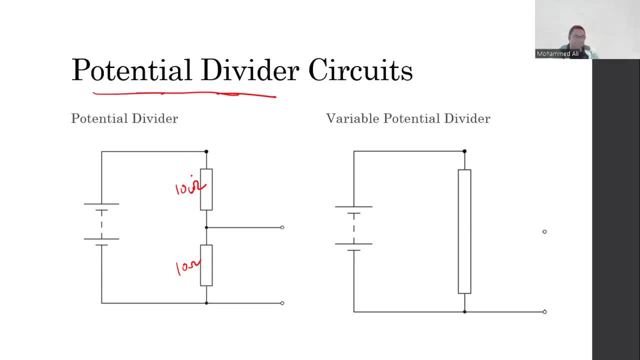 This is why we're gonna call it a potential divider, And we'll see the difference between it and a variable resistor. If this is a 10 volt supply, what's the total voltage here? 10 volts, This will get five volts. 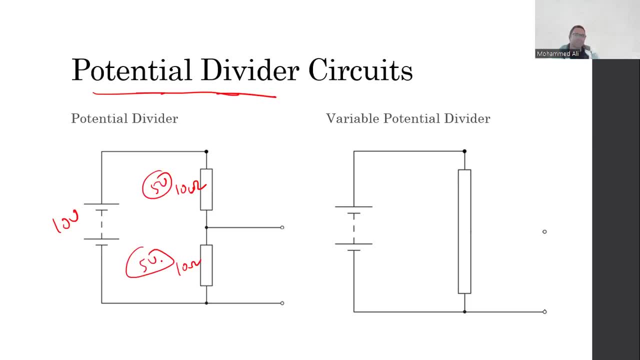 This will get five volts, You. you go ahead and say: hey, mister, the voltage is in series, That's fine, It splits. But here's where the fun comes in If I add another light bulb in parallel only to the first. 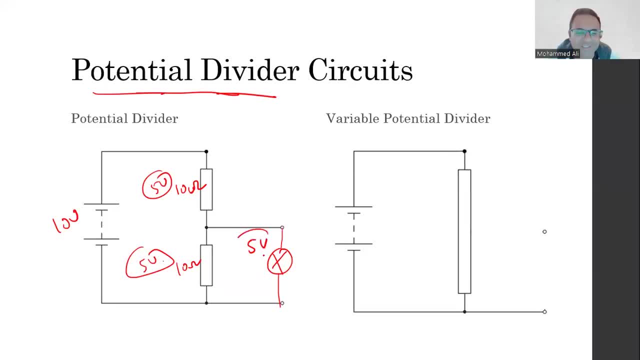 what's the voltage that it will get? Because parallel components all get the same voltage as each other, But since the light bulb is parallel to only one resistor, not the entire circuit, it's not this. It only gets as much voltage as the parts parallel to. 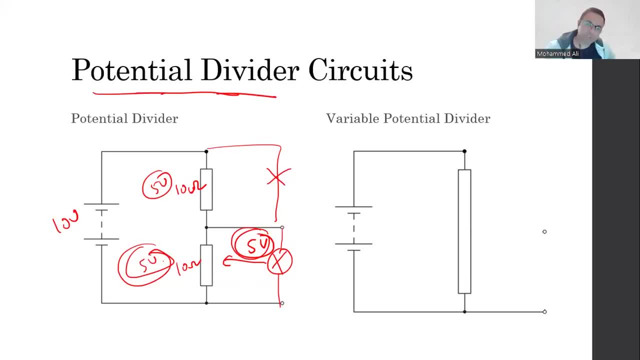 which is exactly what we want, Because sometimes I don't want to control the current. I want to control the exact voltage across a light bulb, for example, and I want to be able to increase it and decrease it In the first case. 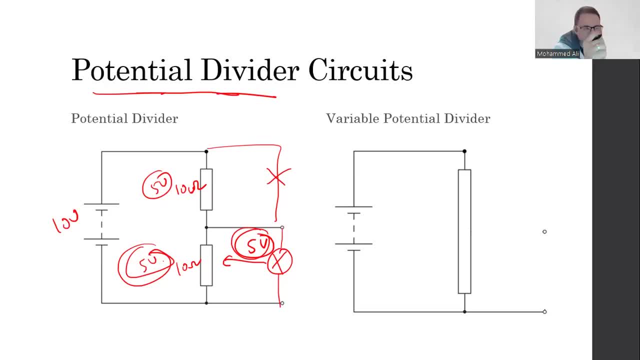 the simple potential divider. you only have two resistors to do that. You could have one of them be a thermistor or an LDR. So now you make this light bulb sensitive to heat or light, Or you could use a variable potential divider. 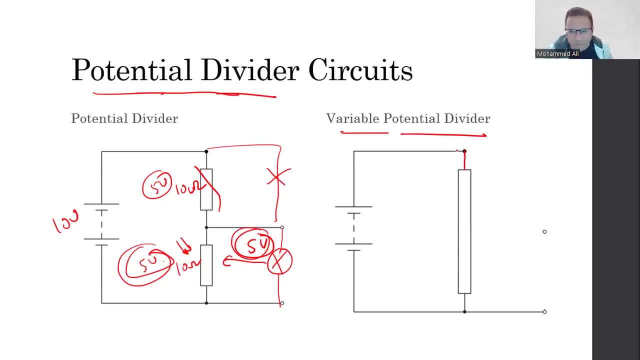 This is like a variable resistor, but you'll notice that both of the ends are connected to the battery. So this is a 10 volt supply and the entire wire gets 10 volts. The trick here comes from where we attach the sliding contact. 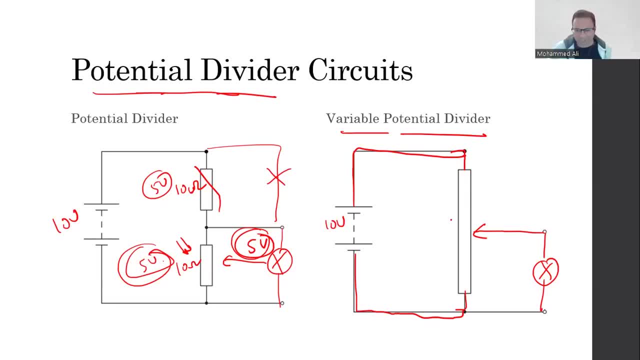 When we connect the sliding contact in parallel, not in series, in a variable resistor. it was this way. It was in series because it came directly from the battery. It's not what I want And I put the sliding contact in the middle. 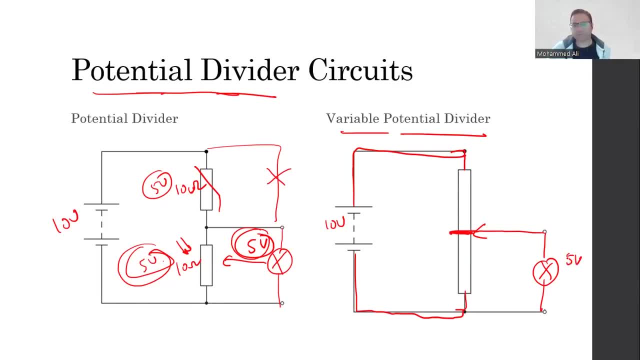 The voltage across the light bulb here is going to be 5 volts. It'll literally be half the voltage. If you move the sliding contact up here, the voltage will be- I don't know- 8 volts. It's 80% of the voltage. 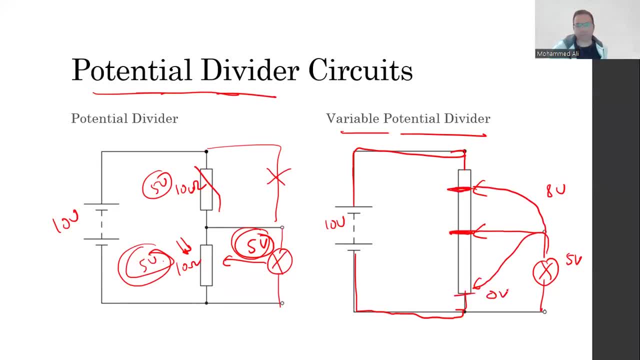 If you put your sliding contact down here, it gets nothing- Zero volts, Because it's parallel to nothing. So the idea here is what By changing where the sliding contact is, you don't change the total resistance of the wire, You change what portion of the wire. 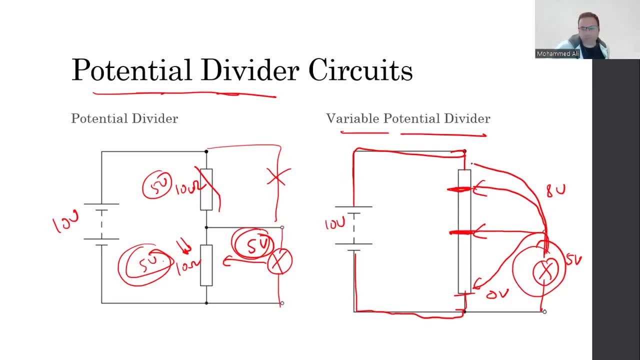 is the light bulb parallel to. If the light bulb is parallel to the whole wire, that's 10 volts. If it's parallel to the beginning of the wire only, that's zero volts. If it's parallel to the center of the wire, 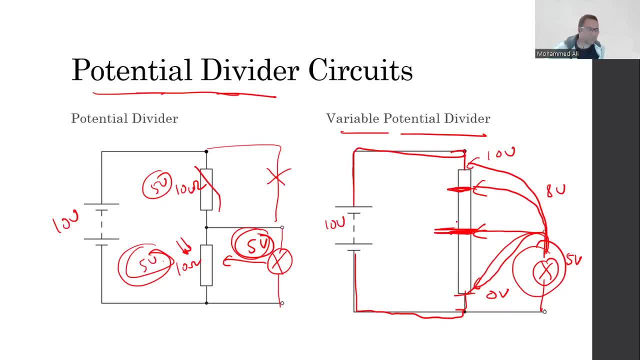 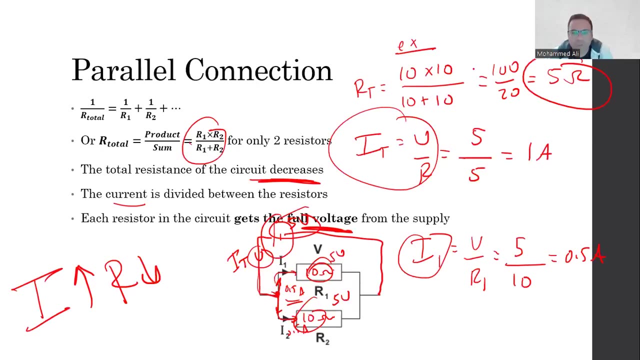 I'm sure you know what that is. Five volts. So a variable potential divider's purpose is to control the voltage across a component, Whereas the function of- I'm just going back a bit- the function of a variable resistor which just changes the resistance. 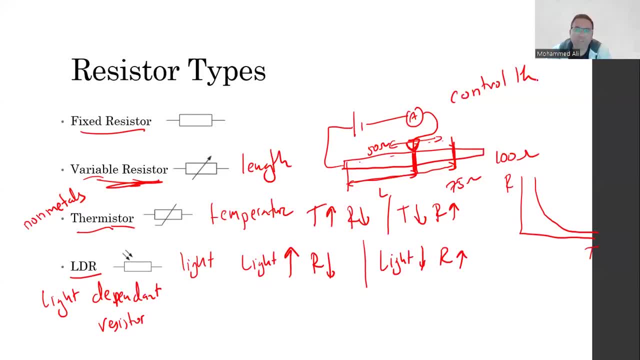 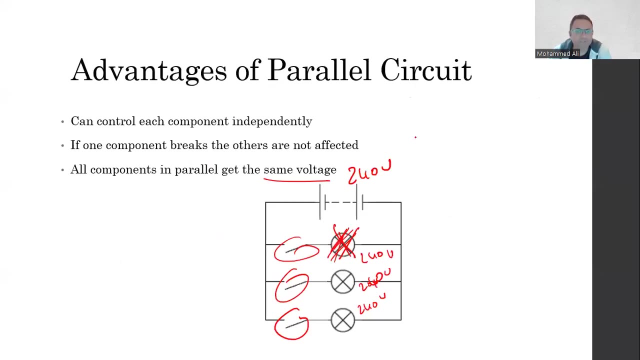 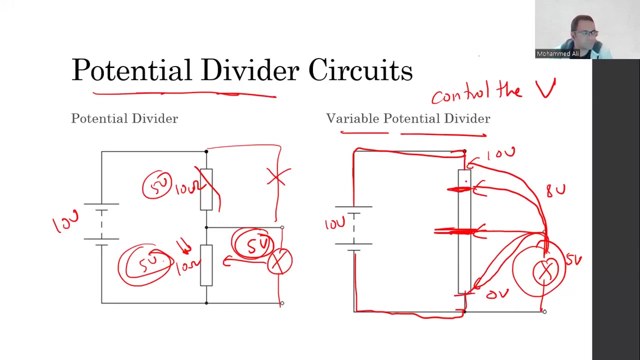 is to control the current in a circuit Because it's often connected in series. Like the variable resistor is connected in series with the rest of the components, A potential divider is connected in parallel to the resistor wire. All right, Okay, So again, just really quickly. 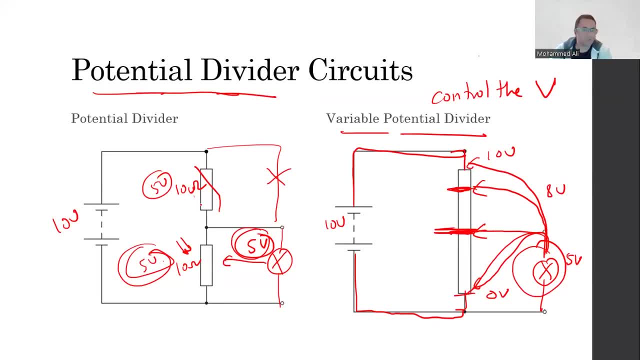 because we need to finish up magnetism as well. today, Potential divider just splits the voltage between the two resistors here And depending on what you connect in parallel, you get the same voltage as the parallel portion only, And the only parallel part is what you get. 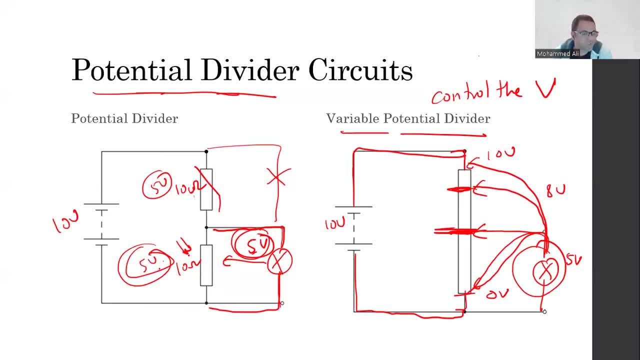 Like the area, the just components you're parallel to, that's the voltage that you get. So, for example, if I change this distribution, if these aren't equal anymore and this gets eight volts and this gets two volts, can you tell me what the voltage? 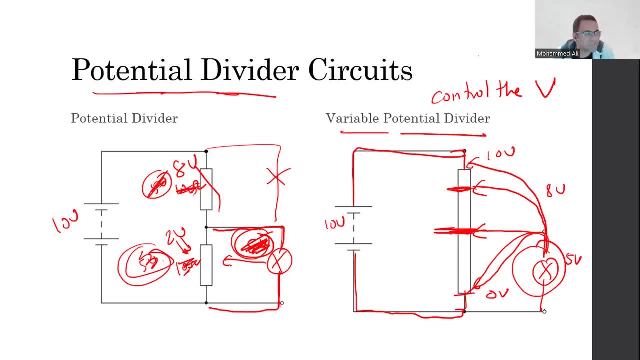 across this light bulb will be, Since it's parallel to the bottom resistor. what's the voltage here? Can you tell me Exactly? Perfect, Two volts, And that's why we use a potential divider, But instead of using fixed resistors. 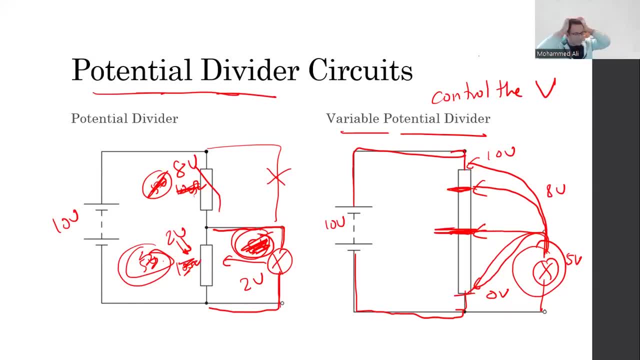 because the problem with a potential divider is like: hey, I want to change the voltage. Now what do I do? Remove the old one, put in a new one. No, that's not what I want. Remove the old one, put the new one. 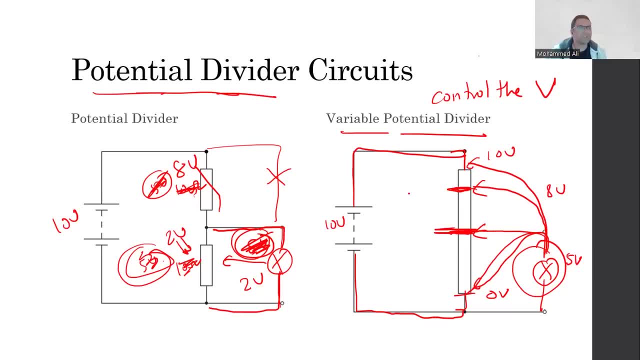 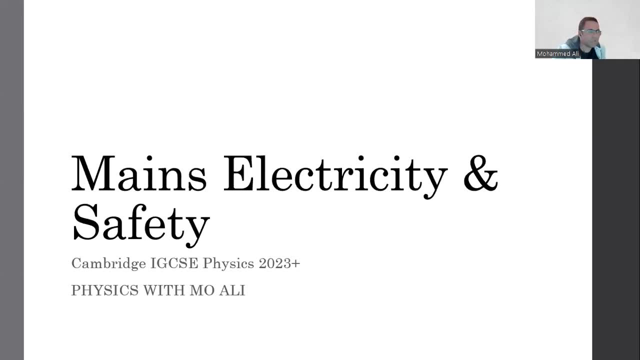 Or you can just slide this contact up and down and just immediately control the voltage. All right, Last part of electricity. Let's talk about safety: electrical safety and electricity at home. It's used in a dimmer switch. Exactly This is used in a dimmer switch. 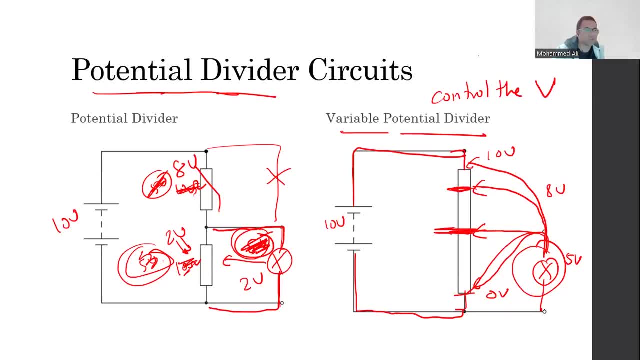 It does not control the current. We said it controls the voltage. All right, Just to be clear. we said it controls the voltage, not the current, because things that are parallel to each other get the same voltage, So you're connected in parallel to something that has. 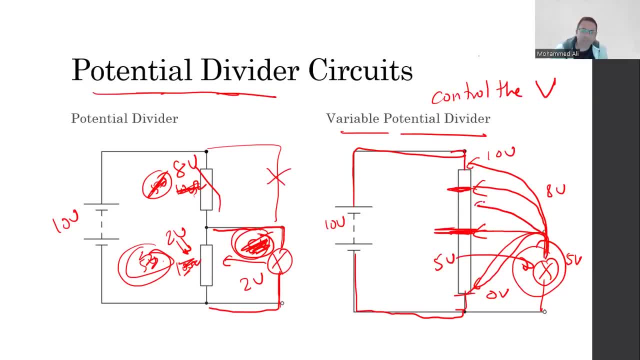 I don't know. five volts, So you get five volts. It's parallel to six volts, So it gets six volts. It's parallel to 10 volts, So it gets 10 volts. So by changing where it's parallel to or what it's parallel to, 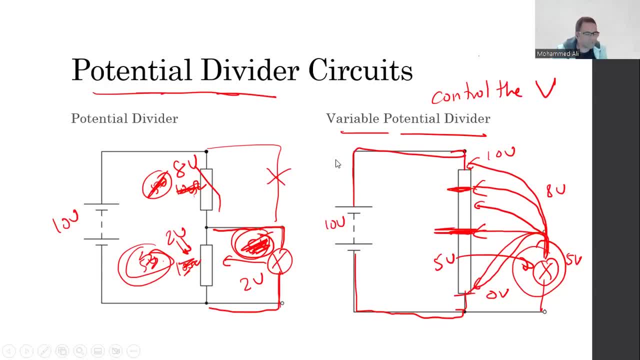 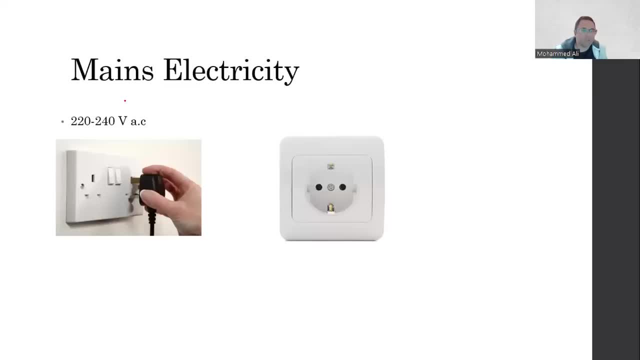 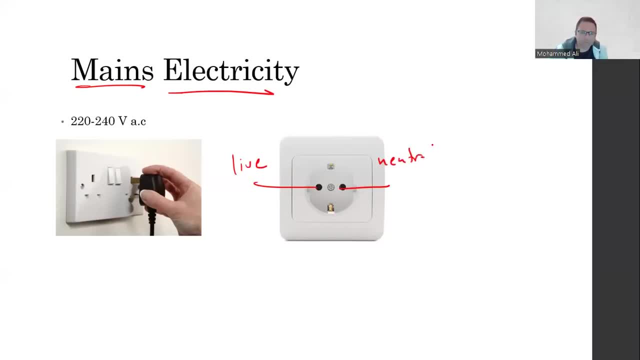 it's quite simple. Any socket has two wires that are very important: one that we call the live wire, one that we call the neutral wire. The live wire and the neutral wire Because the voltage at home is always around 240 volts ac. 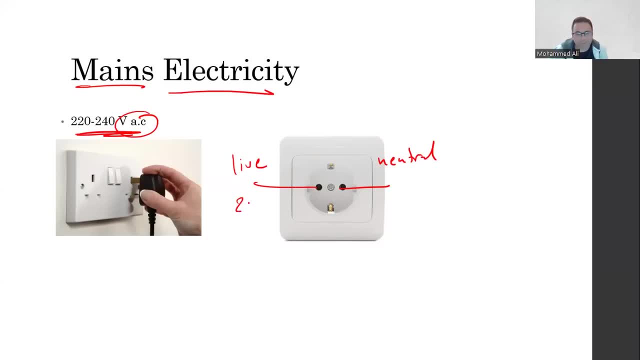 So we don't need a positive and negative supply. The difference between the live and the neutral- 40 volts AC, and the neutral is always at zero volts. So if I were to plug in a socket- something like my PC's socket, for example- plug I mean. 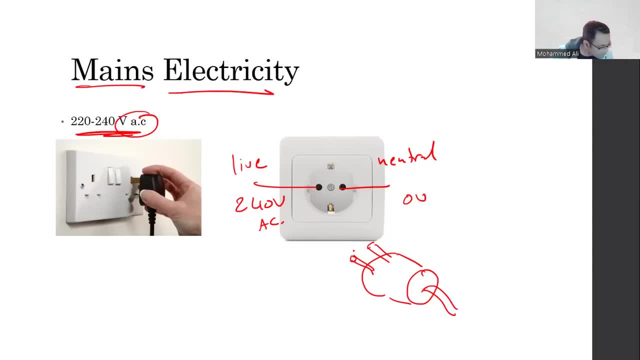 and I plug it in. So we connect this here, we connect this here. So the current goes in through this and then out through this. That's the point of this. live and neutral. Okay, Good, Now two safety features at home. 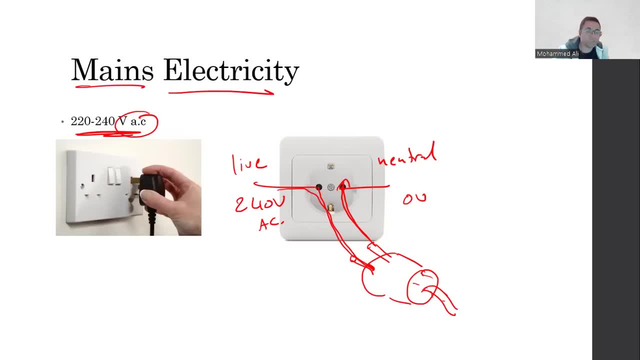 very important three safety features at home. Because you need a. oh, there's a question here. Why do we need to get the current out? Because you need a closed circuit. If this goes and connects to a light bulb, you need a current to go in to the light bulb. 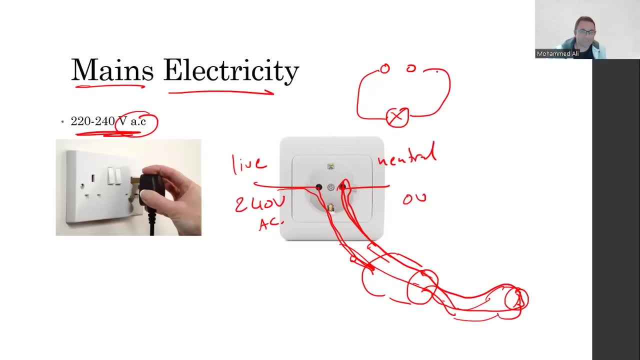 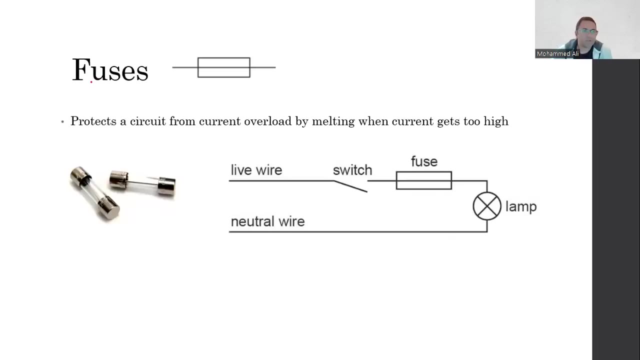 and back out so it can charge again. If the circuit is open, like you, have only one part of it that's connected, it won't work. Okay, Okay, Oops. The fuse is a component that protects the circuit from an overload. 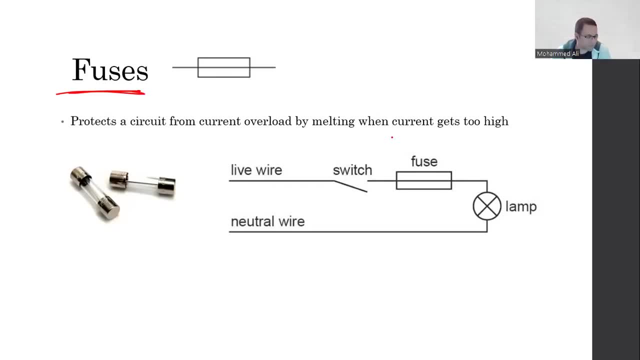 So if the current is too high, if the current is too high, if the current is too high, the lamp is going to a blow out. It's just gonna burn out. If the current is too low, that's fine. So how do you protect light bulbs? 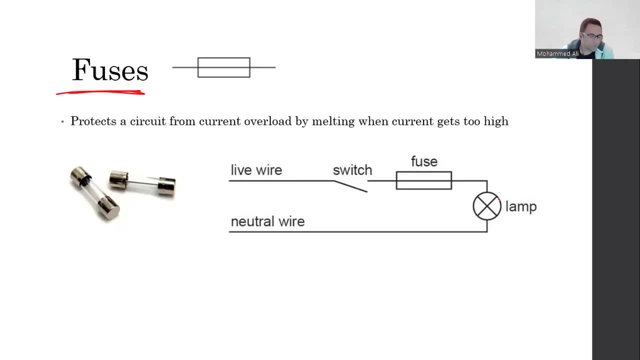 or other components from getting burnt out or, like you know, not working By using a fuse. A fuse is simply a very thin wire like this And it has a certain rating, Let's say 10 amperes. This means if the current going through this fuse 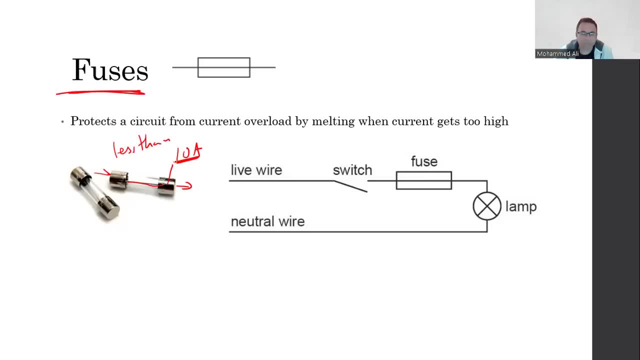 is less than 10,, no problem, But if it's more than 10, this fuse melts, just burns, explodes right that instant. Why? So it stops the current from reaching your lamp or reaching your device and burning it to the ground. 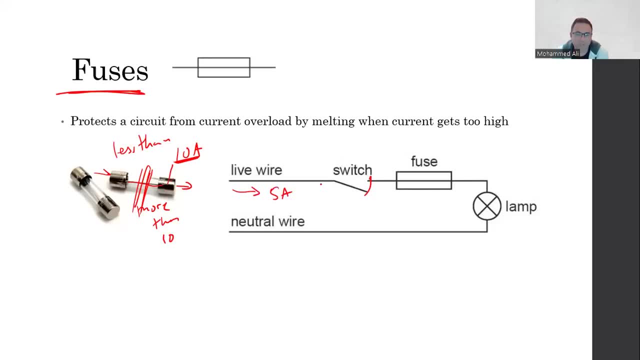 So when you close the switch and the current going through is, let's say, five ampere, and this is a 10 ampere fuse, yeah, it'll just go through no problem. Lights up your lamp, no big deal. But if the current is 15 ampere, 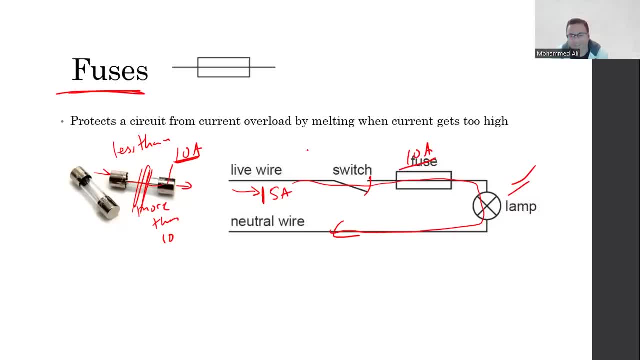 or even if it's exactly 10, or even if it's exactly 10,, it will burn the fuse, which completely stops the current from reaching the lamp. Now you might think it's counterintuitive, like: why do I stop the current? 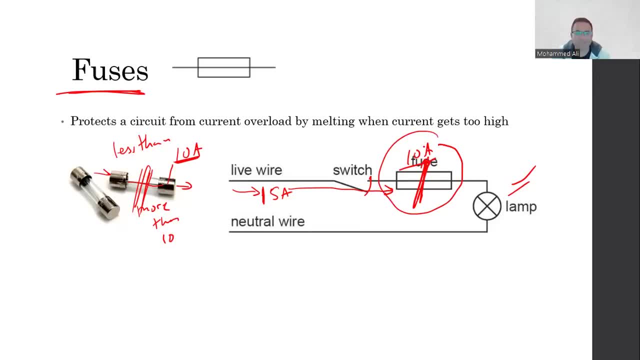 This is ruined now. but a fuse is easily replaced. You can just remove the old fuse, throw it away, put in a new fuse and you're all good. Put in a new fuse and you're all good. So again, the purpose of the fuse. 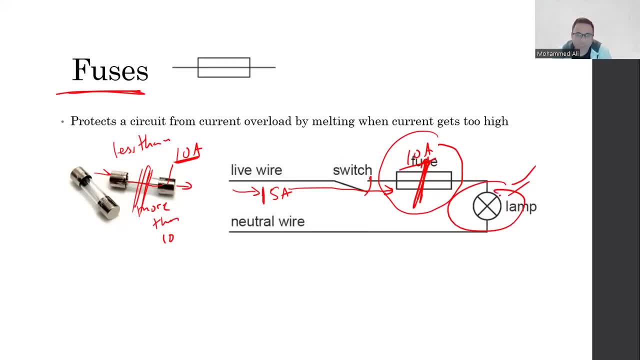 is to protect your devices or circuits from a current overload by melting. Why? Because if the current gets too high, it will completely melt. Okay, Okay, Ahora vamos a tentar. Okay, vamos a intentar. ¿Qué pasa con el circuito de ruedas? 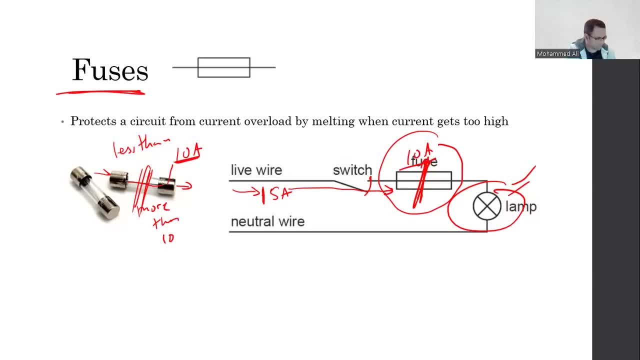 Yo tengo un circuito de ruedas muy pequeño. Puedes ver que su circuito se aburrió, pero está muy caro. No puedo ver nada. El circuito de ruedas es muy grande, Está muy grande. 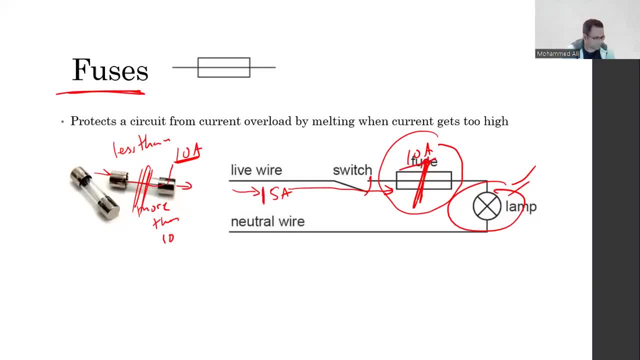 Ahora vamos a despejar el circuito a otro lado. y vamos a despejar a otro lado. ¿Qué pasa con el circuito de ruedas? Okay, Ahora vamos a despejar el circuito a otro lado. 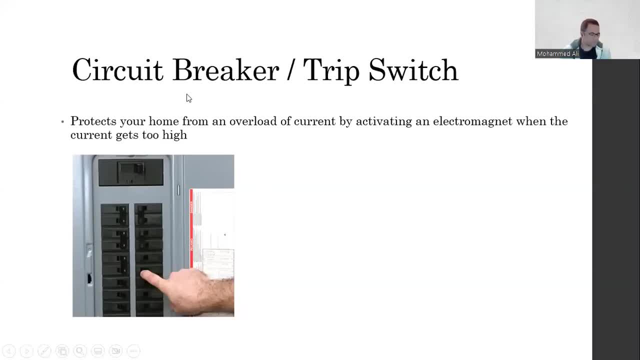 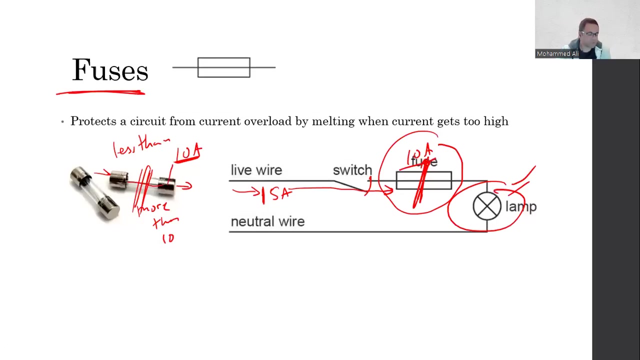 ¿Qué pasa con el circuito de ruedas? circuit breaker protects your home from an overload of current. by what exactly? by using an electromagnet. when the current gets to a high, okay, when it a gets too high, how does that work? exactly like a fuse. it stops the current from getting too high and reaching 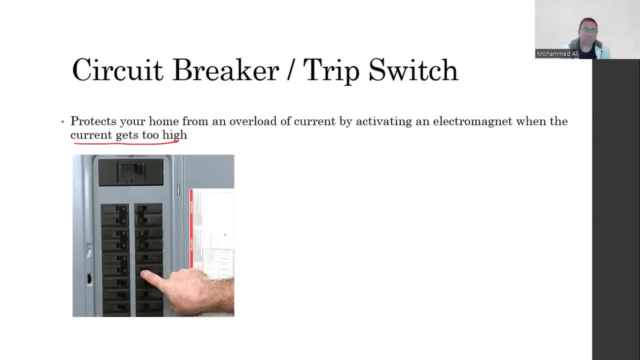 your house. now, how does that work back? uh, here we go first, here's the live wire, here's the neutral, here's a switch, and actually i shouldn't draw the switch upwards, so it's better if we draw it down. and here's your house, or your circuit. 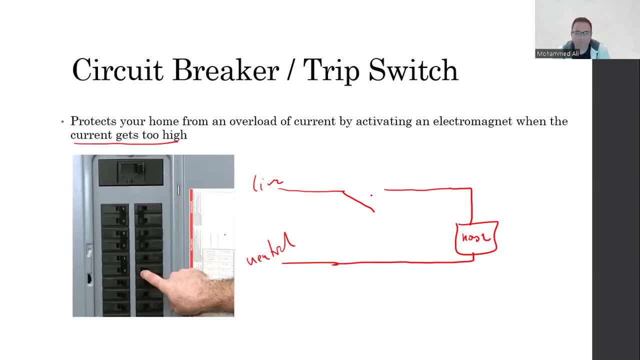 and here's a magnet, okay, an electromagnet okay. and here's your house or your circuit. when the current goes through the live wire and the switch is, you know, closed and it's fine, like right now, the switch is closed, it's no problem, it reaches your house, no big deal. but if the current 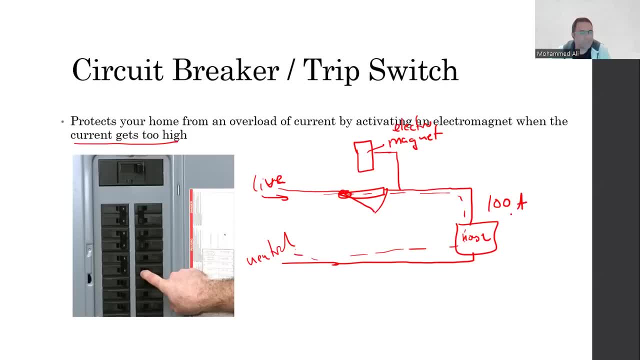 going into your house is too high. let's say your house can only handle 100 ampere. and then the current, and the current is 80 ampere, that's not a problem. but if it's 180 ampere, what happens is that it passes through the magnet. first the electromagnet, first this electromagnet. 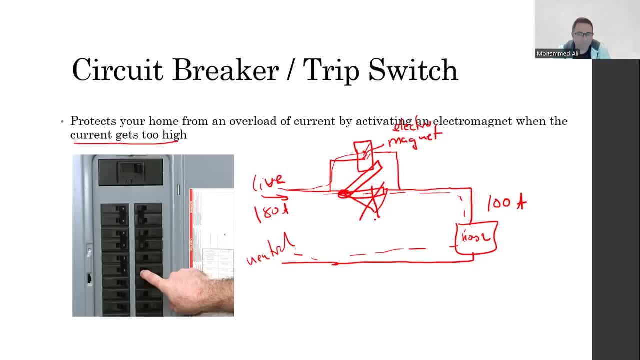 attracts the switch and opens it, so it stops your current from going through. so you see these switches: inside there's an electromagnet, a coil and an iron switch. so when the current gets too high for your house to handle, instead of letting the current get into your house, instead it opens. 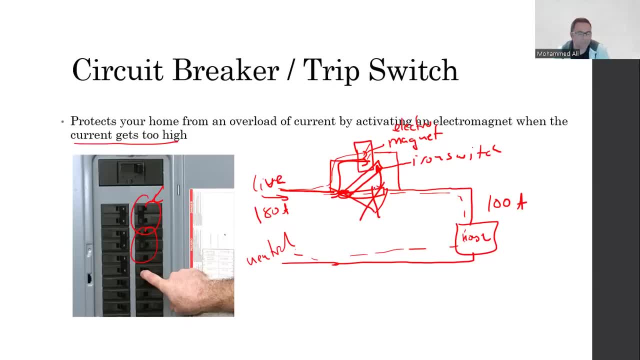 the switch for you and it stops the current from getting into your house completely, however. however, if you want to turn your electricity back on- unlike if you use- you don't have to replace it and just go and flip the switch back up again. so you close the switch again. electricity turns on, if there's anything. 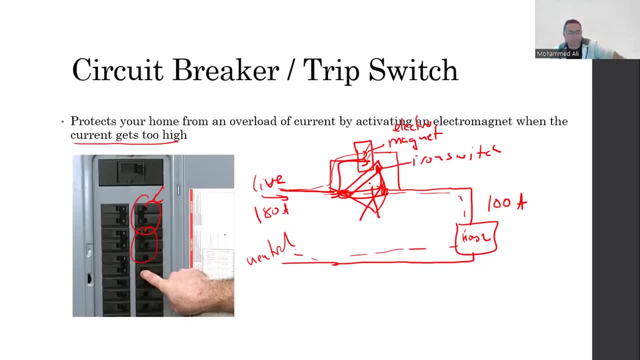 wrong in your house. maybe there's a faulty lamp, maybe there's a faulty socket, anything that happens, maybe there's an electrical surge and the current rises too high, this is what's going to happen: switch is going to open, click and then it's off. your house will not get that current anymore, but you're safe. at least you're not going to be set. 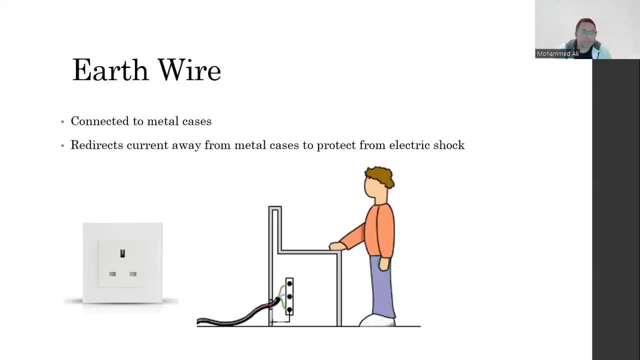 on fire. finally, the earth wire. the earth wire is this. now we already said, we have a live and a neutral wire, and then they have a third wire called the earth or the ground wire. the earth or the ground wire. what we do is, if a device has a metal case, think, uh, i don't know a. 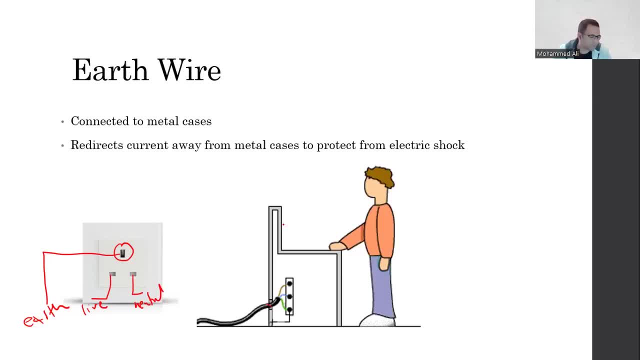 washing machine, then can a fridge, your pc, for example. we connect the case itself to this earth. so if, for any reason, one of your live wires touches the case, the electricity flows through the case and through the wire and it goes out through the earth and it's 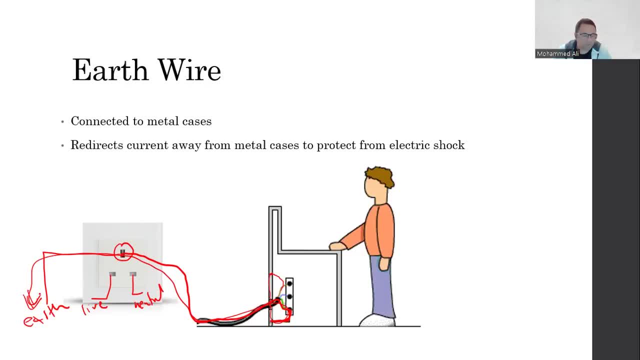 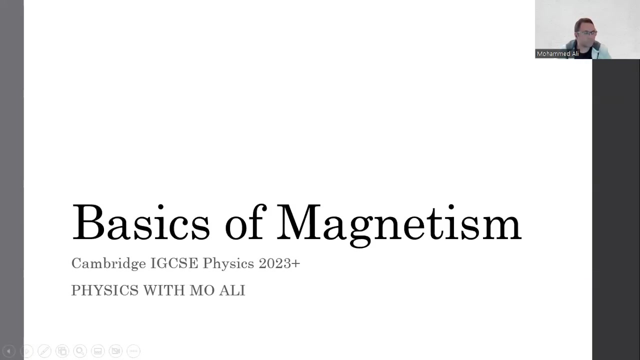 goes out through the earth, which completely cuts off the electricity, like it saves you from getting electrically shocked. so the way it works is that it redirects the current away from metal cases to protect you from getting electrically shocked. that's all. yeah, let's talk about magnetism. 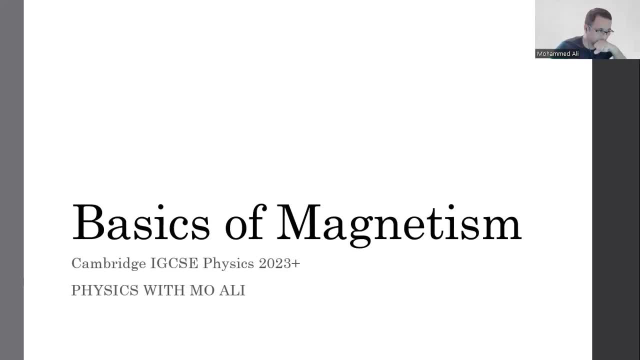 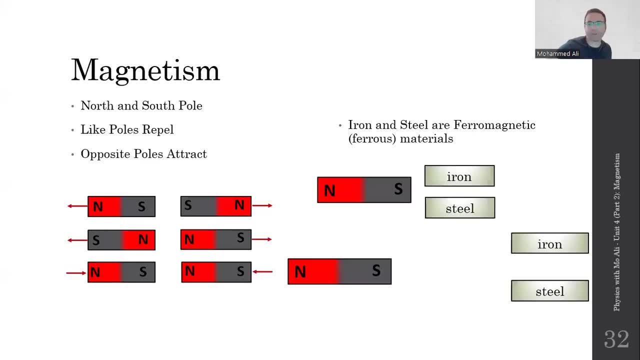 we're done with electricity, all of it. let's talk about magnetism now. you all are familiar with a magnet. a magnet has a north pole and a south pole and it attracts and repels, just like electric charges. the concept is the same: like poles repel, 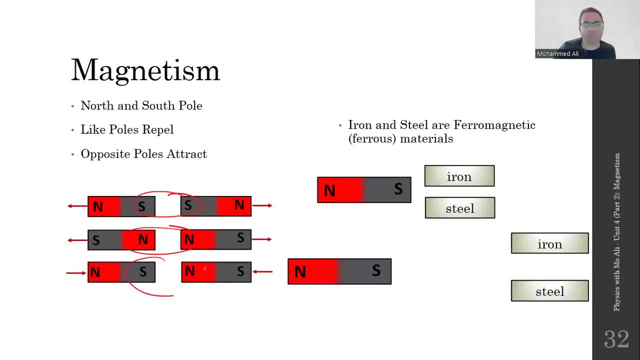 so south and south repel, north and south repel. opposite poles attract. north and south attract. but just like electricity charges can attract neutral objects, here magnets can attract certain metals. now there there's a lot more than just these two, but for now iron and steel are the two ferrous or ferromagnetic materials that 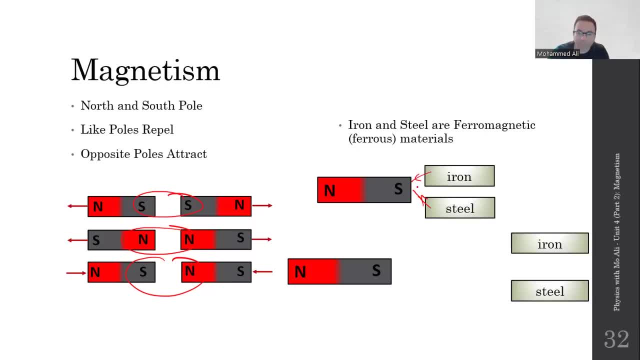 are attracted to a magnet. the way it gets attracted is by magnetization. they become magnetized. so bring them close to a magnet. it has or becomes magnetized and it becomes a magnet within its own north and south poles and it always attracts. so if this is the south pole, this becomes north. 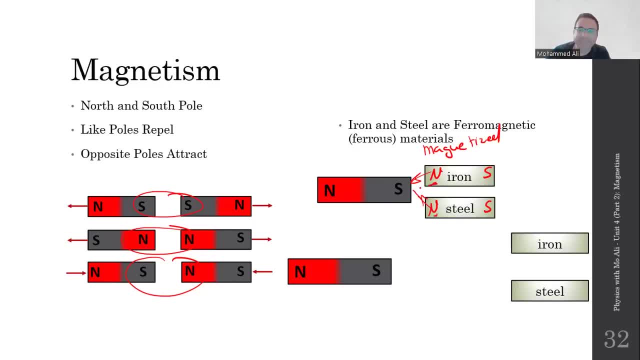 if this was the north pole, this would become south. and then it sticks to the magnet. so magnetization happens first and then it gets attracted. but if you were to remove the iron and steel from that magnet, after some time the iron demagnetizes, meaning it loses its magnetism. 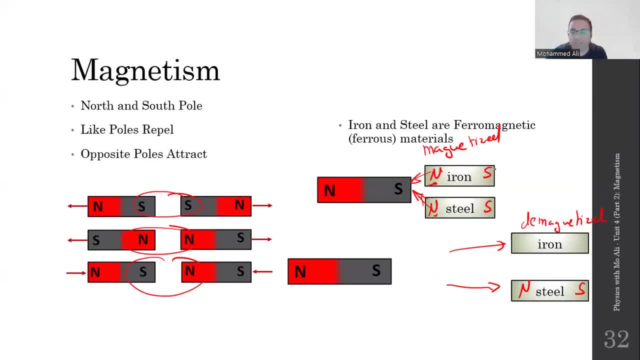 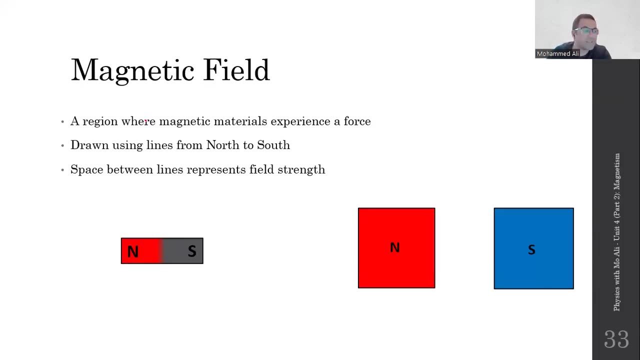 But the steel stays magnetized. Why? Because iron is what we call a soft magnetic material. It's only temporary, Whereas steel is a hard magnetic material. It's permanently magnetized. Okay, Magnets have a magnetic field, just like electricity when it had electric fields. 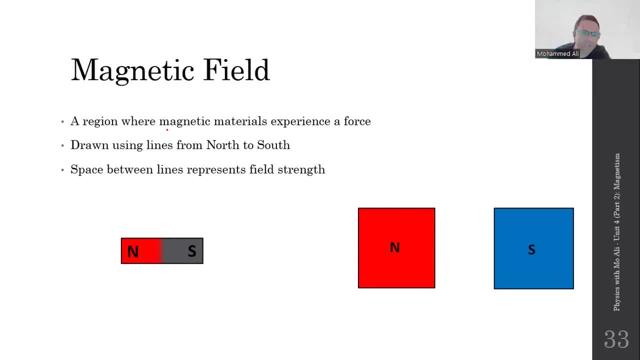 Magnets have a magnetic field. The magnetic field of a magnet is again a region where magnets experience a force. We always draw it using lines Moving from the North Pole to the South Pole, From the North Pole to the South Pole. 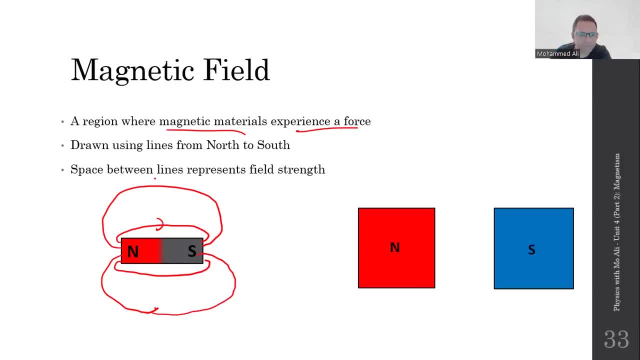 Oops, And there we go, Lines going out of the North and into the South. The space between the lines represents how strong the field is. The closer the field lines are to each other, the stronger the field, And the farther away the lines are from each other, the weaker the field. 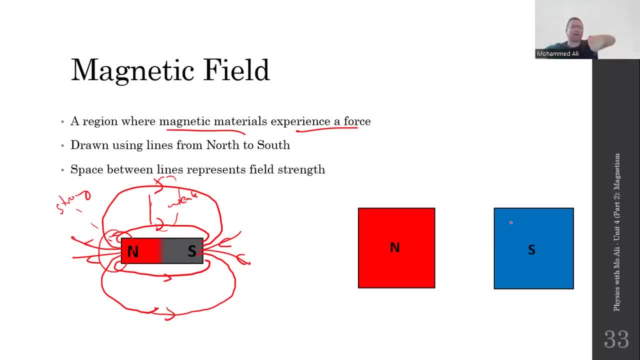 However, if you put a North Pole in front of a South Pole and you hold them- either because this is a horseshoe magnet or just two separate bar magnets and you've held them- the field lines are parallel to each other, Just like the electric field when it's uniform. 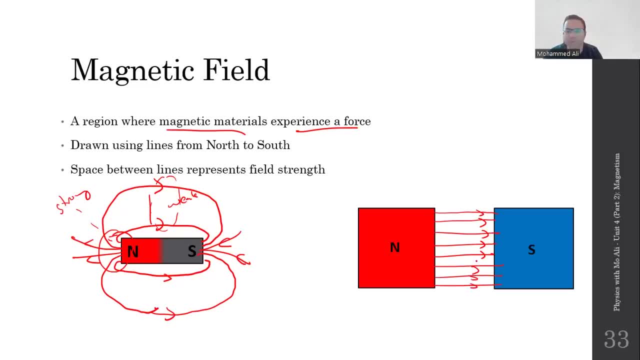 So this field is also called a uniform field. This is also called a Uniform field. Very good, The points have to come up from the edge, not from the same point. The lines have to come up from these poles. please Don't bring them up from the same point. 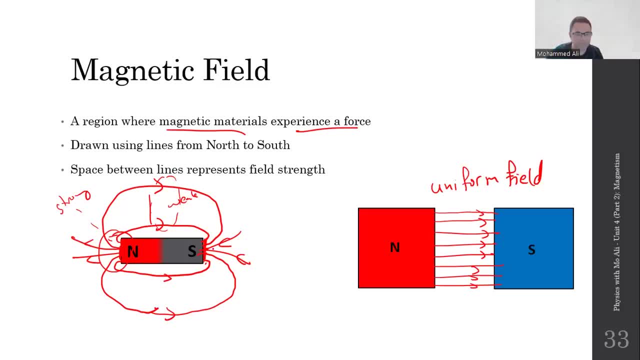 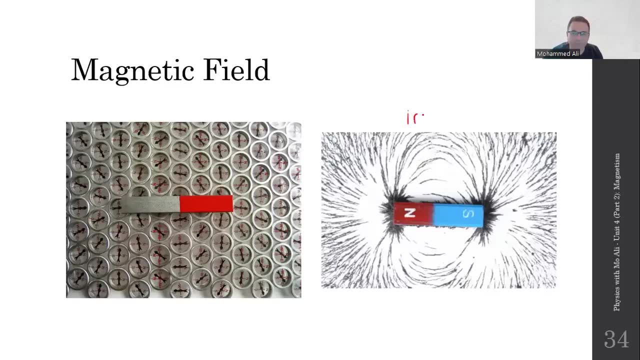 Bring them up from different points on the same pole please. Now, how do we see a magnetic field? If you use some iron filings- Or iron fillings, as some people say, that's fine too. The idea here is what? 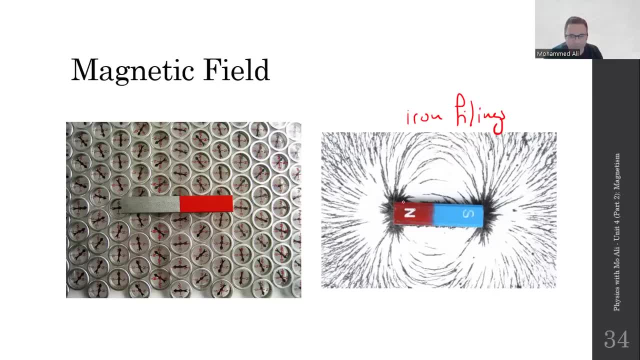 Is that when you have some iron powder and you sprinkle it all around the magnet, it takes the shape of the field. As you can see, the lines of this field move from north to south. Now, you don't know what the direction is, but you see the shape. 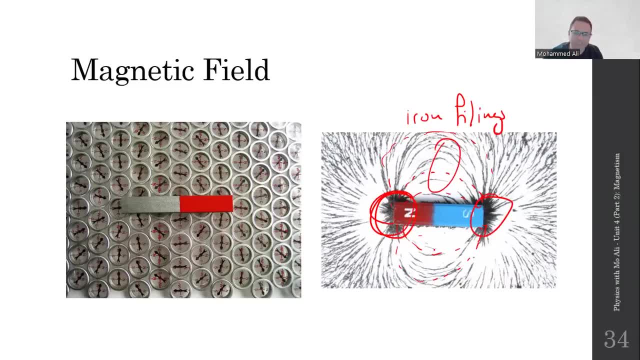 And you see how strong it is here and how weak it is here. If you want to see the direction of the field, you use a compass. This is called a compass. This is called a compass plotting method. You put a compass here and the needle of the compass shows you the direction of the field. 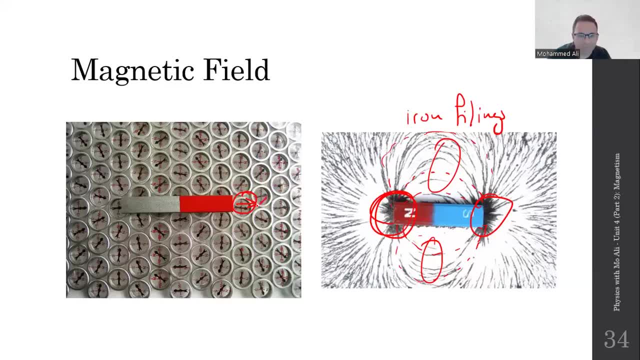 because it is also a magnet. So you mark a point where the compass needle shows. Then you change the location of that point, usually by putting the compass here at the end of this point. You see a new line. put it here. 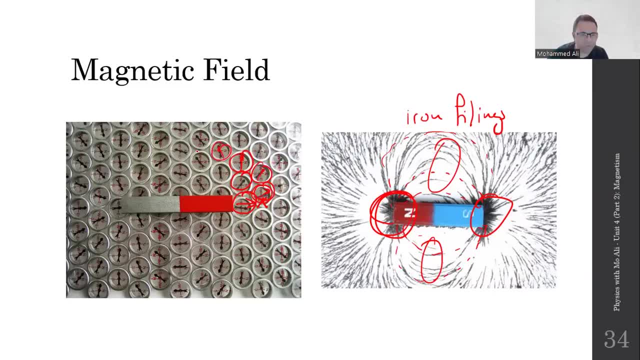 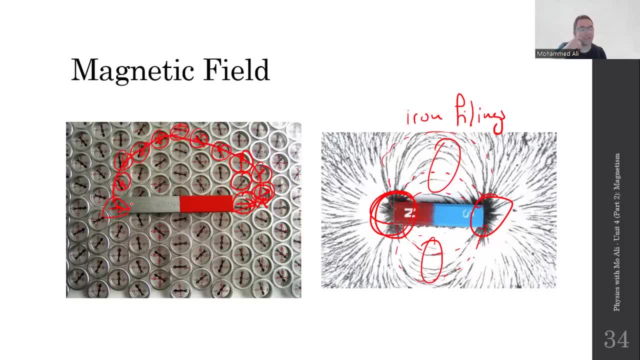 you end up with a line that shows you the direction of the magnetic field moving from the north to the south. So, even though I did not mark which side is north and south in this diagram or this image, this side is north and this side is clearly south. 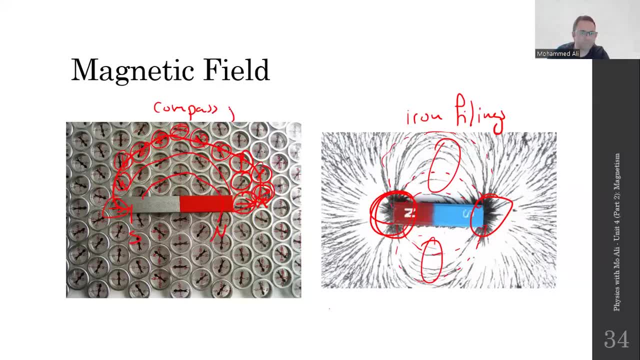 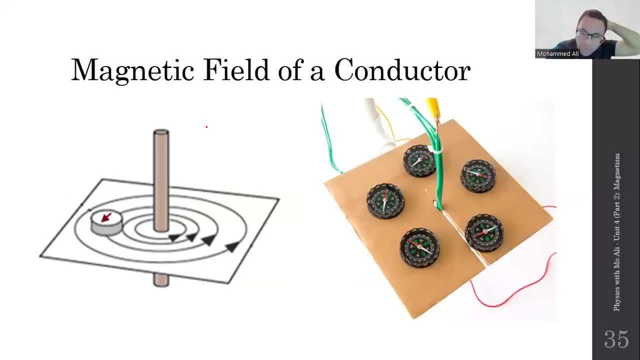 I forgot to write that Magnets are not the only thing that produce a magnetic field. A current also produces a magnetic field. This is the foundation of electromagnetism. If you have a current and you run it through a wire, as you run the current through the wire, 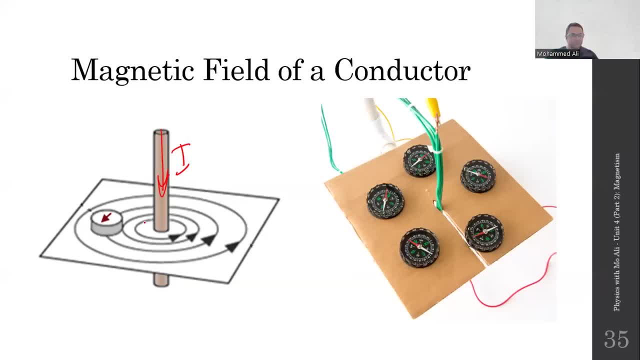 as you run a current through the wire, it produces a magnetic field. There is a magnetic field around it and the field is always circular. The proof of that is this: As you can see in this diagram, there is a wire and he ran a current through it. 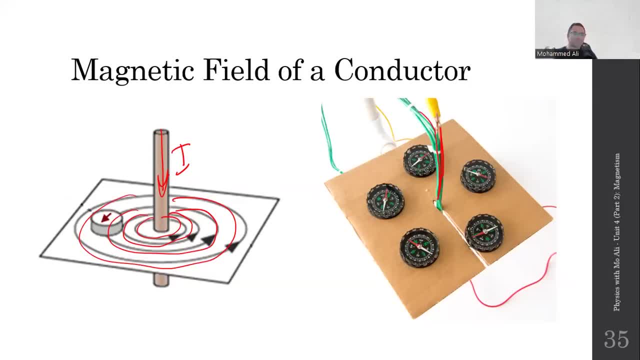 Now, he didn't tell us what the current was, what direction it was, but we do know that there is a current. Why? Because when he put several compasses all around the wire, each compass showed me a different direction, Even though a compass should technically point north, towards the north pole of the earth. 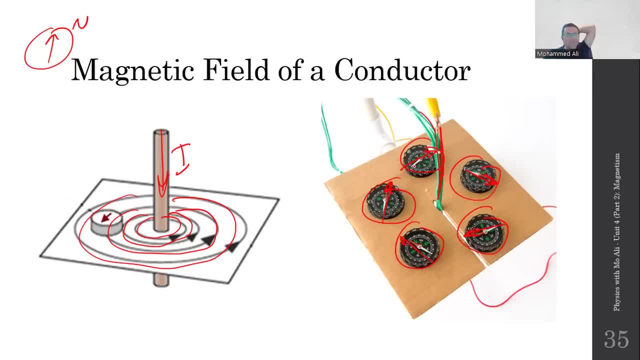 each current is pointing in a different direction. Assuming that the red line is the north pole, all of these are pointing this way. So the field line is either clockwise or anticlockwise. In this diagram it's clockwise. In the other diagram it's anticlockwise. 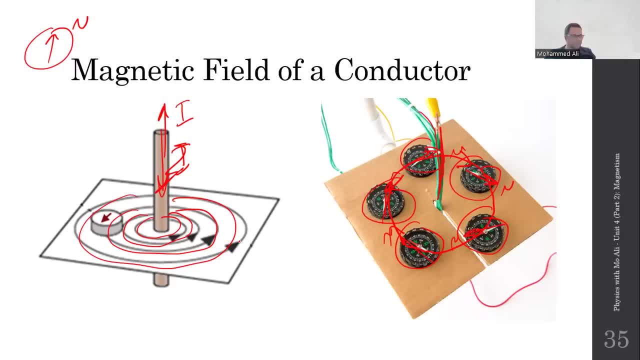 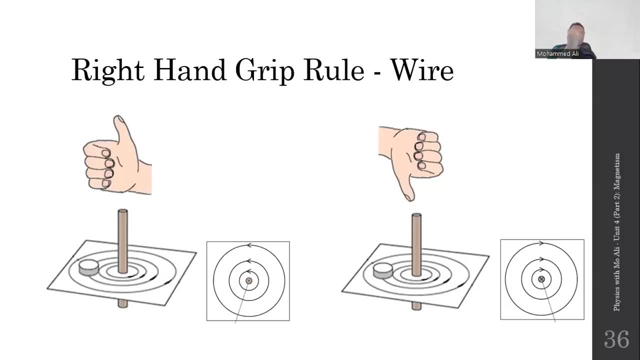 So actually the direction of the current I've drawn here is wrong. Now, how do I know? Because we have a rule called the right-hand grip rule. By using your right hand grip rule, you can control the direction of the current. 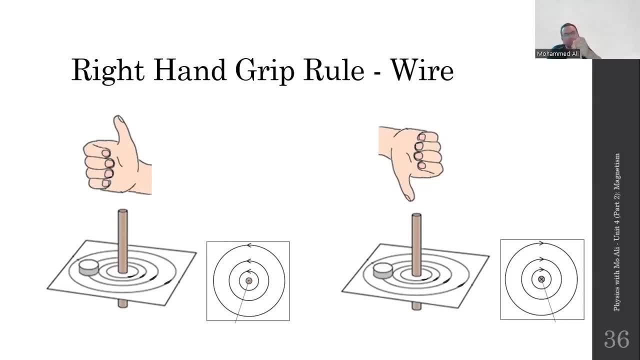 By using your right hand grip rule, you can control the direction of the current. So with my right hand, you give me a thumbs up. your thumb is the current And the curvature of the rest of your fingers is the direction of the field. 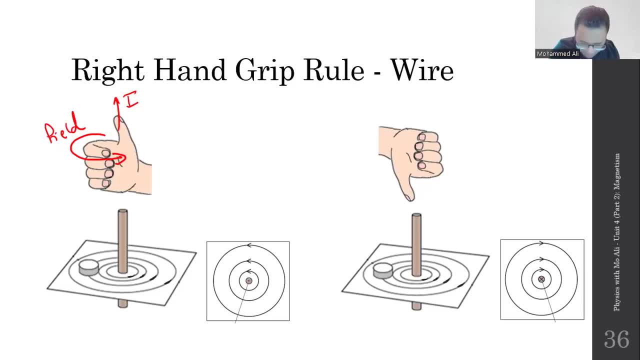 So if the current is going up, the field rotates. And look at your hand from the top: it rotates anticlockwise. If the current is going up, the field rotates anticlockwise. If the current is going up, the field rotates anticlockwise. 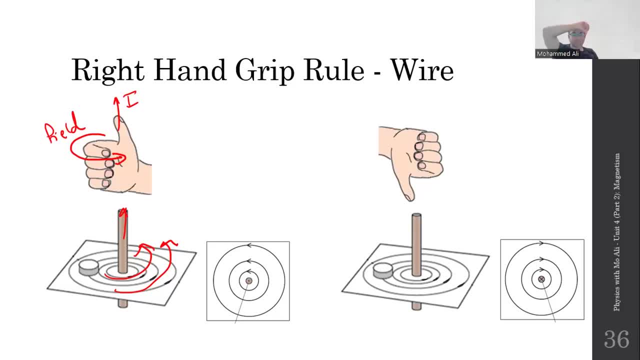 Give yourself a thumbs down, right, Because assume I said a very cringey joke. right now I can't come up with any, but I'm sure I'll come up with a cringy joke in a bit. So if you thumbs down, 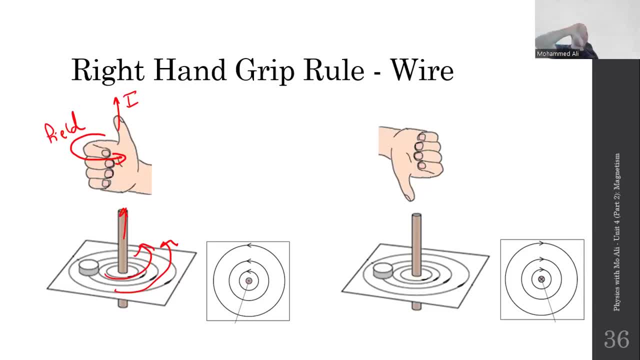 wait, should I say like and subscribe now? I hate saying that stuff, But anyway, if you give me a thumbs down instead of a thumbs up, your current is down, going down here, and the field is rotating clockwise. You don't have to use your hand, by the way. 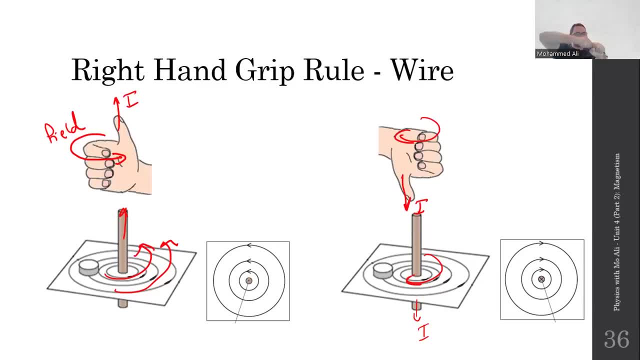 because this is just like a screw: If you screw a nail, clockwise or you unscrew it, anti-clockwise. clockwise goes in, anti-clockwise goes out. Exact same idea. That makes it easy, As you can see, as the space between the lines increases. 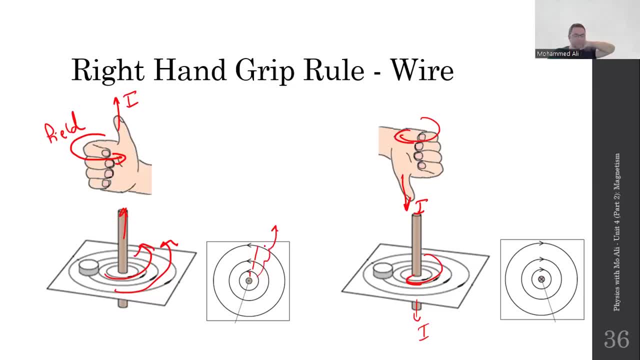 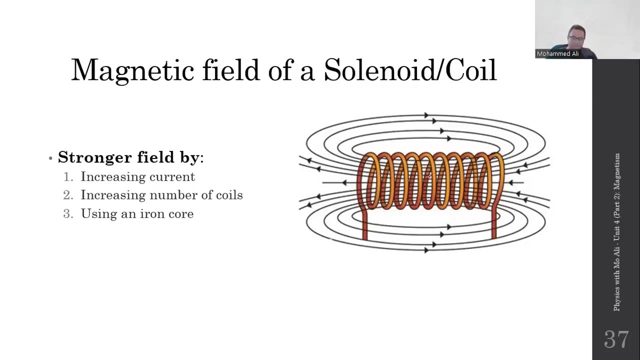 the field strength gets weaker because, it makes sense, You're moving farther and farther away from the center of the wire or this wire, So the field gets weaker and stronger near the center. So if you take that wire and coil it, as in turns into a coil- 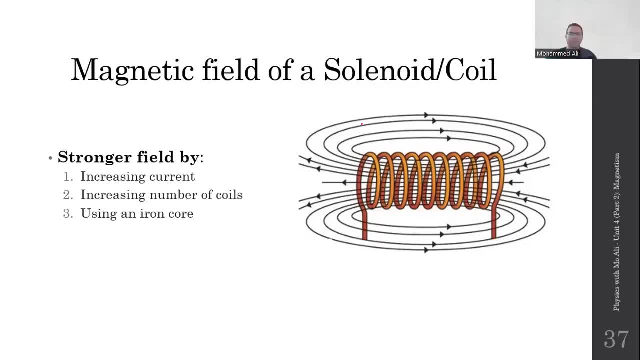 you end up with a magnetic field very similar to that of a bar magnet. We call this an electromagnet, or a coil, or a solenoid. So the field is from North to South Bordeaux as well, But the difference is is that you have field lines inside the coil. 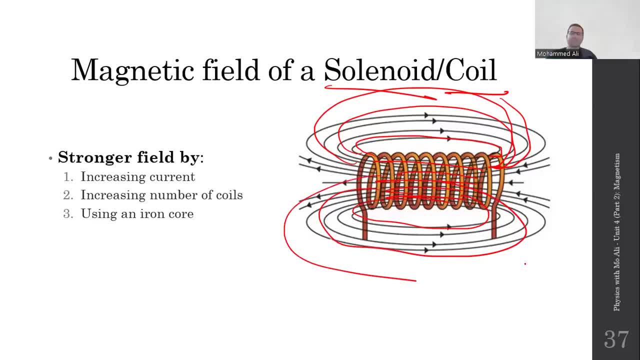 not just on the outside. Now, this is actually a very important observation. Why? Because it shows us. because it shows us that magnetism doesn't only come from magnets, It also comes from electricity. You can make this field stronger or weaker. 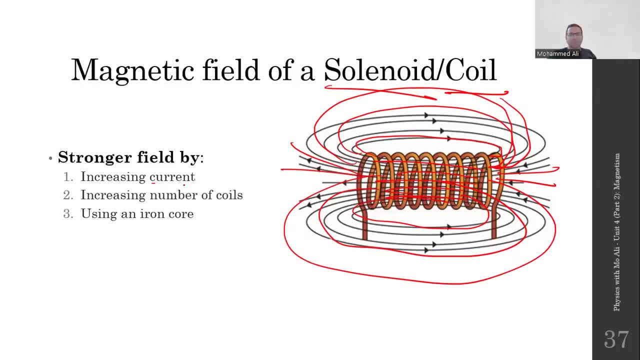 We can control how strong or weak this field is by controlling the current or the number of coils. So, increasing the current, like using a stronger battery, larger battery- Yeah, this is the right direction. Increasing the current increases the field, increasing the number of loops or coils. 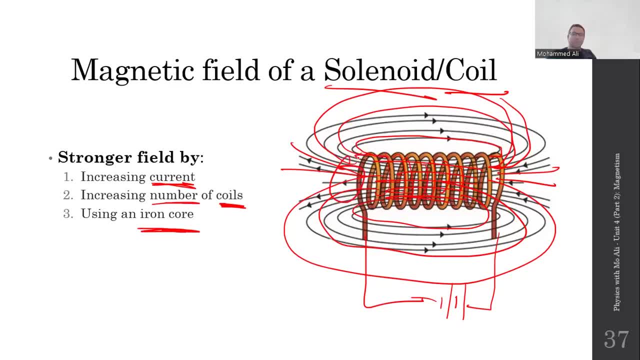 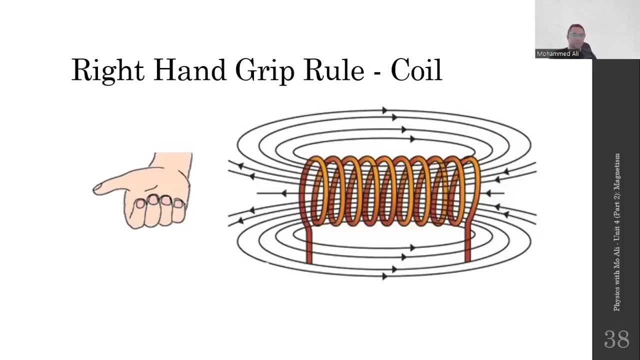 use more turns. that increases the strength, or using an iron core, which is just putting a piece of iron inside the coil. This magnetizes it and makes it strong. Okay, How can you tell what the direction is Using the right hand grip rule? 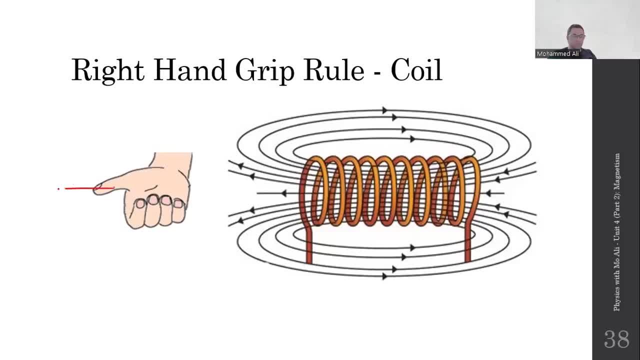 By looking at the direction. this is the same rule, but this is the North Pole, and the turn of your fingers, or basically your direction your fingernails are pointing to, is the current in the coil. So the current is moving this way, for example. 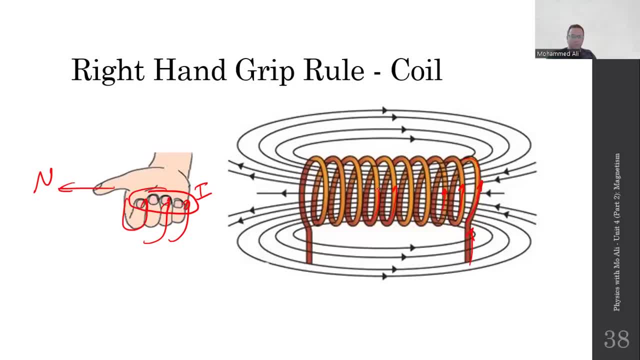 So it's going up, going around, going up, going around, going up, going around, and so on, and so on, and so on, until it goes down. That's because we connected it to a supply like this: This side will be North and this side will be South. 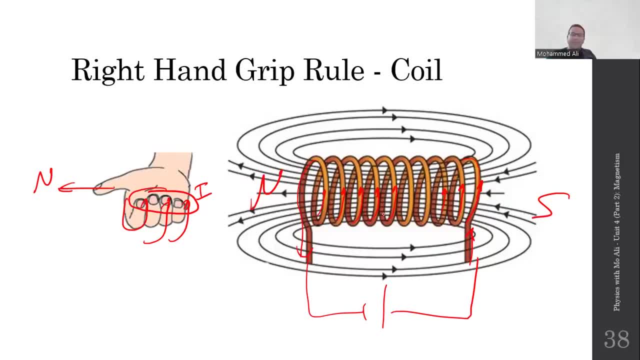 How do I know? Using the right hand grip rule, Look at the current on the outer face of the coil. All right, If it's going up. your fingernails are pointing up and they always have to be facing you As you coil your hand. your fingernails are pointing up. 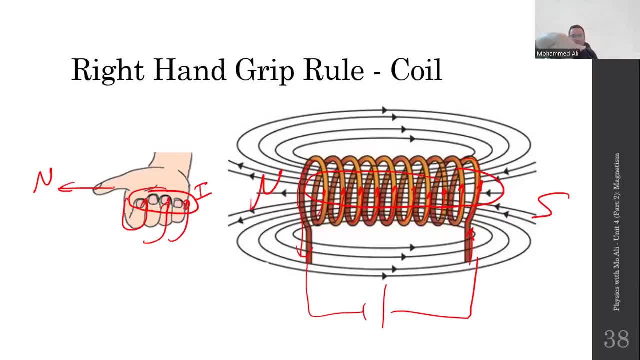 Your thumb shows you the North Pole, So the North Pole is on the left side. If I reverse the current so that the fingernails are pointing down, the current is going down, the North Pole will be to the right, But right now North Pole is to the left. 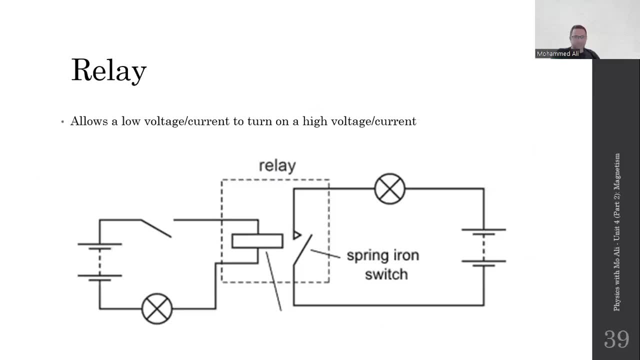 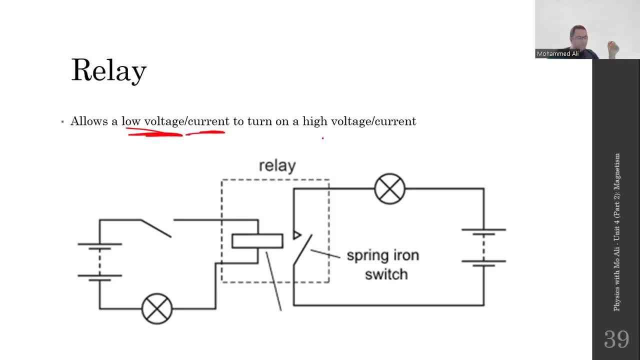 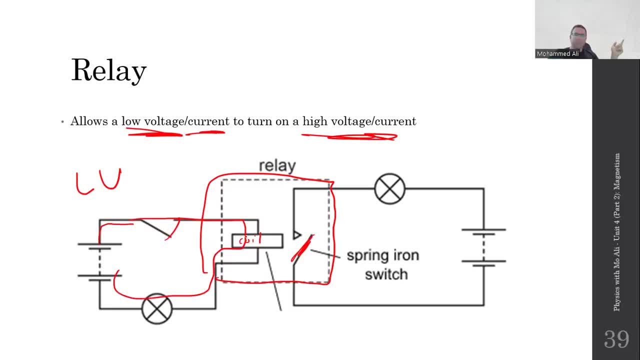 And when the current you close the switch and when the current goes through it, this coil magnetizes, which attracts the iron switch. So when this iron switch clicks and closes, this coil magnetizes, which attracts the iron switch. Oh God, I was about to close the entire thing. 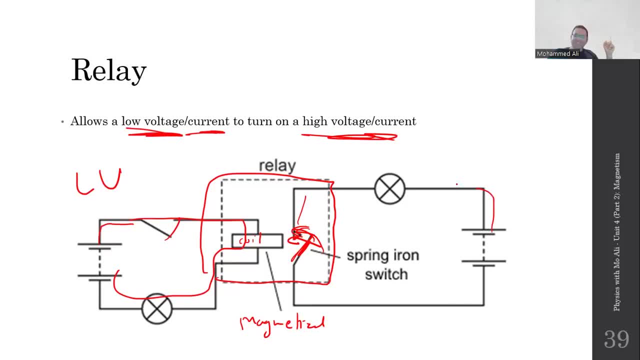 When you close the switch, the second circuit's current starts to flow and it turns on if this is the high voltage circuit. So it's only used to allow a low voltage circuit to turn on a high voltage circuit. Next, What about speakers? 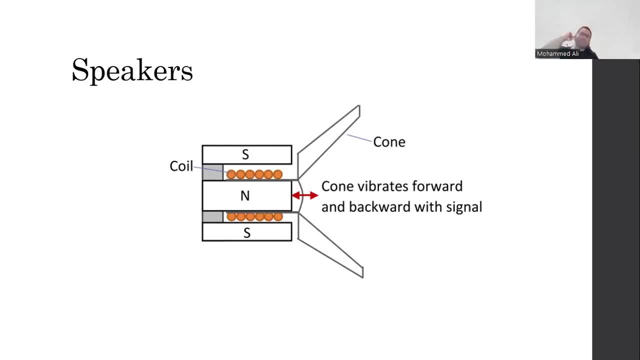 Speakers also use electromagnets. by the way, You know the speakers I have in my ears, for example- they're earphones but nonetheless it's a speaker. or the speaker of your phone, or if you have a giant Bluetooth speaker. 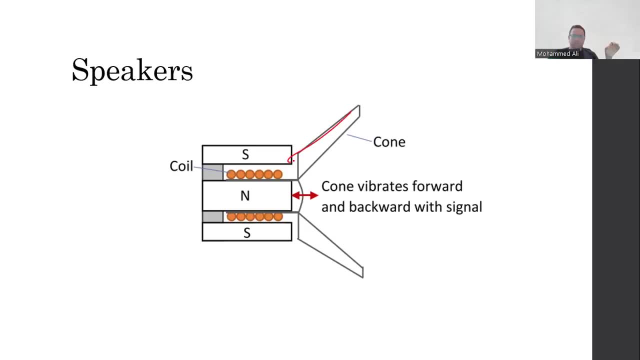 They all function roughly the same. You have a cone, and when this cone vibrates forward and backwards, it produces sound waves. It produces sound waves. The way we move this cone forward and backwards is by putting a coil around a magnet that's connected to the coil. 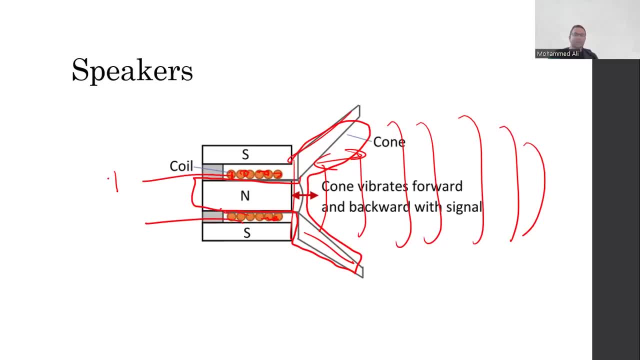 When the coil becomes magnetized by passing a current through it which contains the music, by the way. so we take the music signal, we turn it into a current which alternates a lot, And then, when it goes through the coil, 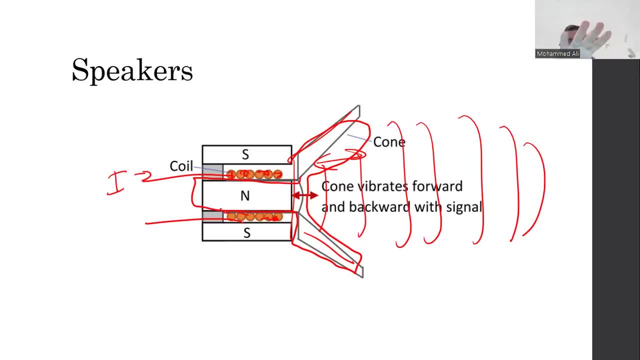 it magnetizes the coil, So it either repels or attracts the magnet that's connected to it, which moves the cone forward and backwards, forward and backwards, forward and backwards with the music, And that produces sound. All right, Very good. 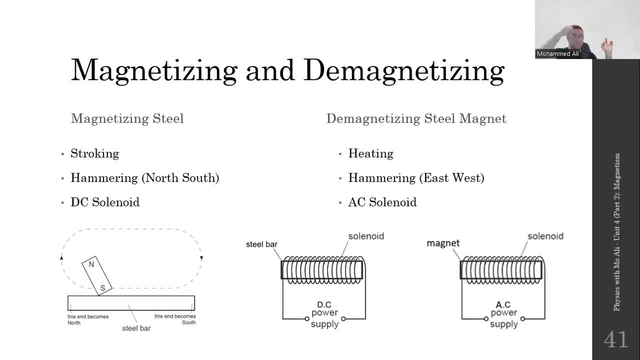 Now, before I answer questions, one last bit. How do I magnetize a piece of steel and make it a permanent magnet? You either stroke it- What do I mean by stroke it? Just get the magnet and rub it on the surface of this piece of steel until it comes back. 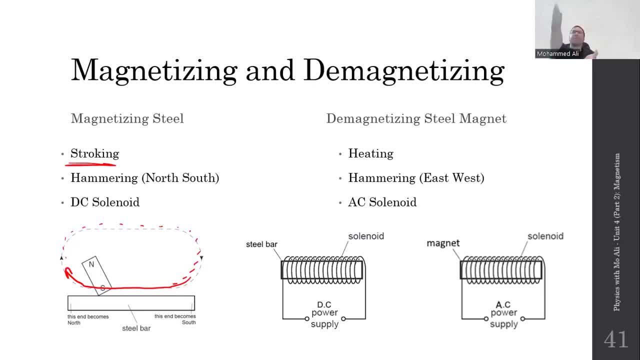 Just rub it in one direction, only in one direction, and then remove it, put it down, move it again in one direction. remove it, put it back down, move it in one direction. move it, put it back down, move it in one direction. 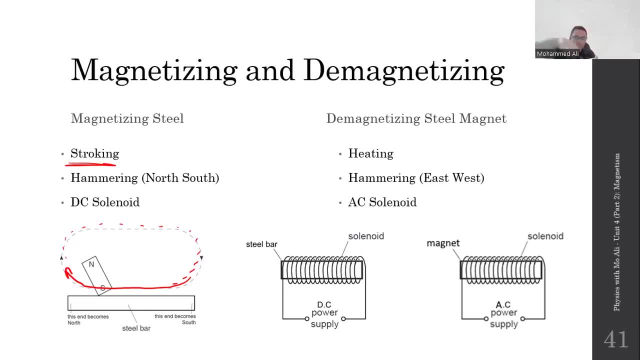 And so on. As you continue doing that, you're pushing the charge of the north and south poles in a certain direction. This end- let's say you have a south pole that's going down here, it's moving to the left- This end becomes south and this end becomes north. 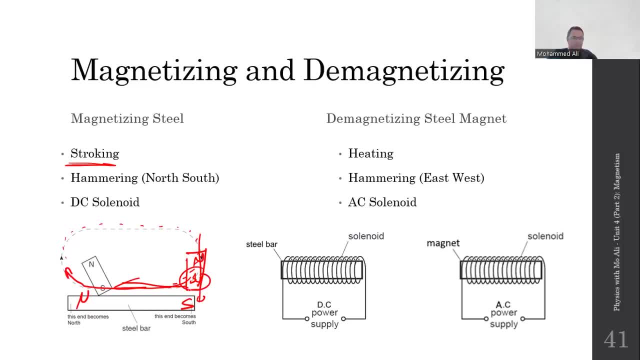 Like the end that you push down and you start the magnet stroke with goes south. The next method is something I don't really like. It's called hammering. You take the magnet and you hold it in a north direction, A north to south direction. 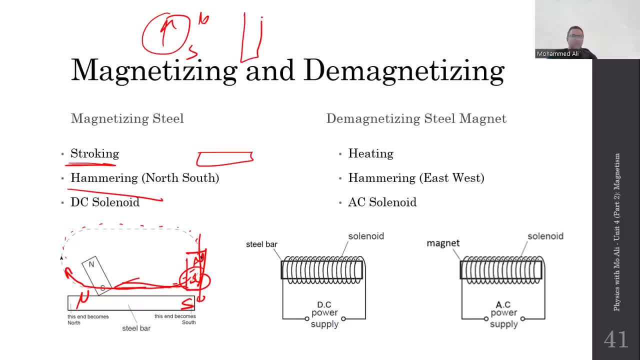 So let's say: here's a compass and here's the north to south of the earth. You take a magnet and you hold it aligned with the north and south of the earth, And then you bam, bam, bam, bam bam. 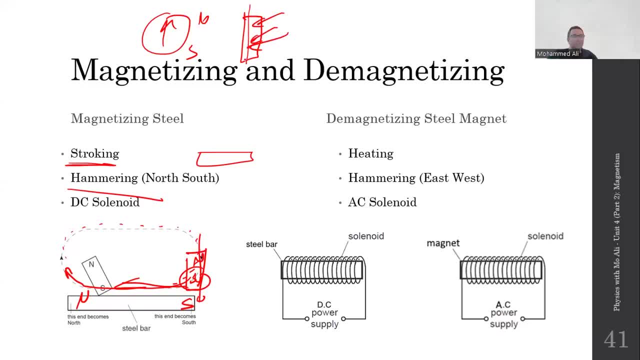 start hammering it, hammering it, hitting it harder and harder and harder And it will eventually magnetize because it gets the magnetic field of the earth. It takes the same field of the earth, However big problem then Hammering it in any other orientation. 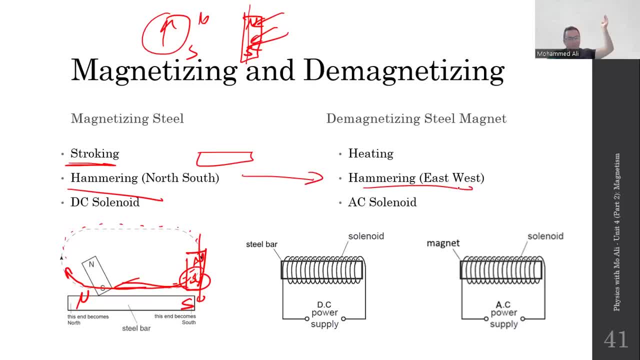 demagnetizes. by the way, this is why a method of demagnetizing is hammering as well, but holding the magnet east to west. This is why I don't like hammering very much. It's not very consistent. The best method to magnetize a piece of steel. 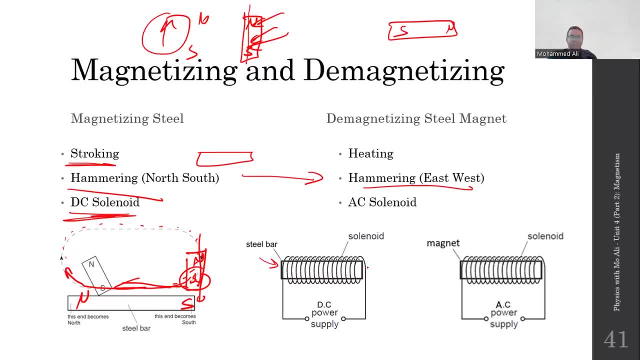 is to get a coil and put the steel bar inside the coil, inside the solenoid, and connect it to a DC supply so that it has a north and a south pole. This will magnetize the steel inside very quickly and very strongly Because, remember, you can just turn it on. 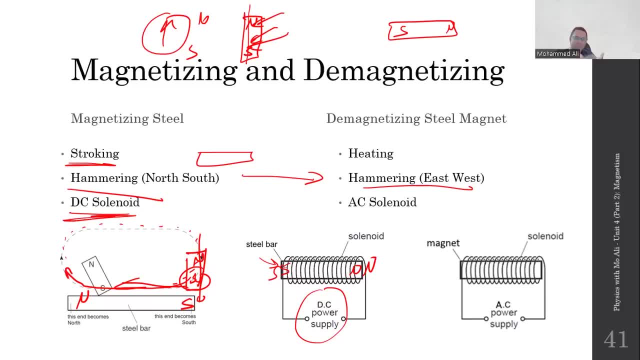 and there's no effort involved on your part. You don't have to hammer anything, You don't have to stroke anything, It's just: you just leave it there And several minutes later it's a nice permanent magnet. Have a nice day. 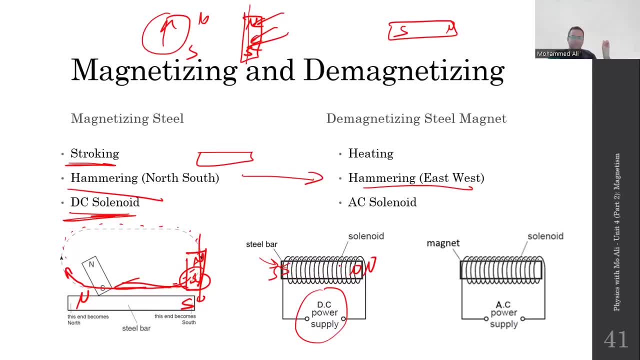 Turn it off the supply and then switch it off and you take it out. To demagnetize a piece of steel, you either heat it to very high temperatures. You don't melt it because some people, the moment I say, heat it to high temperatures. 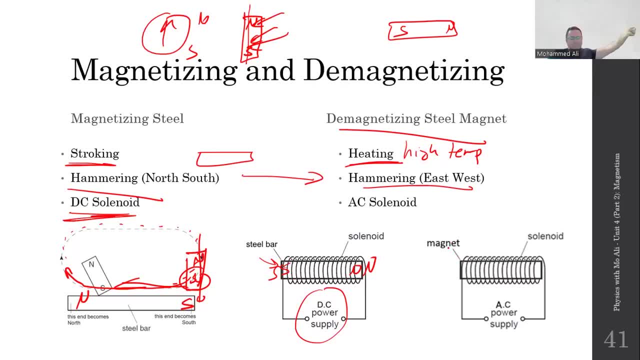 they imagine the metal melting. No, You heat it until it's nice and red and hot, but not melting, Okay. Okay, You can hammer it as you hold it from east to west, or you can put it inside a coil or a solenoid. 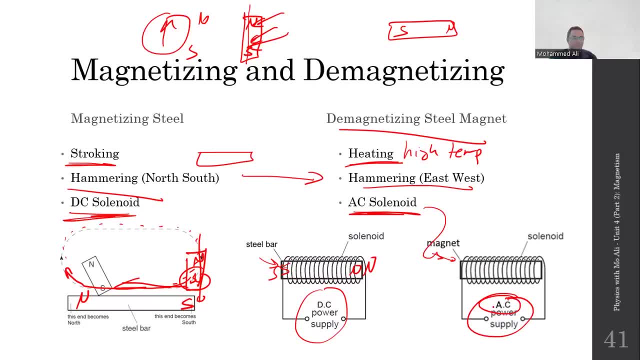 but you connect the solenoid to an AC supply. So what's AC and DC? again, You don't remember? We said DC is short for direct current, Which we revised a little while ago with diode. So it's a constant supply with a constant positive. 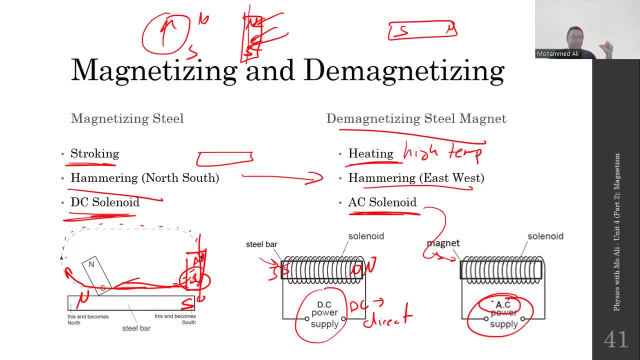 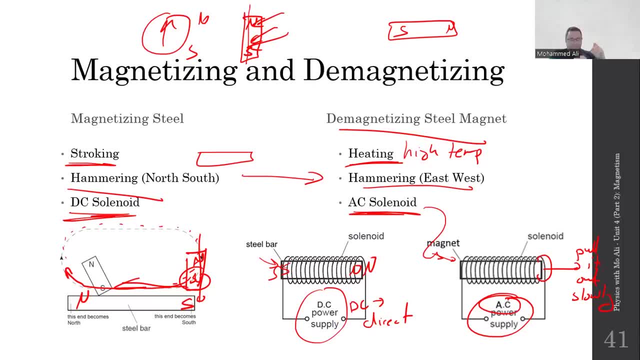 that will demagnetize your supply, your magnet. So AC means the current keeps alternating. And why is this important? Because the poles of the coil will not be constant. It won't be North and South. It keeps changing the North and South poles all the time. 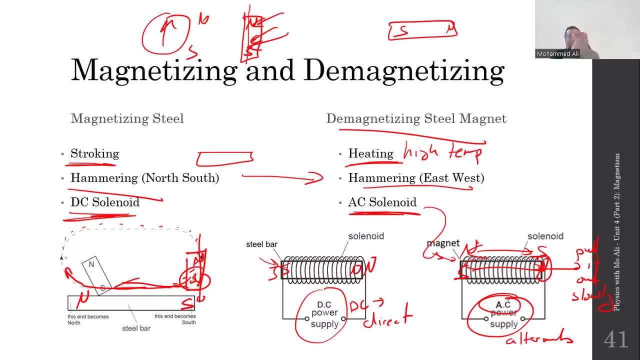 They keep alternating North and South all the time. So you're messing up the magnet on the inside right And then you pull it out slowly. So again, three methods of magnetizing, stroking in one direction. I should make a one direction joke here. 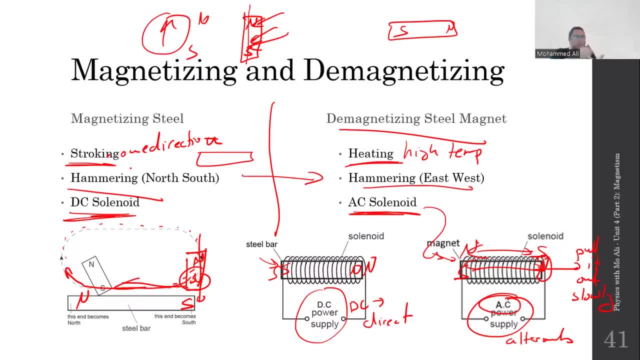 but we don't have the time Hammering. but you hold the magnet North to South because when you hold it North to South it takes the direction of the field of the Earth. When you hold it East to West it doesn't take the direction of the field of the Earth. 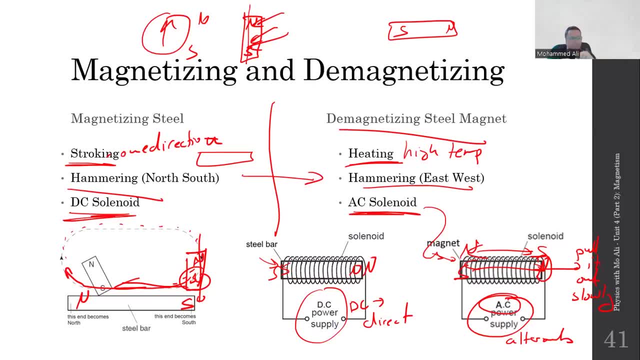 That's why you can demagnetize it by hammering it East to West. That's the difference. And when I say East to West, I mean you're holding it East to West. So if this is the North and South of the Earth, 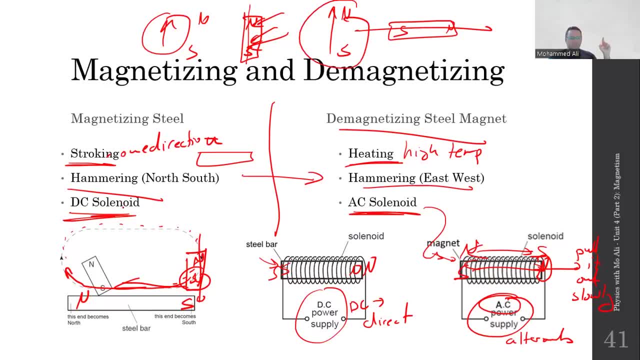 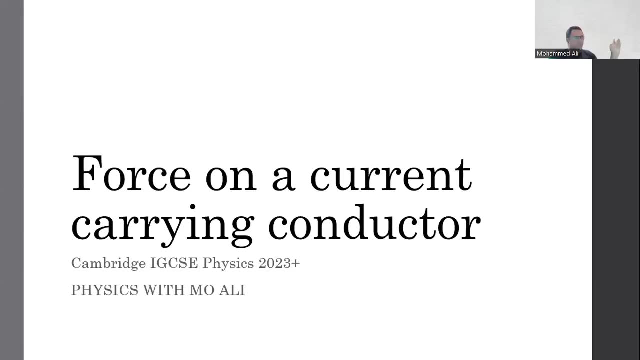 you hold the magnet sideways, not up, And then to magnetize you either put it in a DC coil or solenoid or put it in an AC coil or solenoid to demagnetize, But you pull it out slowly Before we finish up magnetism over the next 15 minutes or so. 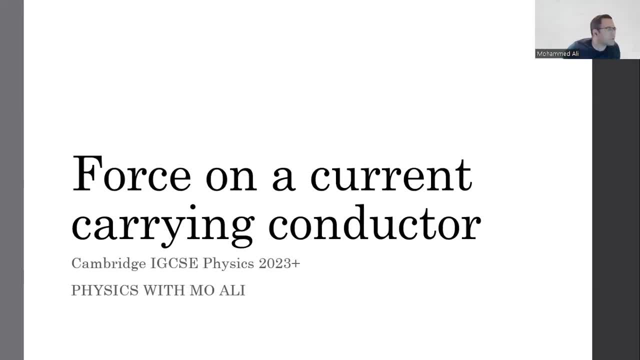 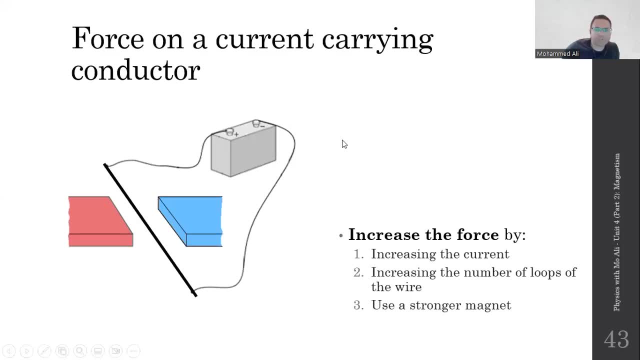 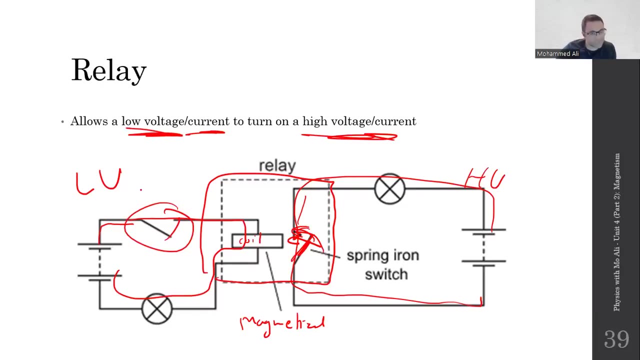 let me take a look at some of these things. There are a couple of questions. Why don't we just turn on the high voltage circuit right away? I'm sure that was regards to the relay. Sometimes this is not us. Sometimes this is an electric circuit like your phone. 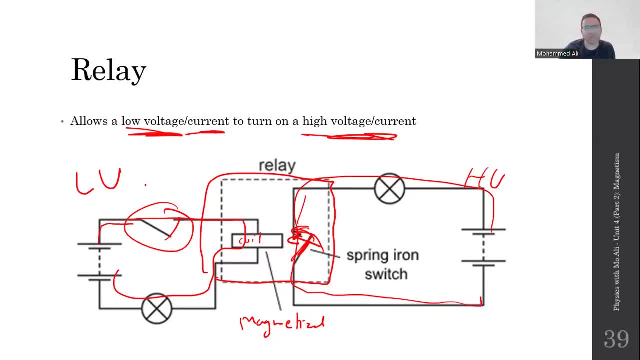 or like an infrared sensor. These are all components that are low voltage. They're not designed to work with high voltage supplies, but you want it to control a high voltage supply, Like an air conditioner. So you've got the temperature sensor in your air conditioner. 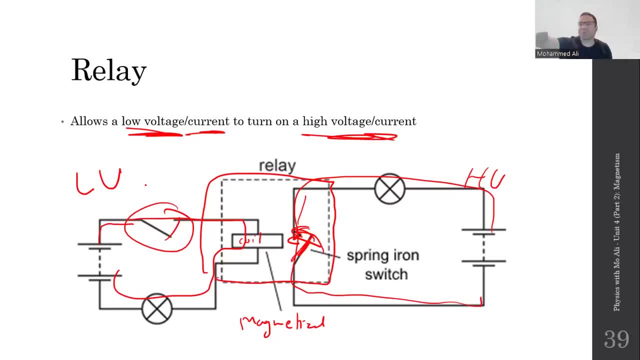 that needs low voltage to work but it needs to turn on or off the rest of the motors inside your air con. So we put a relay inside to allow it to control the higher voltage circuit. That's why we can use a relay, but that's why we need to use a relay. 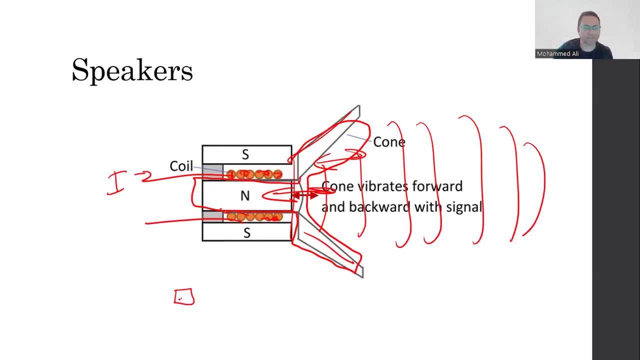 If you didn't understand the speaker, it's very simple. If you have a magnet here- just let's say a North pole of a magnet Here- attach it to a piece of paper and then I get a coil here, Depending on the direction of the current of this. 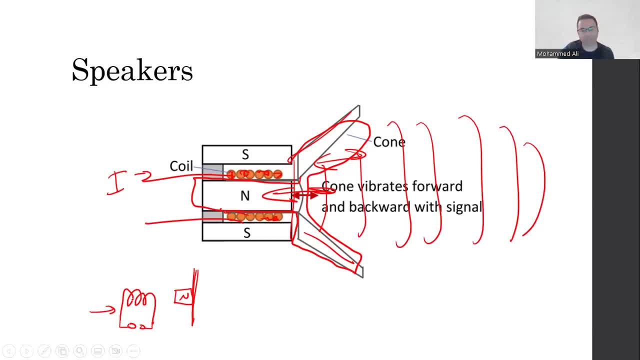 in this coil, one of two things happen. One of two things happen: Either this magnet is attracted, so it moves to the left, or it gets repelled, So it moves to the right. But if the current here is alternating, because you know, 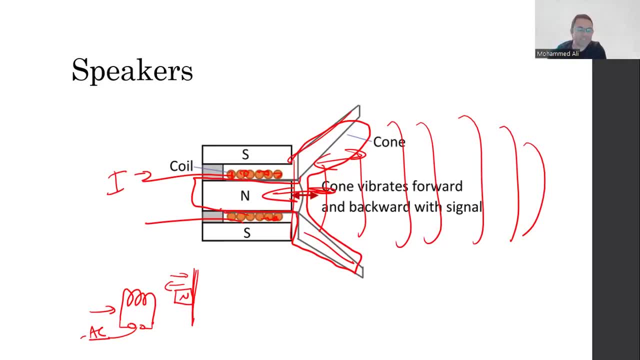 it's music and the music- voltage and current- keeps changing. This magnet continues to be attracted and repelled, attracted and repelled, attracted and repelled. So if you have a sheet of paper connected to that magnet, it'll keep getting pushed forward and back. 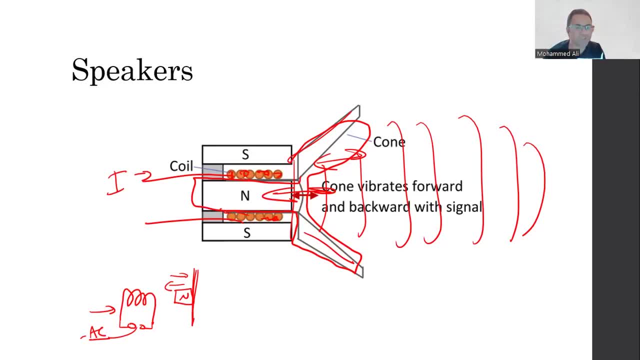 forward and back, forward and back, And that's what creates noise or sound, The motion of that cone or paper back and forth. So what moves, it is the music. The music produces a current that's alternating, and the current goes through the electromagnet or coil. 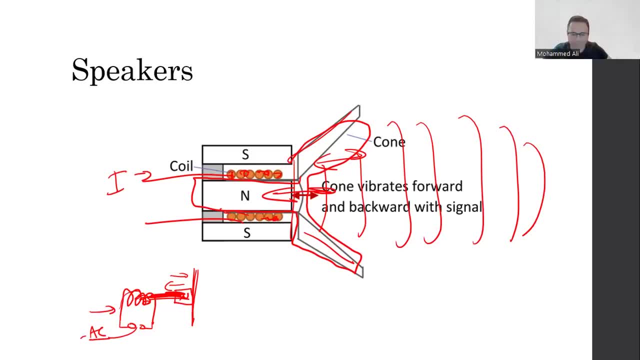 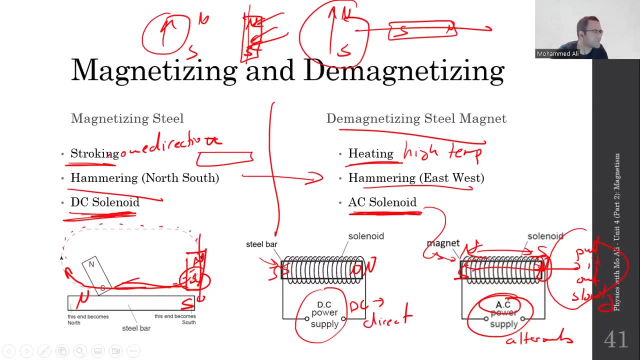 which attracts and repels the magnet, moving the speaker back and forth, And we already answered what's AC and DC. Very good, I mean honestly. here's a good question. Why isn't stroking in a different direction, or in different directions, a way of demagnetizing? 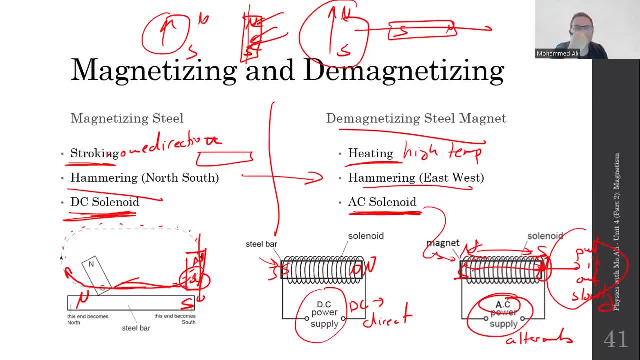 I mean it does. To be honest, it is, but it's even weaker than hammering. It's even worse than hammering. So we don't add it as part of our. you know, we don't add it as part of our options. 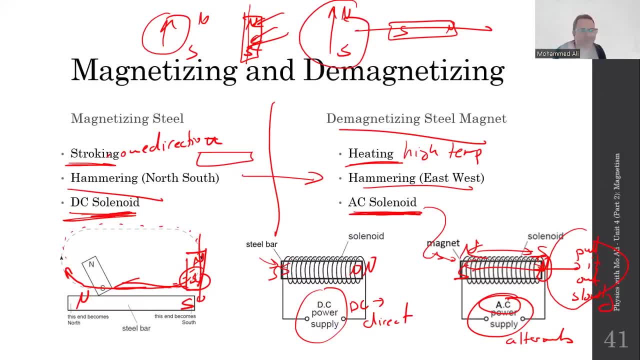 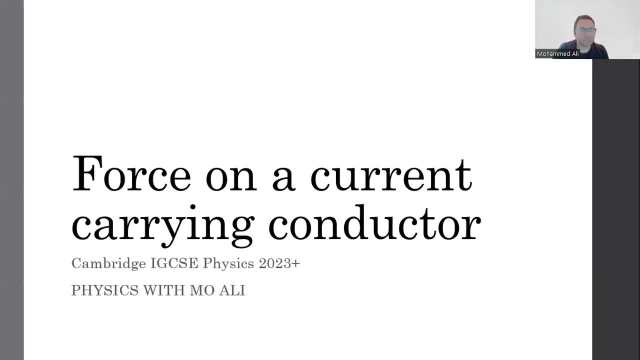 but yeah, it should technically demagnetize, but it's very weak. So we just go like, eh, we don't know, We don't talk about that, All right. Moving on, Finally, back force on a current carrying conductor. 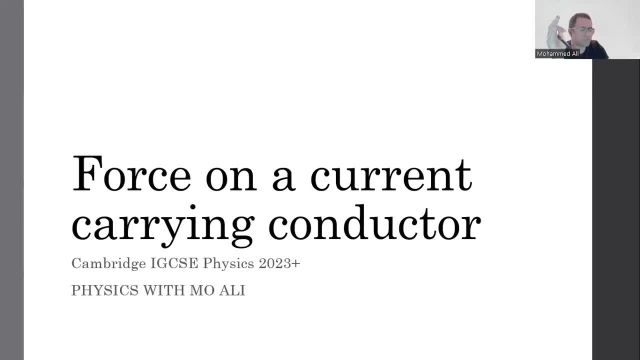 We have three things to finish and I'll be going through them very quickly because, to be honest, I just want you to memorize certain points of these devices. The thing I want you to understand will be in a bit, Electromagnetism. 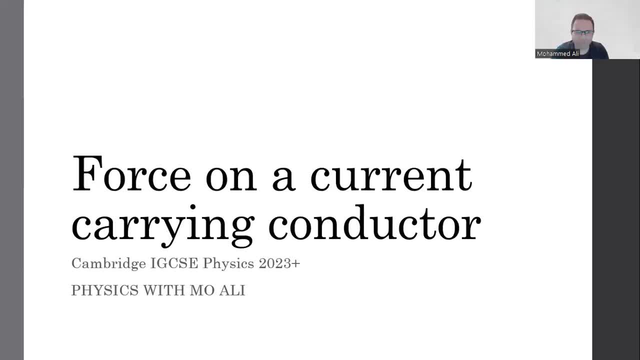 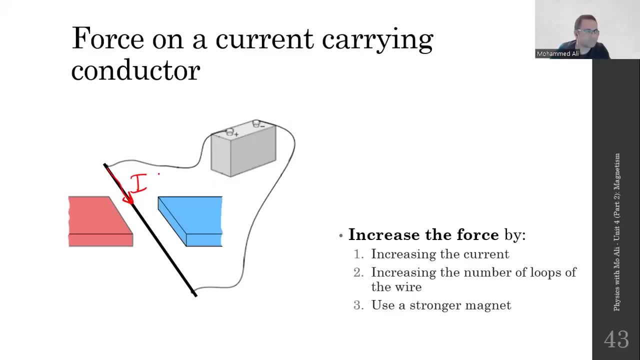 Electromagnetic induction. You need to understand it properly, but the rest you can just memorize. So what's this force on a current carrying conductor thing? If you pass a current through a wire by connecting it to a battery and this wire is placed between the poles of a magnet? 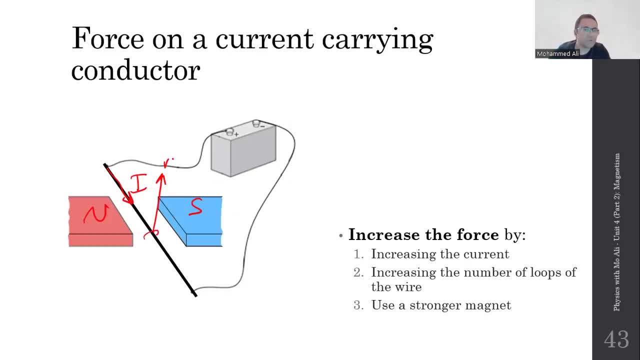 this wire will move Again. this wire will move Why? Because the magnetic field of the magnetic field and the current in the wire, to be specific, and the magnetic field of the magnet, interact, So you have a magnetic field from the wire. 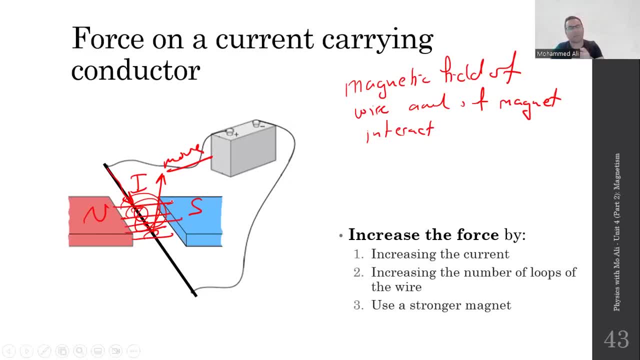 You have a magnetic field from the magnet. These two bam smack into each other And they apply a force on this poor wire. over here The force is always in a direction, So that it gets pushed out of the magnet. So it's either getting pushed out or down, up or down. 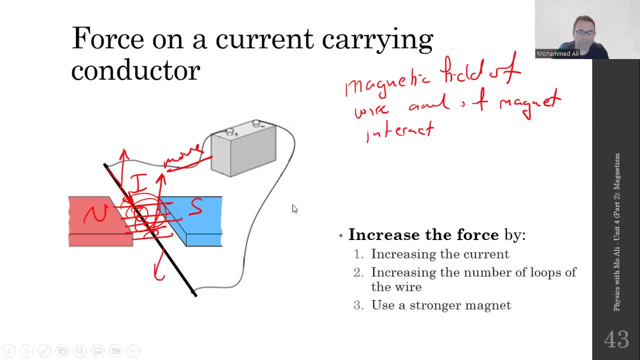 What direction we're going to see now. oops, sorry, We'll see which direction, but the value of this force that causes this wire to move depends on the current, because, you know, if you increase the current, the magnetic field of the wire is stronger. 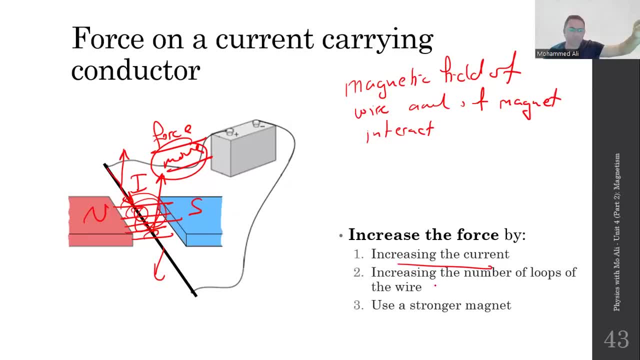 So it moves the wire with a bigger force. It depends on the number of loops. So instead of having one wire, you can have two, you can have three, you can have four. that increases the force, Or we can use a stronger magnet. 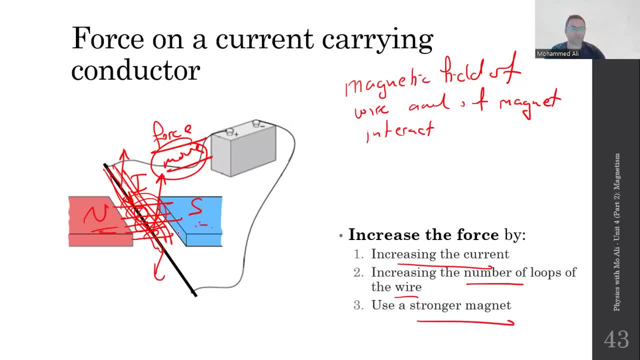 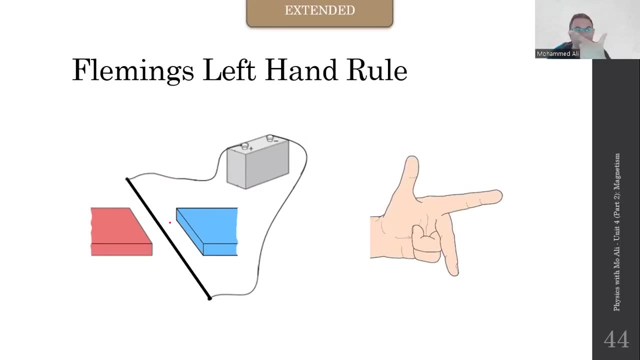 You can replace this with a stronger magnet and it will move the wire with a stronger force. How do we know the direction? The direction depends on the direction of motion, depends on the current and the magnetic field. We have a law called Fleming's left-hand rule. 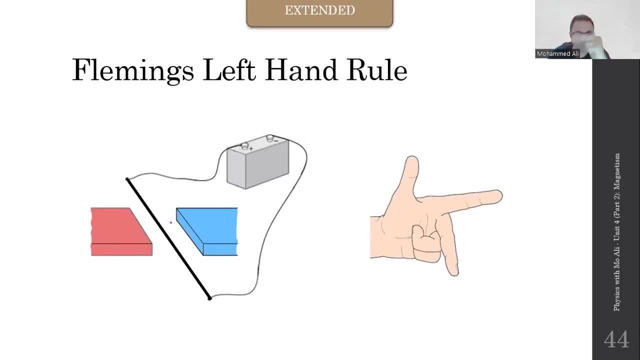 With your left hand. you turn your hand like it's a gun in a sense. This is your index finger, This is the magnetic field, Your middle finger is the A current and your thumb is the force. Yeah, your thumb is the A force. 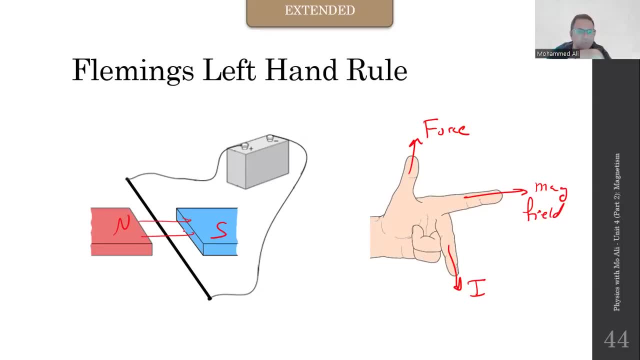 So north and south. magnetic field is from north to south And this is the A, the current. So if the current is moving this way, look how I hold my hand. First, you hold it from north to south. Always start with the magnetic field. 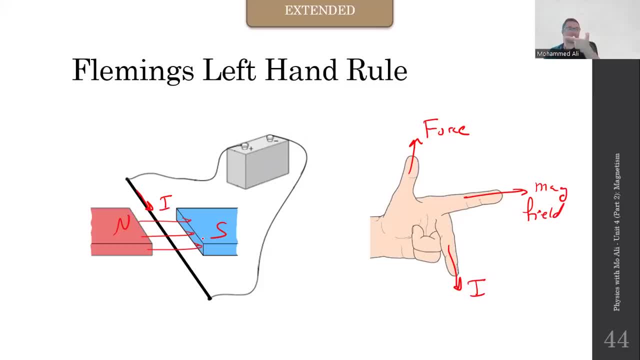 And then the middle finger is the current. You only have one of two options. It's either towards you, towards your mouth, so you can bite into it, like why am I biting my finger Anyway? so magnetic current is towards you. 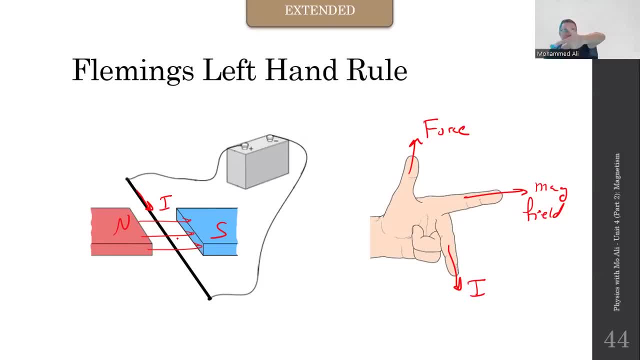 or the current is away from you. You only have one of these two directions, and it's either towards you or away from you. I can see the appeal of babies sucking their fingers, but nevermind So, anyway, let's see. Sounded so weird. 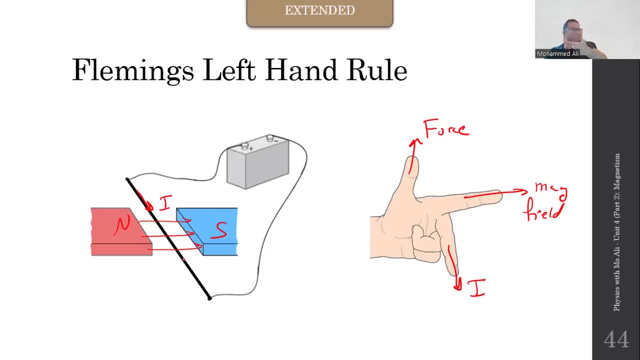 Guys, move on. I'll assume this is edited out and I did not say anything creepy. So what's the third finger, My force, my thumb, my thumb. My thumb is pointing upwards, which means the force is going to be upwards. 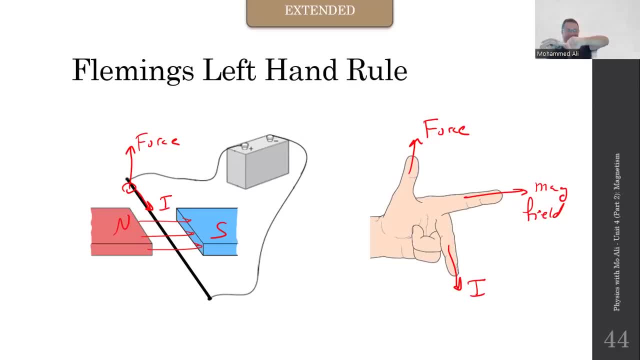 If I reverse the current, if I reverse the current and I have the current go into the page. this way the force is downwards. So by changing the direction of the current you change the direction of the force. This needs a little bit of practice. 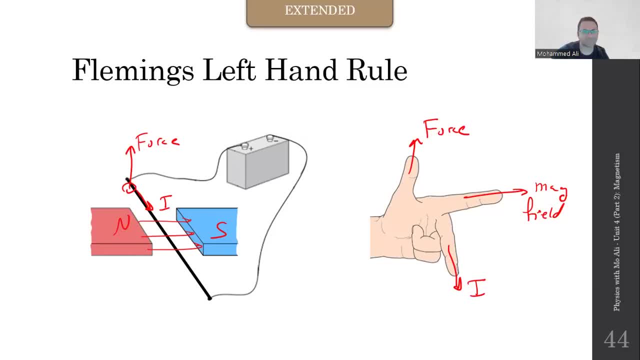 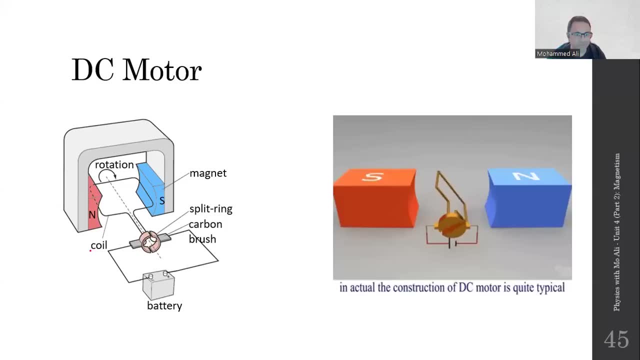 but you'll practice as you solve some more questions. And finally, we take all of this and we design a DC motor. DC motor consists of a coil, just a rectangular coil. You can see the animation on the right. This is the coil that's going to be spinning now. 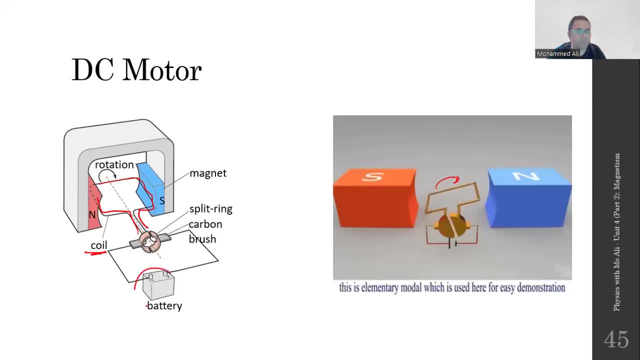 You have a magnet surrounding it, and then you have a battery Connected to a split ring and some carbon brushes. The concept is simple. Current flows through the coil, The wires of the coil, experience a force according to Fleming's left-hand rule. 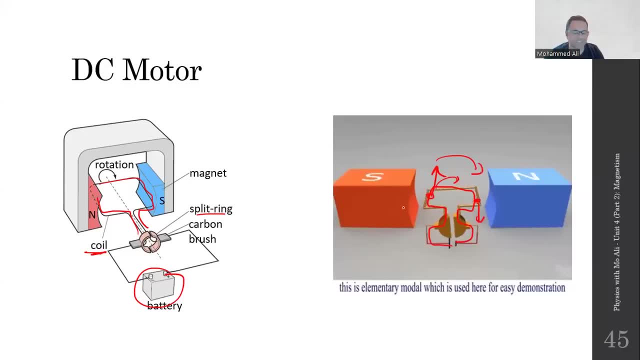 This goes up and this goes down, so it rotates. That's literally it. That's all what happens. You can make it rotate faster by increasing the number of turns, or by increasing the current, or by using stronger magnets. Okay, Next. 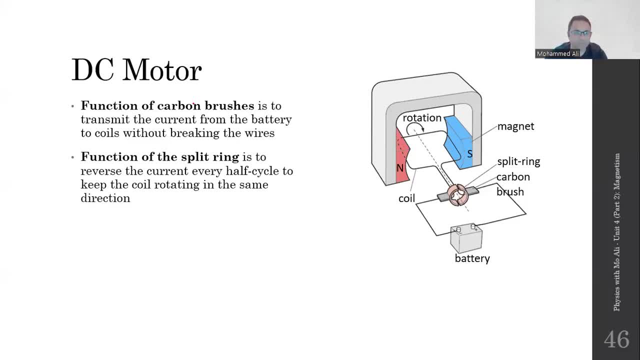 Now, what's the function of a split ring and carbon brush? Again, just memorize them. The function of the carbon brushes is to conduct electricity from the battery to the coil without breaking the wires of the circuit, Whereas the function of the split ring 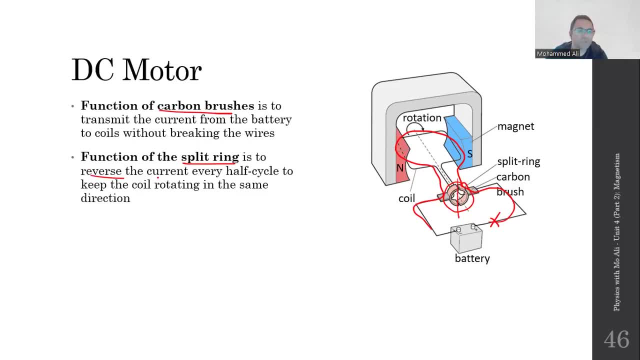 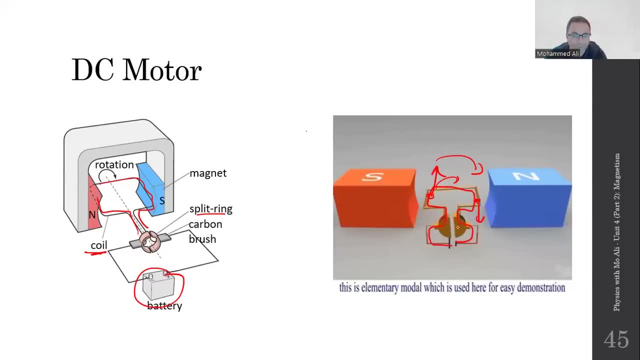 this thing over here that's cut in half is to reverse. to reverse the current every half cycle to keep the coil rotating. Because here's the thing, Without this split ring, which is half of the time touching the positive side of the wire, 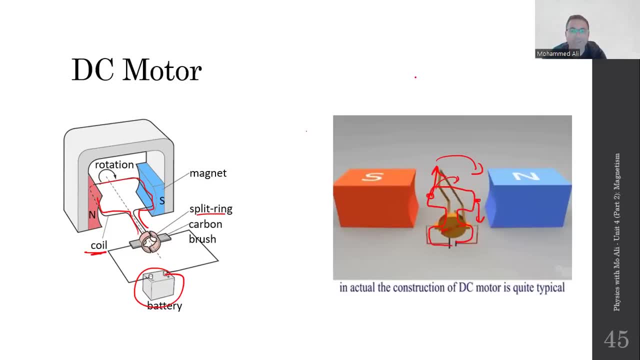 and half time, touching the negative side of the wire. without it, this coil would just get stuck, Like it would get stuck in a vertical position like this: This is the north and this is the south- To just get stuck in a vertical position. 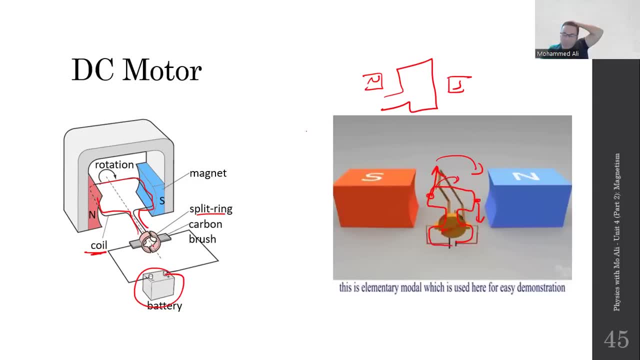 and it wouldn't move. So without the split ring, it will not be able to rotate. So without the split ring, it will not be able to rotate. It will not be able to rotate. This is only for the motor, all right. 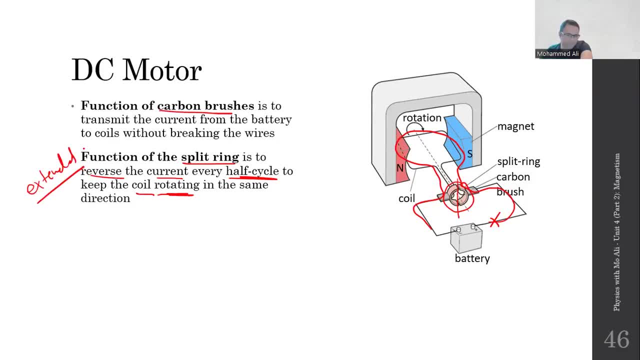 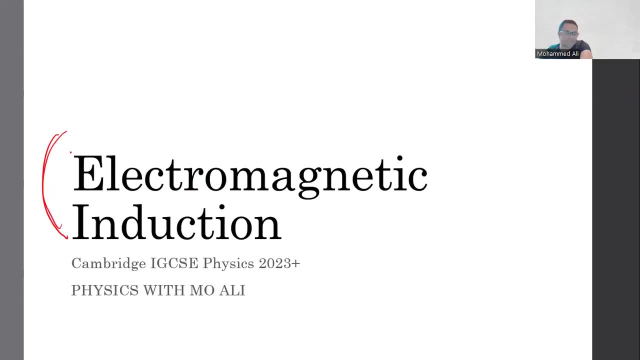 And, honestly, this part is extended and I forgot to put the label here. but just this part. Okay, This next part, which explains the generator effect, must be understood because it's a very common question trope: What is induction Generating electricity? 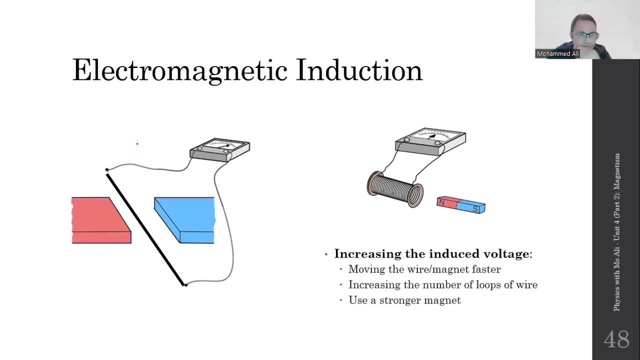 What? Yeah, we generate electricity. How, If you get a copper wire, place it between the poles of a magnet and you move the wire up and down through the magnetic field of this magnet. as you move the wire up and down through the magnetic field of the magnet, 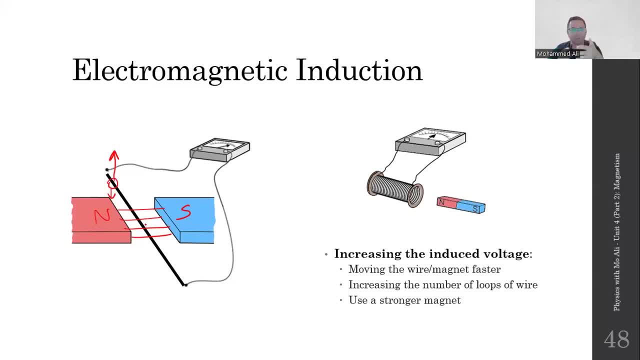 this generates a current. So why does that happen? Because when the wire look at my fingers, my fingers are the magnetic field and this pen, the stylus, is the wire Cause, when the wire cuts through the magnetic field lines, this forces the charges inside to move. 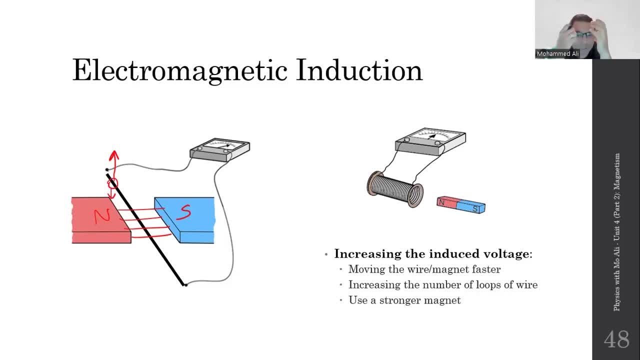 If you stop moving, the charges inside also stop moving. Wait, if charges are moving, that's called the current And the current moves because there's a voltage. So clearly, by moving the wire up and down through the magnetic field and cutting the magnetic field lines, 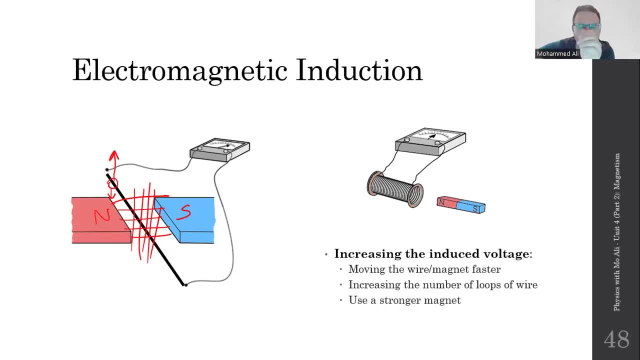 I don't physically mean you cut, I just mean you go through them, You change through them. This generates electricity. This is called electromagnetic induction. It's when you generate a current or a voltage, when a wire or a conductor cuts through a magnetic field. 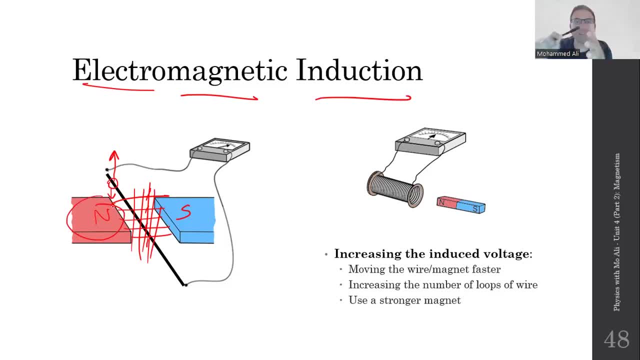 Nobody said you have to move the wire. We could move the magnet. The important thing is that the cutting happens. So either move the magnet or move the wire. So the best way to do it is to get an actual magnet And it's magnetic field will cut through the coil. 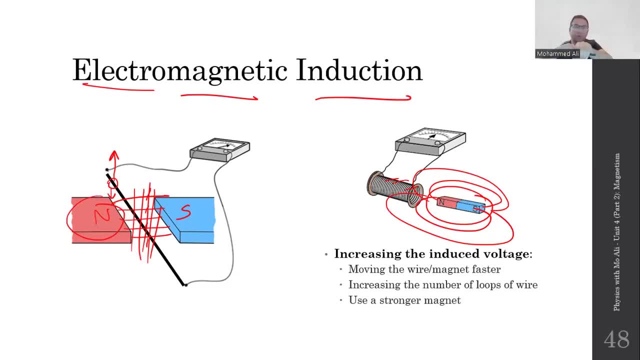 So as you move the magnet into and out of the coil or next to the coil, it doesn't matter. What matters is that this magnetic field continues to cut through the coil. This generates electricity or, we say, induces a voltage. He loves that term. 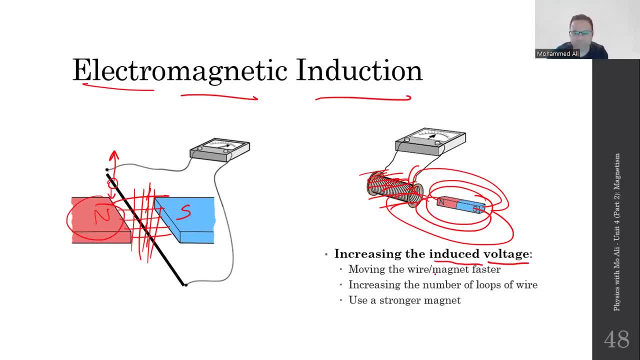 The examiner loves that term- Induces a voltage. So how does that work? again, How, I'm sorry, Do you increase the voltage you generate, You move the wire faster, or you increase the number of loops or coils, or use a stronger magnet. 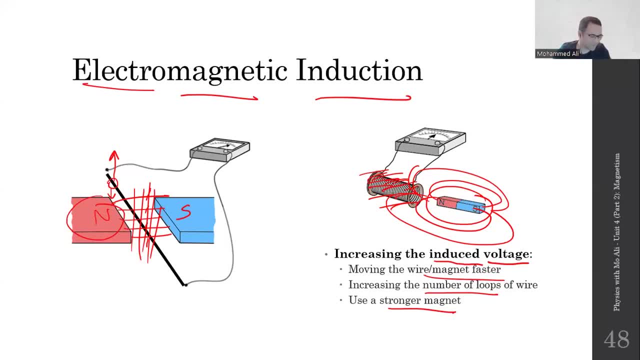 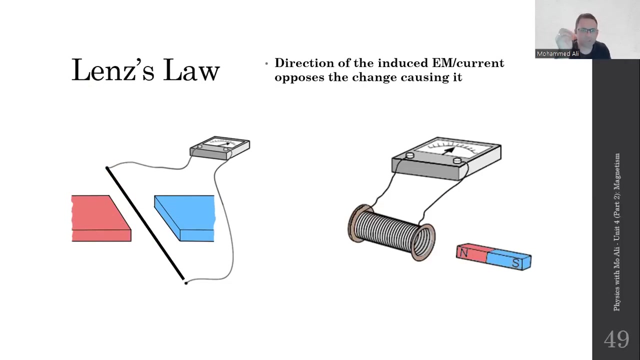 Just like the motor effect. Just like the motor effect. Then, Finally, Before we move on to the generator, this is a very extra part And, honestly, this is also extended. Keep this in mind. You don't have to remember the name of this law. 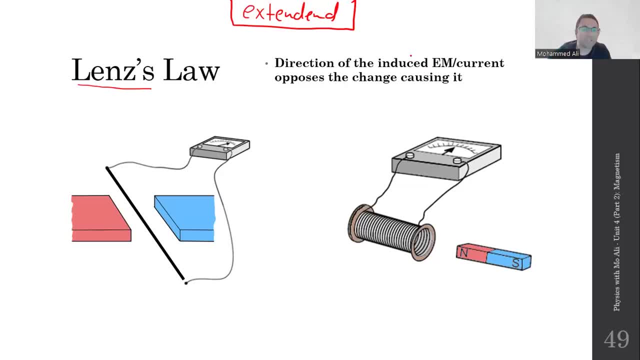 but the examiner expects you to understand the implications of this law. When you move a wire, for example, down. When you move a wire down, the magnetic field is cut through And the wire cuts through the magnetic field. We have a law called Fleming's right hand law. 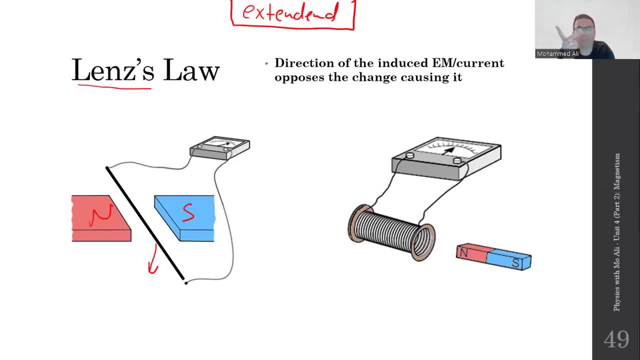 It's just like the left hand rule, but with your right hand. So you find, use it to find the current that you generate. So if you're moving the wire down, the magnetic field is from north to south. The current is moving this way. 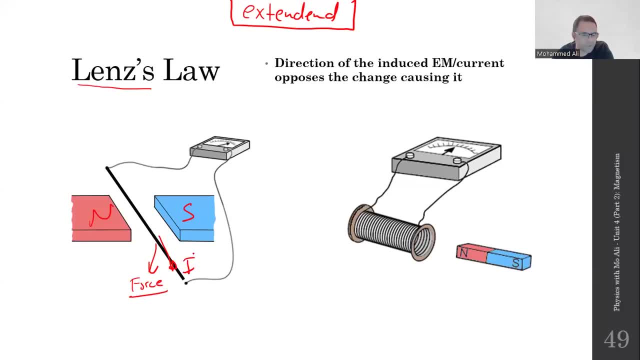 Now ignoring the law for a second, ignoring the right hand rule for a second. Why is the current generated in this direction? There is a reason for it. You want to know why? Because, for some reason, whenever you try to generate electricity by moving a wire through a magnetic field, 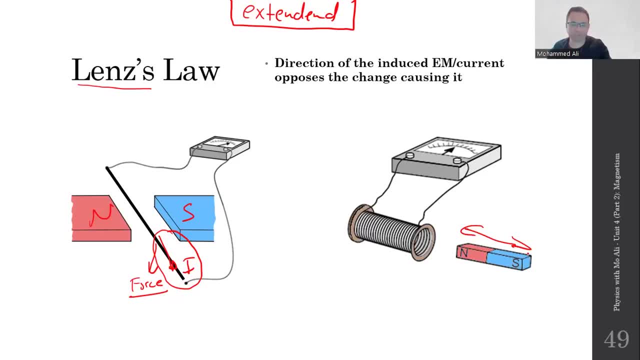 or by moving a magnet into and out of the field, into and out of a coil. I forgot to hydrate. So by moving a wire up and down through a field or by moving a magnet into and out of a coil, it generates a current in these things. 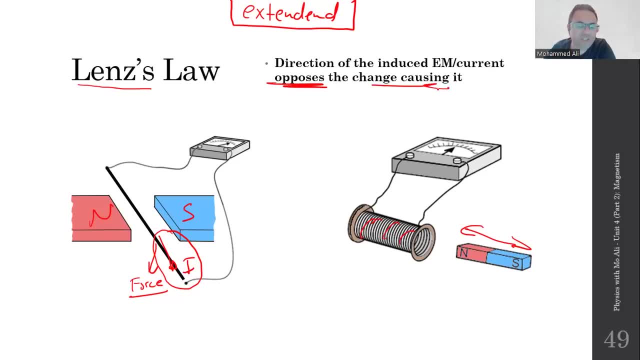 to oppose the change, causing it Meaning to oppose you, Yes, you. If you are moving the wire down, it will generate a current that will resist you so that it tries to go up. I'm not saying it is going up. All I'm saying is the current that the wire will generate. 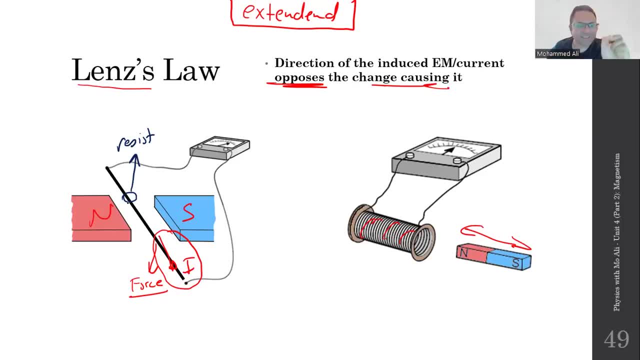 it will be generated So that it produces a magnetic field, and the magnetic field that it produces resists your motion. It's very, as we say, toxic. Hey, I want to move the wire down. No, I want to go up. 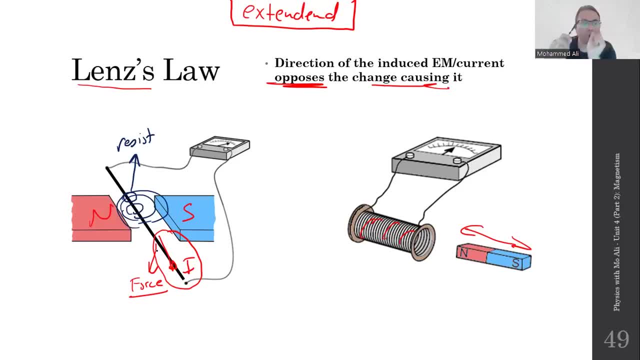 Okay, then let's go up. No, no, I want to move the wire down. It will always try to oppose you Even better here. If you're trying to move the magnet towards the coil, the current in the coil will be generated. 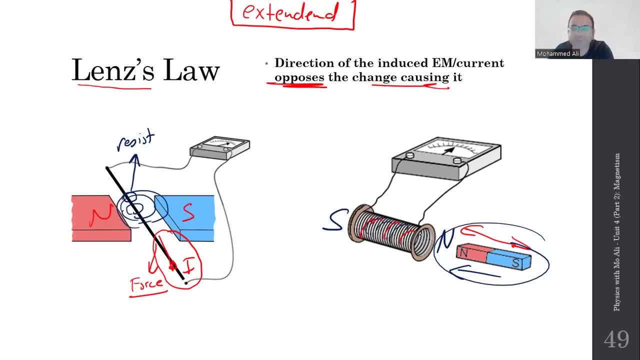 so that this side becomes north and this side becomes south because it wants to resist you. It's like, hey, I'm moving the north towards you. No, go away. I don't like you Get repelled. And if you try to move the coil away, 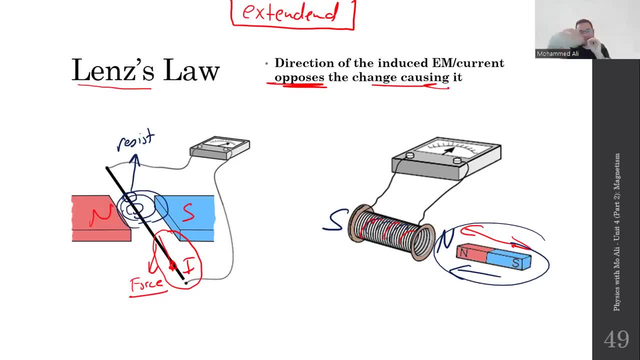 if you try to move the coil away, sort of the magnet away from the coil, what will that do? This will change it so that this becomes the south pole. This becomes the north pole. This will change it so that this becomes the south pole. 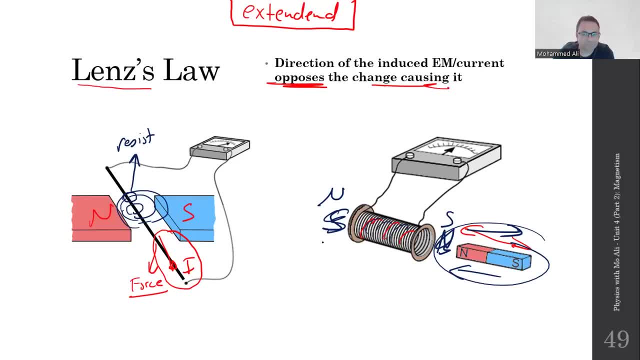 This becomes the north pole. This is called Lenz's law And it's always. it's a very minor law, to be honest, And it doesn't show up very much, but it has shown up last year in multiple choice questions. 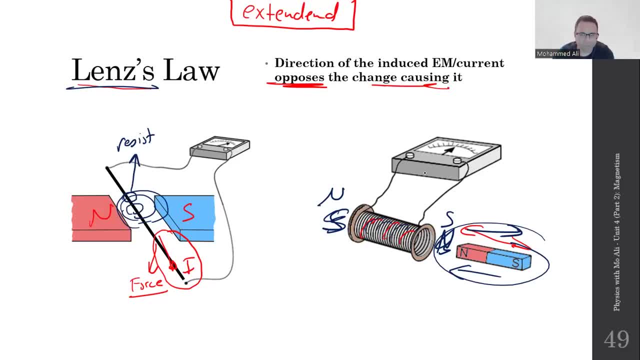 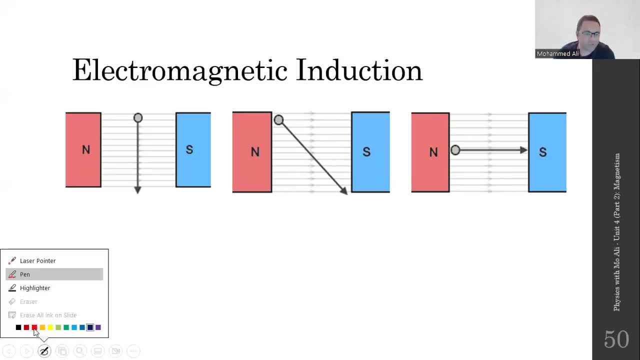 And it has shown up the year before in, I think, a paper. four question: Yeah, There's one more thing that affects the current that's generated And that's the angle at which we cut the field If you move the wire up and down. 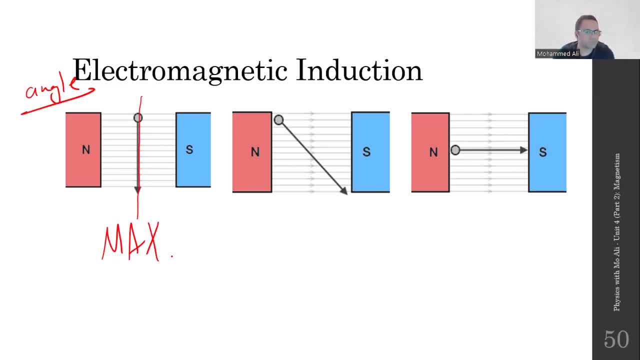 that's perpendicular to the field, you generate maximum voltage. If you move the wire at an angle, you generate something in the middle. If you move the wire horizontally, which is parallel to the field, you generate zero voltage because you're not cutting anything. 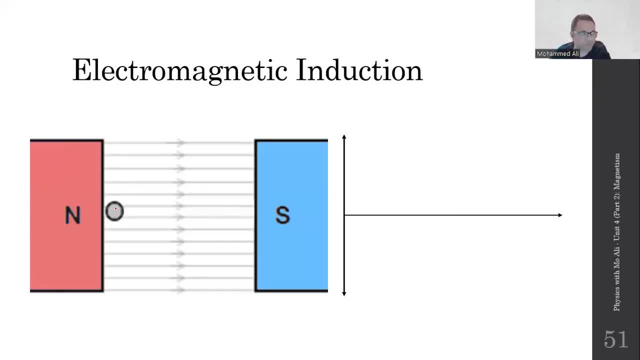 This is very important because the generator that we're going to see in a few minutes- maybe about 10 minutes, just 10,, five or 10, because the generator will be a coil moving around in a circle. When you move the coil around in a circle, 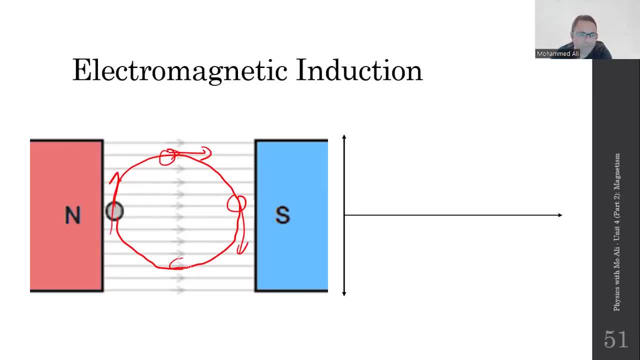 the angle at which the wire is moving is never right, constant, it's always changing. sometimes it's going up, so that's maximum voltage, then it's at an angle, and then it's horizontal, so now it's at zero, but then it's going down. now it's perpendicular again, so it gives you maximum voltage, but negative instead of positive. 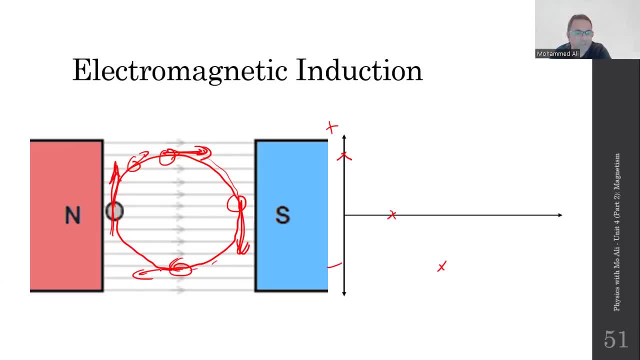 why? because the direction is the opposite and then the wire is horizontal, so it generates zero voltage, and then you're going back up again, so maximum voltage. if you draw a line joining these points, you will end up with an alternating current. so by moving a wire or a coil in a circle, 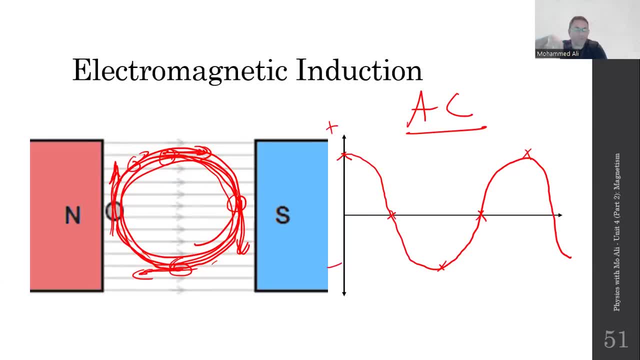 not up and down, like we were talking about a little while ago. this will generate an alternating current with changing values and directions. you, because sometimes it's going up, sometimes it's going down. this gives you maximum voltage when the coil is going to be horizontal and it gives you zero voltage when the coil is vertical, because at these moments the wires that 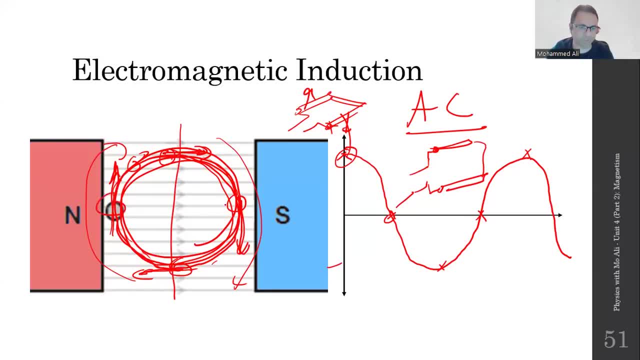 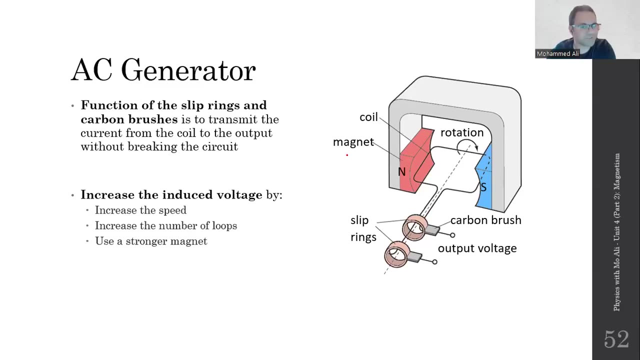 are doing the cutting are moving up and down. like we said, up and down is maximum and here it gives you zero because the wires are moving left and right, so left and right is zero and finally this gives us the generator. if you noticed? do you think i made a mistake? do you think these two look the same? of course they. 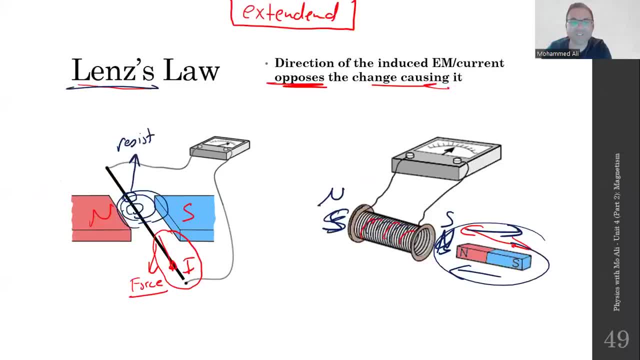 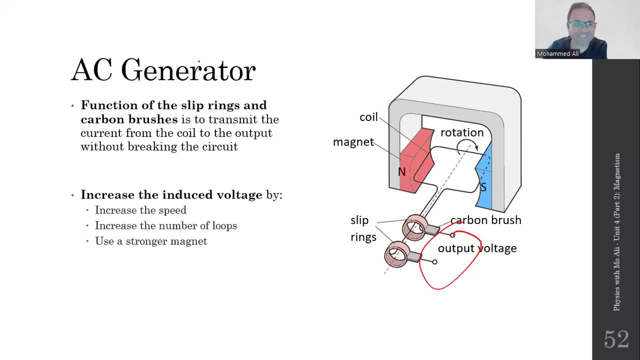 do. they're almost the same device. the difference is what? the biggest difference besides the slip rings: is there a battery or is there no battery? there's no battery. this is a generator. we're the ones who rotate the coil. we grab the coil, we rotate it. we rotate the coil, we rotate the coil. 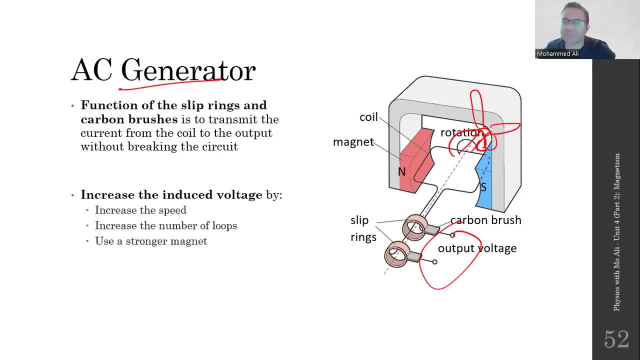 there could be a turbine here, there could be, i don't know, a hamster wheel here. all right, there could be human guinea pigs here, where we have them try to exercise. you know, you put someone on a treadmill, have them run. uh, the as they run, they're running, causes the. 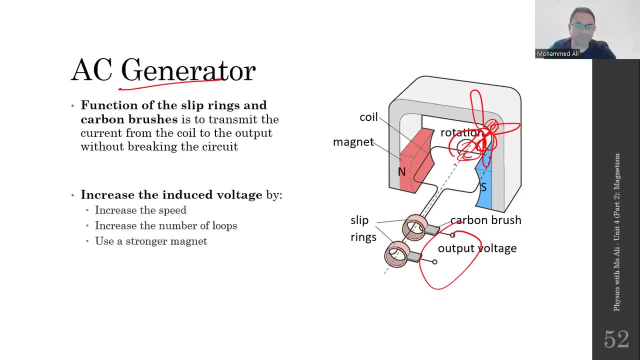 or put them on a bike. the bike causes them to spin a coil through a magnetic field that generates electricity. see, we can even make humans generate electricity. if we want to. right and they get the to lose weight, win-win. i'm not sure how effective that would be, but nonetheless so as the coil 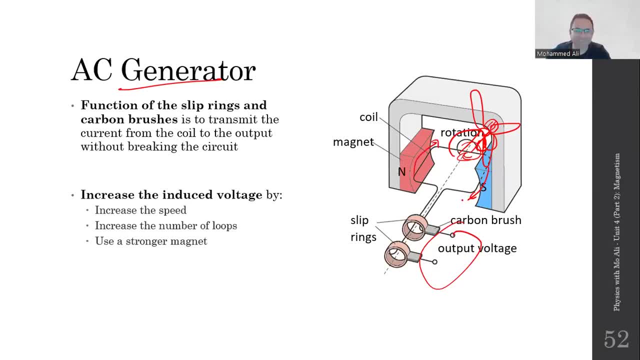 rotates, the coil cuts through the magnetic field and that generates electricity. you can increase the voltage by moving it faster, increasing the number of loops or using a stronger magnet. the function of the split rings and the carbon brushes is just one thing: to conduct electricity from the coil to the circuit outside without breaking it. 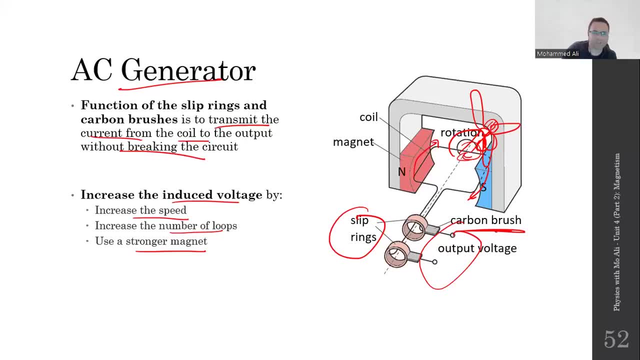 there is no need for let's reverse the direction of the current every half cycle. there's none of that. it's a very simple function: conducts electricity. there they are definitely have different uses it- uh, there's a question here. how are the two of them almost identical and have different uses? well, here's how. first, this generates electricity. we provide motion. 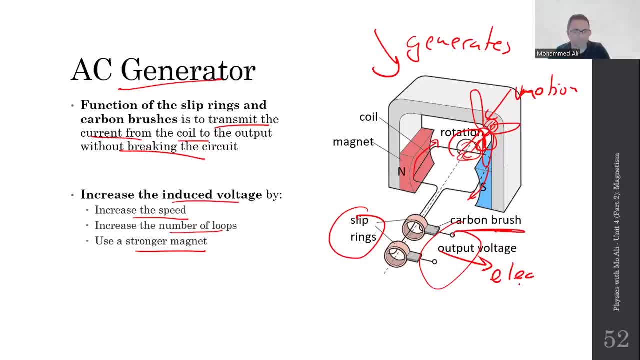 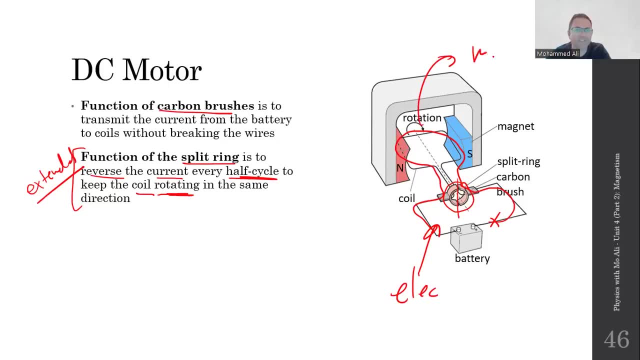 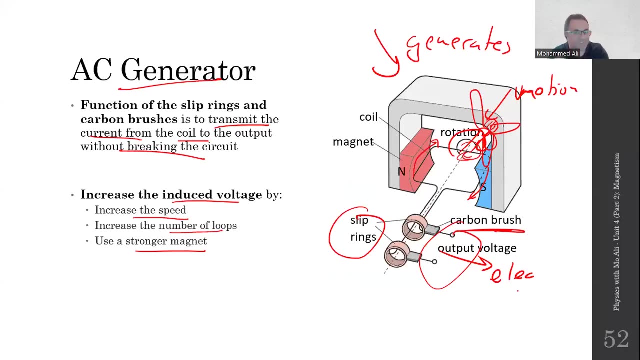 it gives us electricity. however, in a motor, we provide electricity. it gives us motion. you get the idea. it's what you decide to do. it's not what the device is, it's what you decide to do. so you give it a battery. it moves. you move it. it gives you electricity so you can charge. 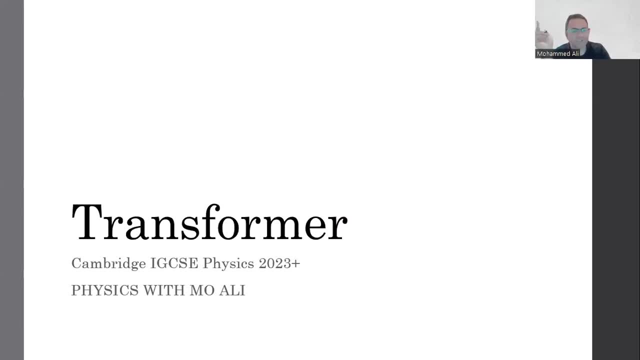 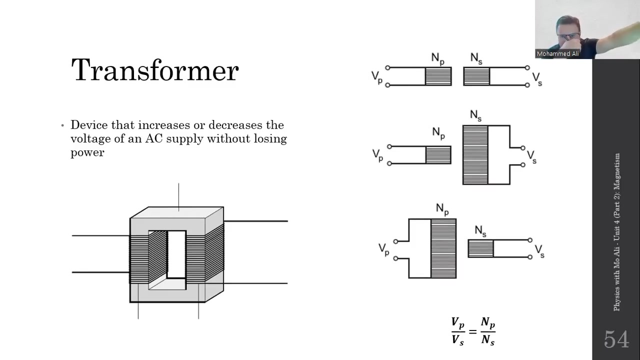 your phone or your battery or something. finally, the transform. this exists everywhere, by the way, like i was using this right now because i was charging my phone right next to me over here. i was just charging my phone, so why am i saying charging my phone? because the charger of a phone decreases the voltage from the 240 volts of my socket supply down to the 5. 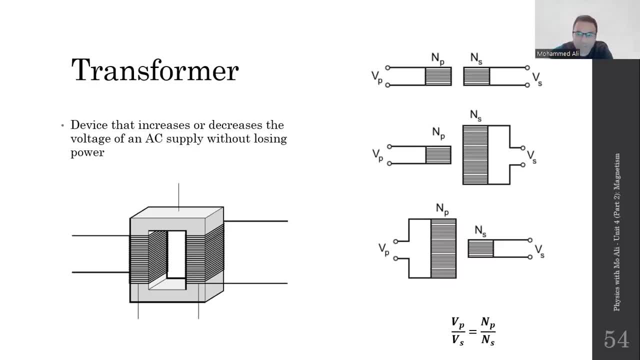 volts that my phone needs. how does that work? here's how it works. a transformer consists of three devices- i'm sorry, three components. i meant to see components- a primary coil, a secondary coil and an iron core. here's how it works. we put an ac voltage through the primary coil. the current goes through the. 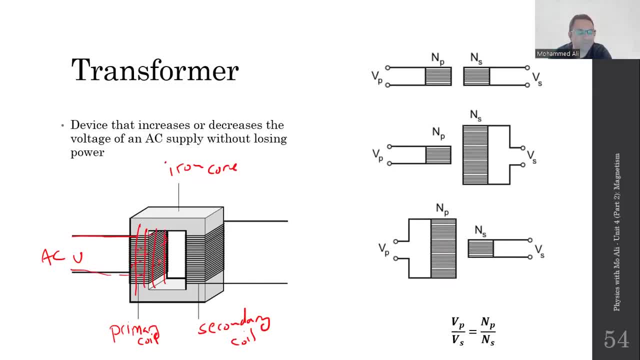 primary coil and it produces a magnetic field. you're like: cool, this is a magnetic field, then what? this magnetic field goes through the iron core and then it cuts through the secondary coil- ah, hear that term. cuts through, which means electromagnetic induction is occurring. we're generating electricity. 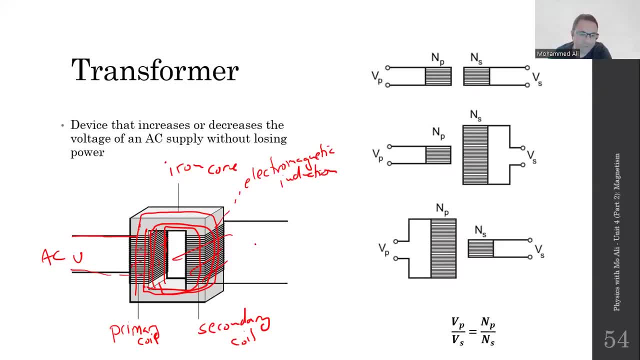 so when you generate new electricity or a new voltage here, you get an output ac voltage. now what's the point? um, bravo, mister, bravo, you changed voltage to magnetism, back to voltage. so what? the one thing that you can control here is the number of turns of the coil. 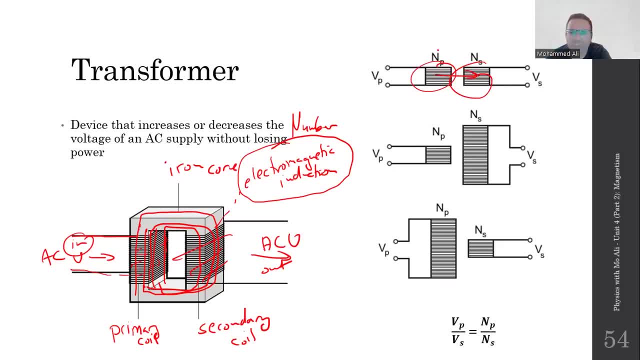 if the number of turns of both of these coils are equal, nothing happens. you give it 100 volts, it gives you 100 volts. but if the number of turns of the secondary coil is greater than the primary, the voltage will increase. give it 100 volts. give it 100 volts, it will give you 200. 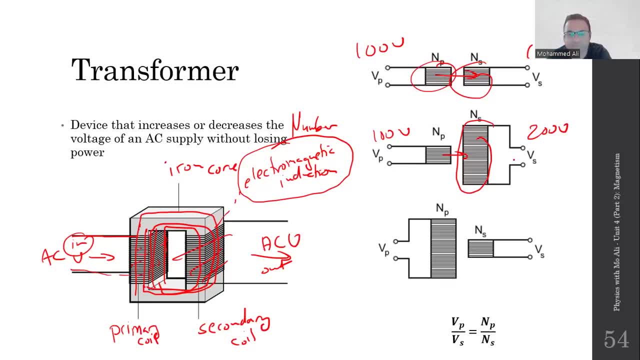 volts. if you double the number of turns, it will double the voltage. however, if the number of turns of the secondary coil is less than the primary, give it 100 volts, gives you 50 volts. what's that? based on the ratio of the number of turns. so here's the rule: vp over vs, that's primary volts. 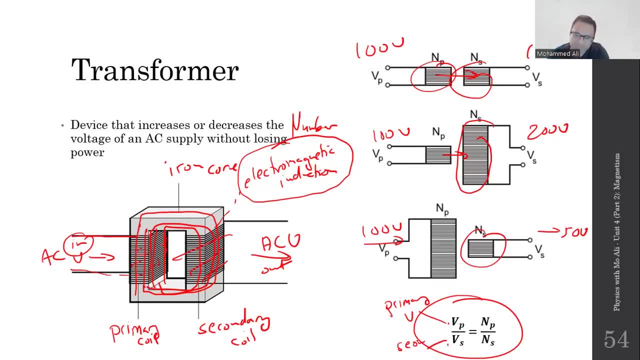 which is equal 10 volts divided by ns дет. what's the verse with tent density? so, as an example, if you calculate the voltage, think of it as 2017 per hour. here's the Victor E streets concentration in terms of time. see how i took the terms in terms of volt. 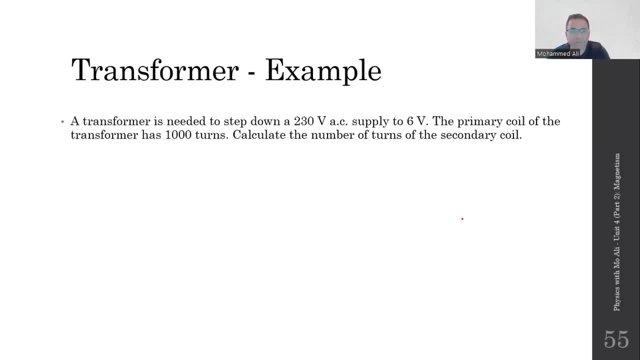 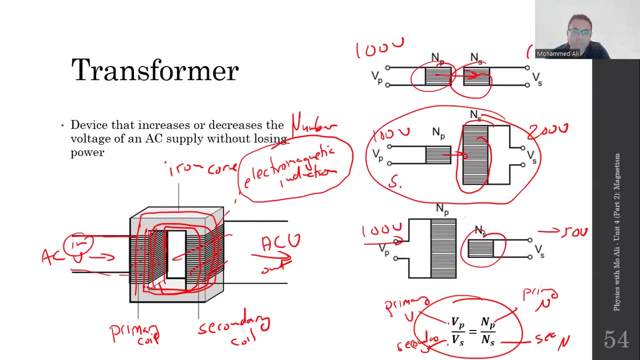 do the sum of the current of voltage. this is losing liter to current valued under Spicy charge, so it's now zero. so what is the average voltage? the Verse T. so this is the� high up voltage. indicated voltage where I start is 11. or there are Qatar Stadium medisson. 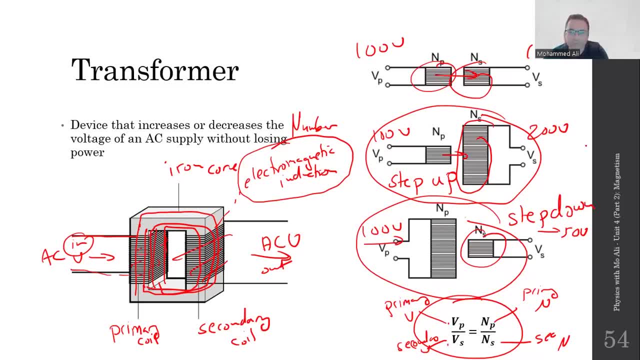 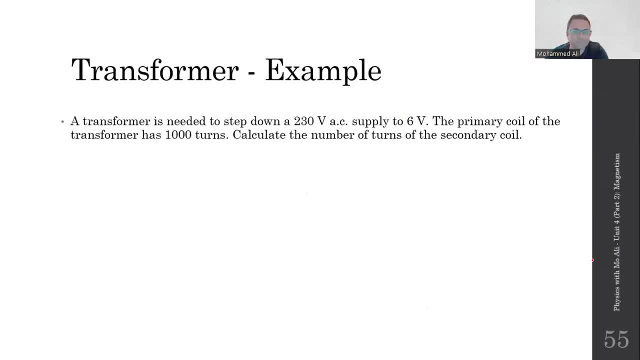 and cii times 50 point y resources for this PV1 is c4515 down transform, because this increases the voltage, the other decreases the voltage. let's solve this again. the transformer is needed to step down, so the voltage is decreasing 230 volts to six. so that's your primary voltage. here's your secondary voltage. the primary coil has a. 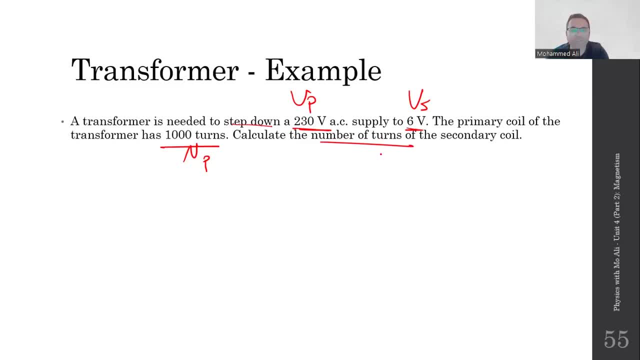 thousand turns. he's given me the number of turns of the primary. what's the number of turns of the secondary? come on, here's the rule: np over ns equals vp over vs. okay, i have the np, that's a thousand. i don't know. the ns vp is 230 over six. by the way, you're literally cross multiplying. 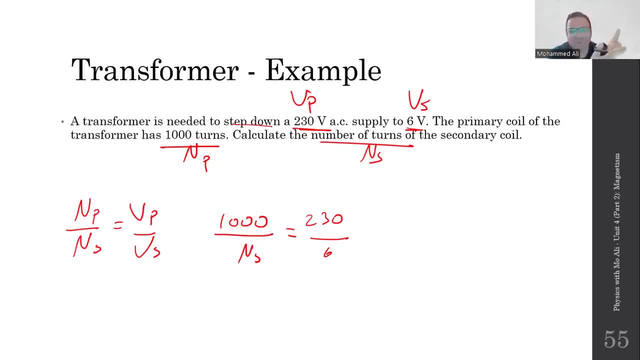 you don't have to use the ratio either. you can just cross, multiply the number of turns with its appropriate voltage and you get your answer right away. so ns is actually equal to times six over two 30. this was just math. i rearranged the formula. this goes up, this goes down, this goes up, so 1000. 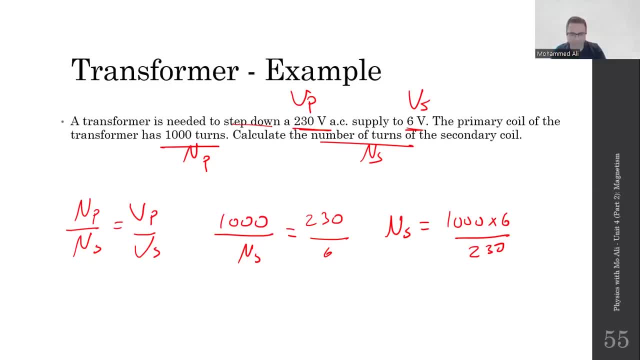 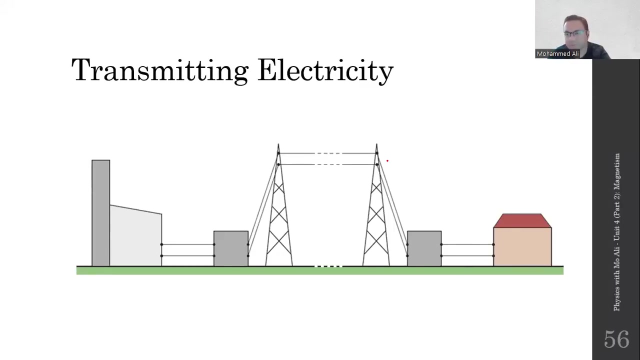 times 6 over 230. this gives me 26.1 turns. all right, so 26 turns makes sense. it's a step down transformer, so the number of turns is supposed to decrease, not increase. okay, finally, why do we even step up? this is going to be very important. that's the last thing we mentioned. 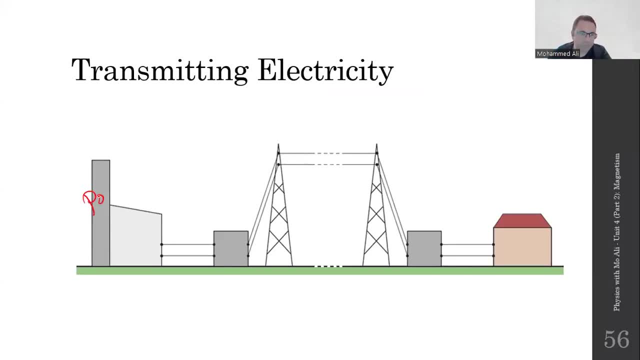 a power station, for example, generates, let's say, 10 000 volts of voltage at, let's say, one ampere. the problem with 10 000 volts in one ampere is that the transmission cables, the cables that transmit electricity from the power station to our house. 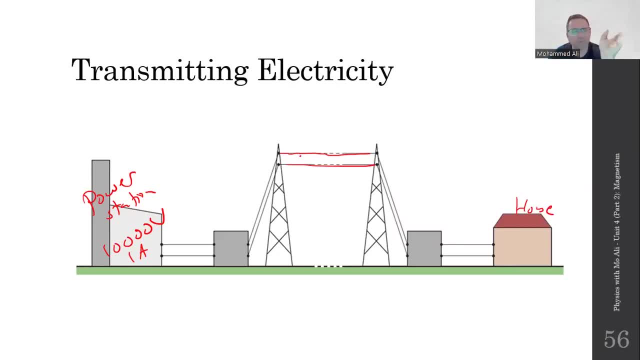 are very long, several hundreds of kilometers long, which means their current- sorry, their- resistance is very high. this will cause the wires themselves to take some of that electrical energy and waste it as heat. the wires are going to get hotter. the only way to reduce this heat is to use the power station to generate electricity from the power station to our house. 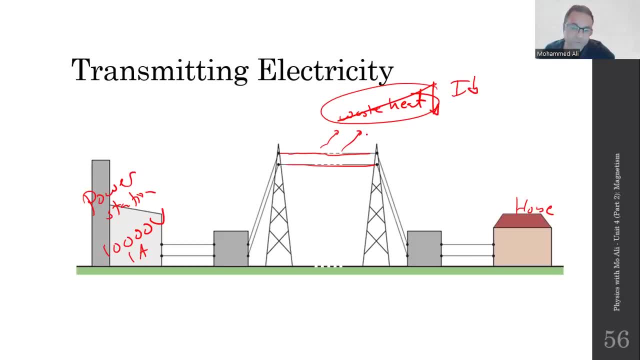 is to reduce the current because you want to reduce the power loss. honestly, you can reduce the resistance too, but they're already very long. you can't make them any shorter, so you can decrease the current. how we put a step up transformer here: when you step up the voltage, let's say from 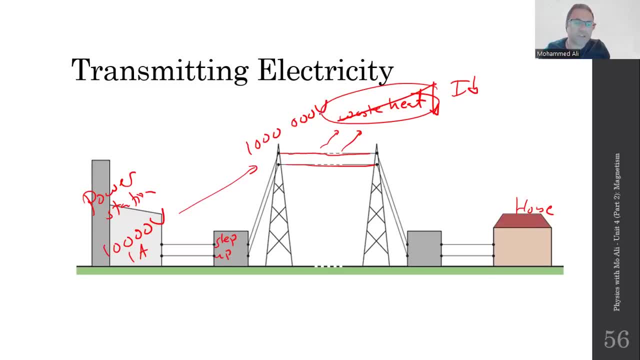 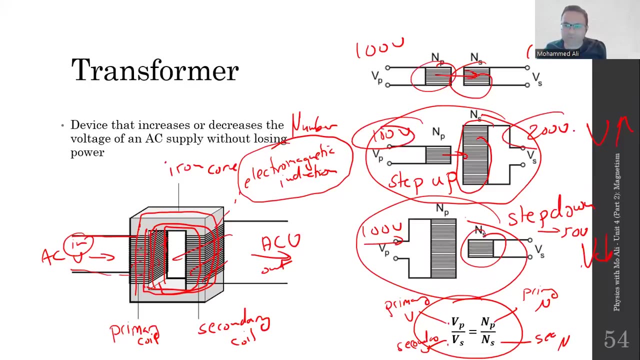 10 000 volts to 1 million volts. the current decreases. because that was a question you should have asked me a while ago, which was: what, mister? how do we step up? where do we? how do i get an extra 100 volts, mister? he said there's 100 volts, it's now 200 volts. how did the voltage increase? 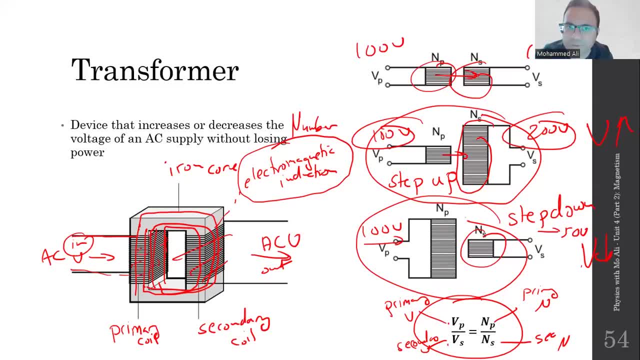 the voltage does not increase out of nothing. energy cannot be created or destroyed. it's only changed from one form to another. when we increase the voltage, something else has to decrease in its place. that's current. when we decrease the voltage, something else has to increase in its place. that's the current. 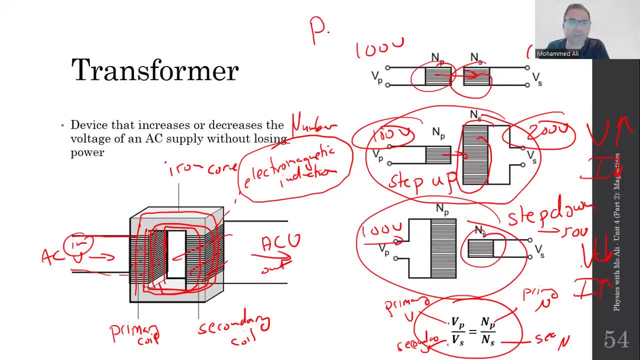 because the way transformers work is that the power, that's input to the transformer, should be equal to the power output from the transformer. so the v times- i remember that's, we studied this a little while ago- input equals v times i output, so when we of course there should not be a number. 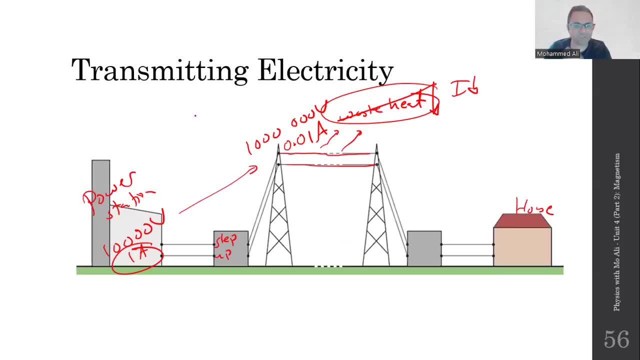 of. uh, that's some places here. that's why i said that's the current, that's the voltage, that's the current. i said 26 in the end, but you can leave it as is. when we step up, the current decreases. so what's the advantage here? when you increase the voltage, the advantage here is that number one, the 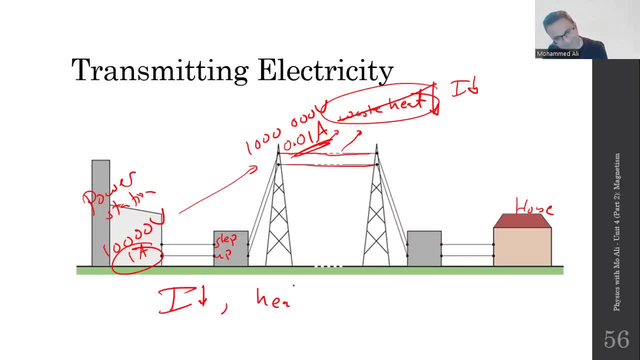 current decreases. so number two: the heat produced by the cables decreases, so there is less energy lost or wasted. obviously we can't have a million volts reaching our homes, so before our homes we have step down transformers which drop it to our usual 240 volts, whatever ampere it. 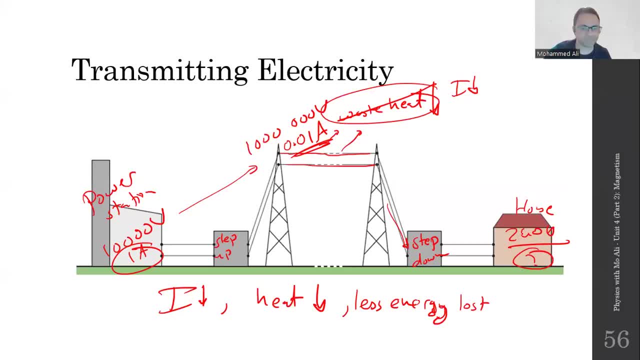 is we need here, and that's it. so what are the advantages of high voltage transmission of electricity? it decreases the current, which decreases the heat produced by these cables. so less energy is lost from these cables and we save money. in the end we can use thinner cables. we we 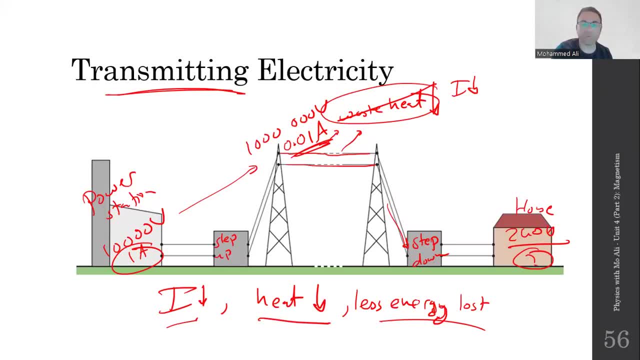 don't waste money, so i don't lose energy and money here. what's the relationship between i and v? only in a transformer are they inversely proportioned. only in a transformer are they inversely proportional, because in a regular circuit, if you increase the voltage, the current increases. if you decrease the voltage, the current 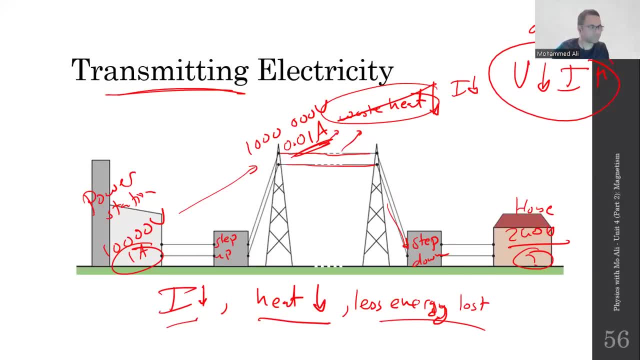 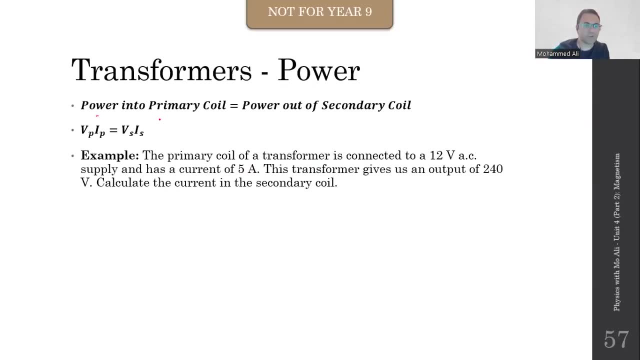 decreases. was that clear, excellent? so last example: power in equals power out, as we said. so the primary coil of the transformer is 12 volts, the current is 5 ampere. the transformer gives us an output of 240 volts. calculate the current in the secondary coil, so literally use this rule. so this is what. let me mark these this. 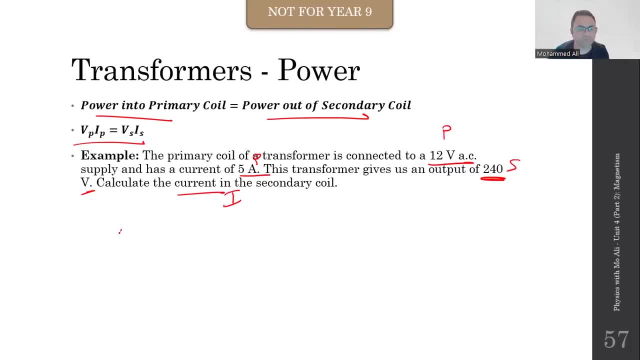 is primary, this is primary, this is secondary. i want the current. so vi primary equals vi secondary. so that's 12 times 5 equals 240 times- i don't know. so i don't know- equals 12 times 5 over 240. i'm expecting the current to decrease because the voltage is increased. 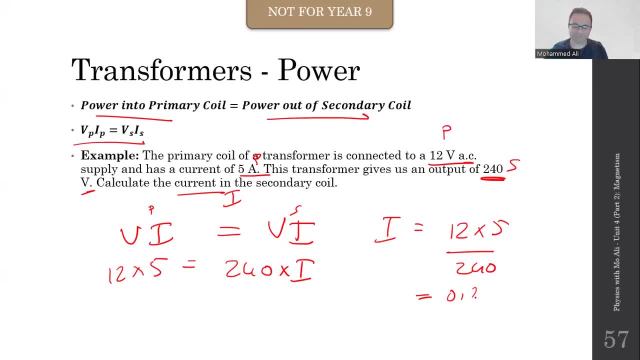 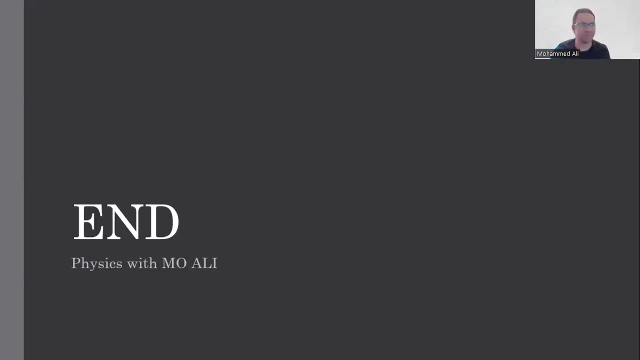 and we would be right. it's 0.25 ampere down from 5, and that's correct. ladies and gentlemen, thank you very much for your time and i'll see you guys next time. peace.